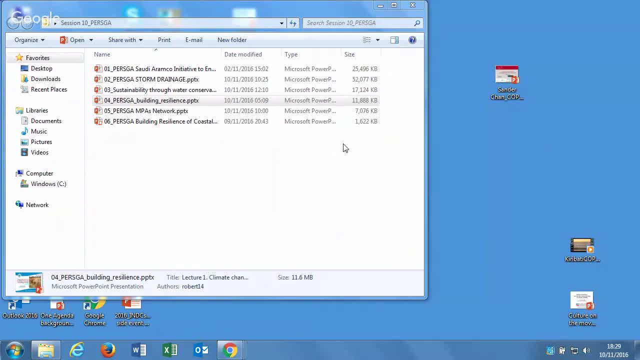 has a PhD in biological oceanography from Texas A&M University. He's a senior consultant with Saudi Aramco Environmental Protection Department. He's a board member of Saudi Wildlife Authority. He's a past chairman and current member of the Environmental Technology Management Association. 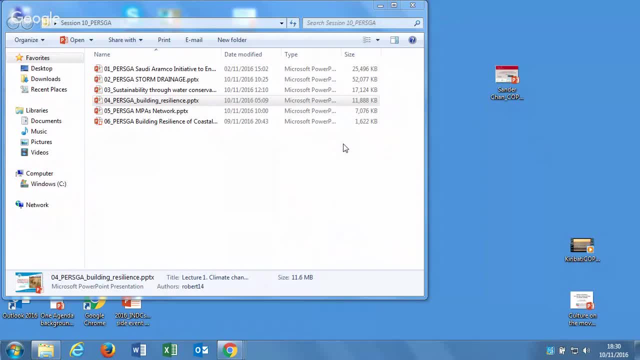 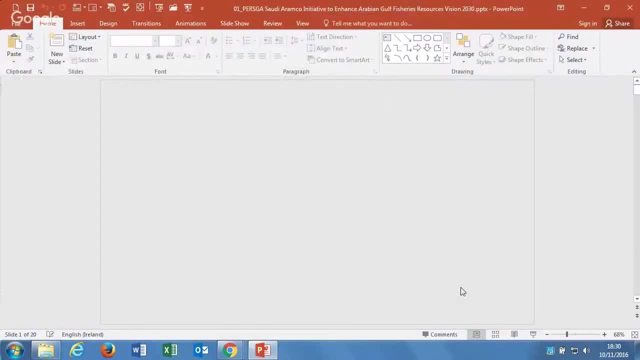 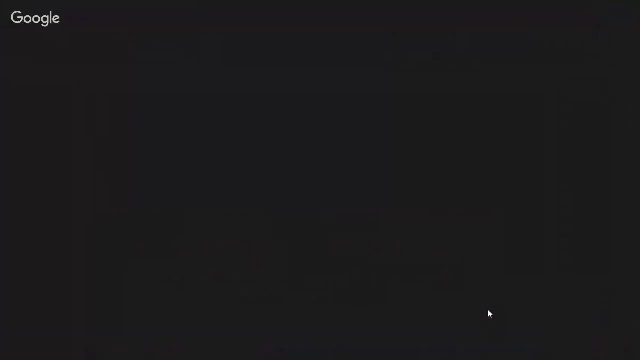 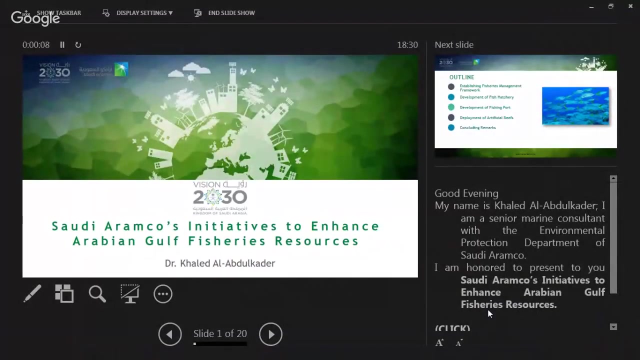 and he's the vice chairman for the Saudi Aramco Environmental Committee Standard. Thank you, Good evening. I hope we'll be able to keep you awake at the time of this day. I will start my presentation today with the outline of the presentation. 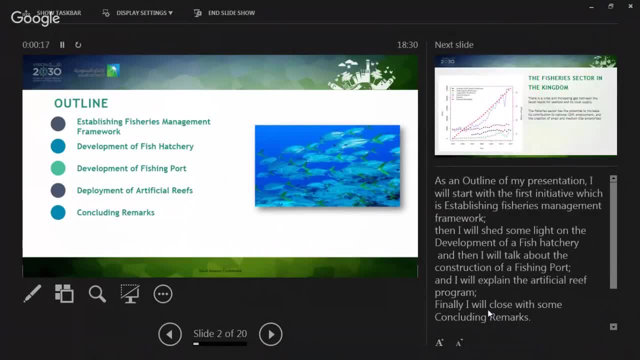 I will start with the first initiative, that is, the establishment of fisheries management framework. Then I will shed some light on the development of fish hatchery in the Red Angles And then developing the fishing port and deployment of artificial reef in the areas. 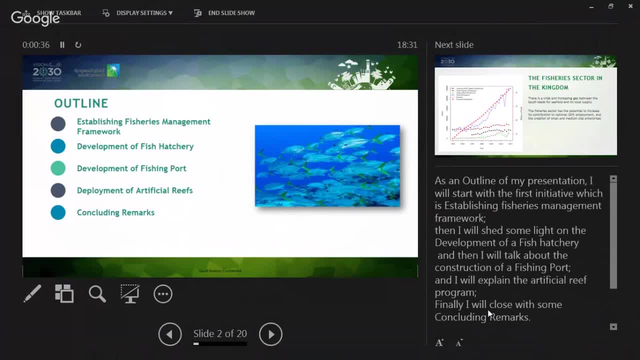 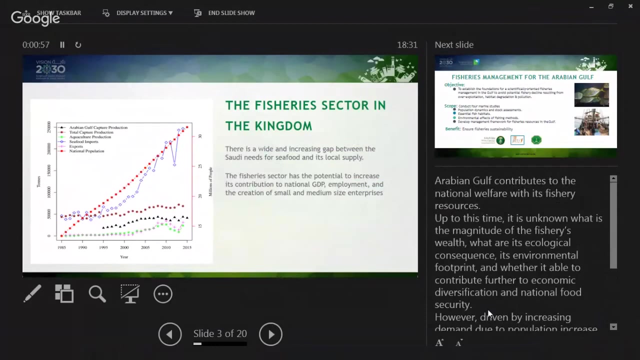 of the eastern part of the Gulf. And then I will conclude with some remarks. The Arabian Gulf contribute to the national welfare with its fisheries resources. Up to this time, it is unknown the magnitude of the fisheries resources. what are the ecological consequences, its environmental 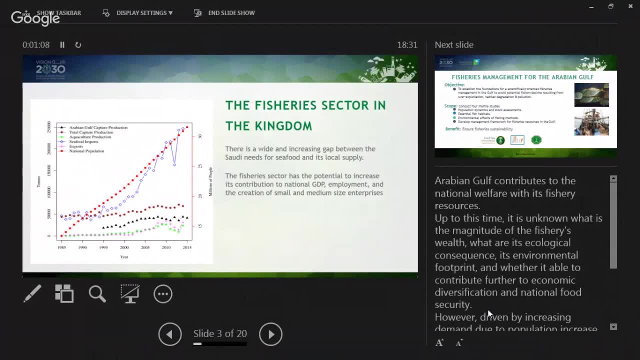 footprint and whether it's able to contribute further to the economic diversification and the national food security. However, driven by increasing demand and population, increase total volume of the national and currently less than half of the seafood import to the Gulf, making the kingdom dependent on the other countries for fisheries resources. 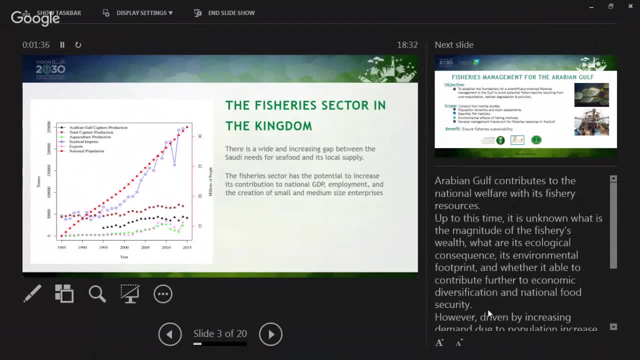 And if you look at this graph, you will find the increase of the demand of the fisheries going up with the population increase, while still the production and the harvesting of the Gulf is still at the same level. So the in collaboration with the Ministry of Environment, Water and Agriculture, we're 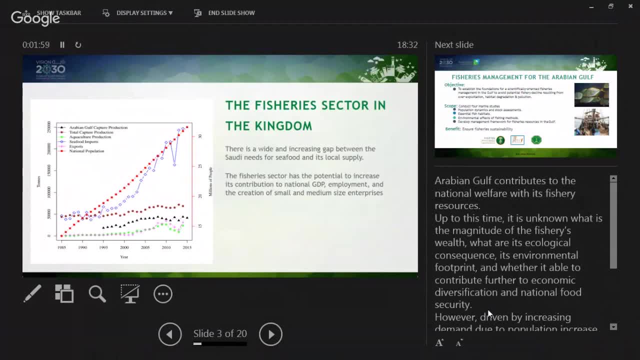 able to do this. I realize the need to establish a foundation for scientifically oriented fisheries management in the Arabian Gulf to increase the utilization of the available fisheries resources, at the same time avoiding any potential fisheries decline resulting from over-exploitation or habitat degradation. 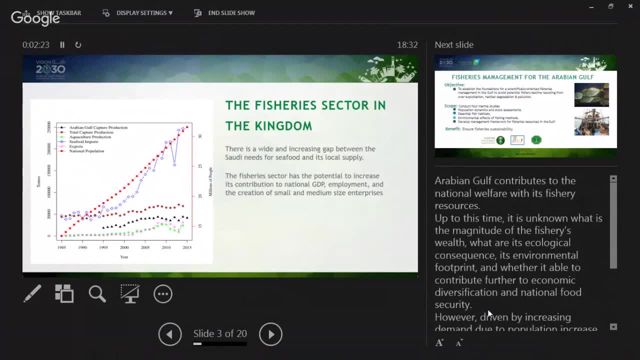 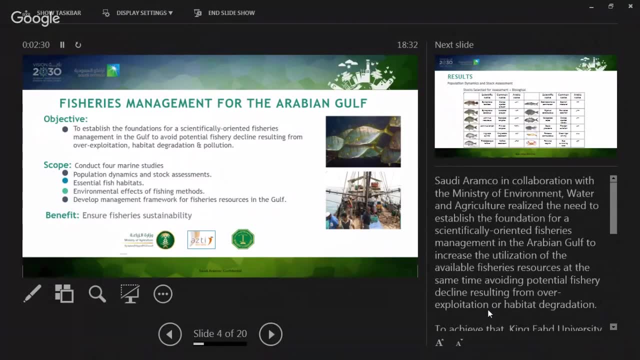 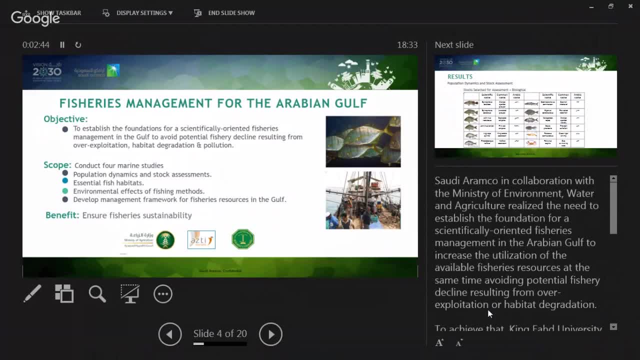 the population dynamics and stop assessment of major commercial stocks of the Gulf, and also to indicate essential fish habitats and quantify the environmental footprints of fishing method- the current fishing method in the Gulf. All of these results will be utilized to develop a management framework for sustainable fisheries. 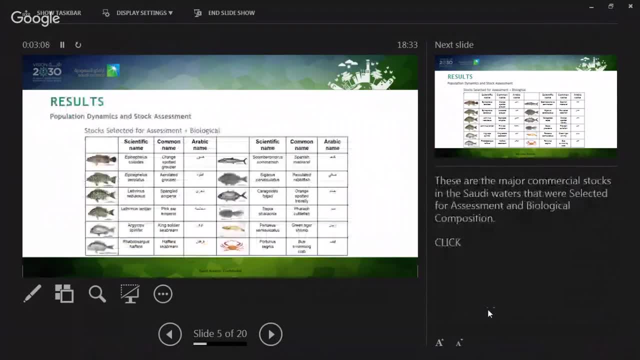 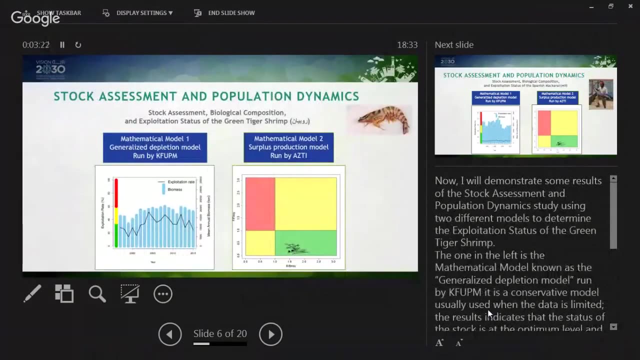 management in the Gulf. These are the major commercial stocks in the Saudi water that were selected for the assessment and biological composition. Now I will demonstrate some of the results of the stock assessment and population dynamics of study, using the different models to determine the exploitation status of the green tiger. 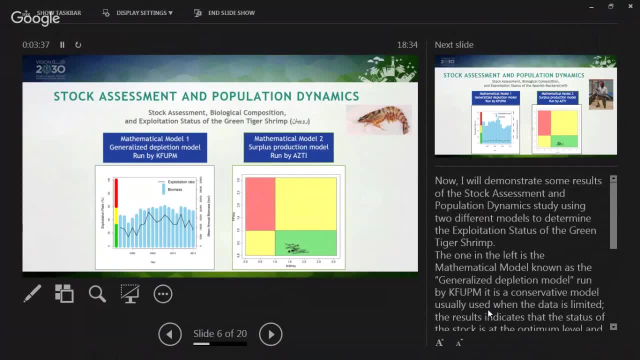 shrimp: The one on the left, the one on the left. sorry, it is a mathematical model known as the generalized depletion model. run by the KFUBM is a conservative model Usually used when the data is limited, where the results indicate the stock in the optimum. 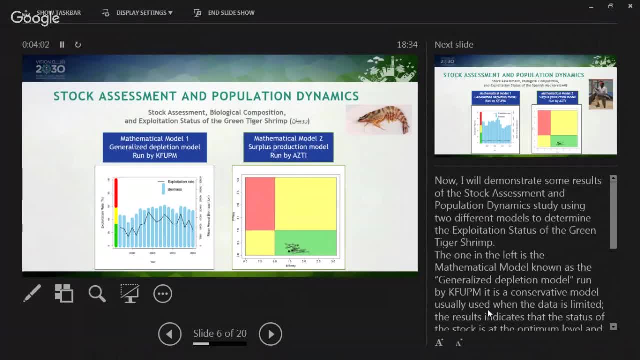 condition and is stable and does not recommend any increase. However, in the graph at the right, the mathematical model surplus production model used and run by ASTEE and usually used in Europe. where data is available, a long series of data is evident. 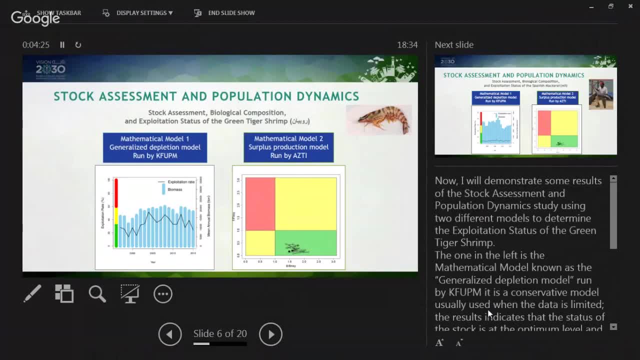 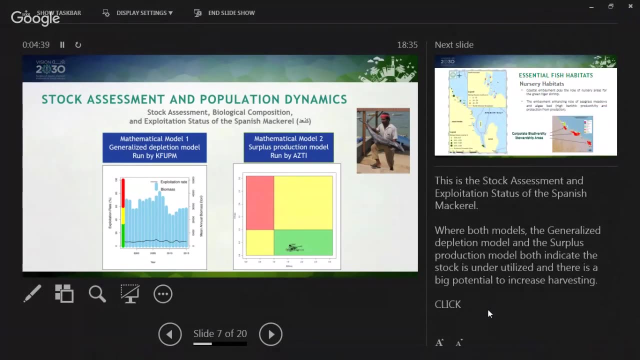 The results of the model indicate there is a high potential to increase the shrimp harvest from the Saudi water. This is the stock assessment on exploitation status of Spanish mackerel, where both model- the generalized depletion model and surplus production model- both indicate the stock. 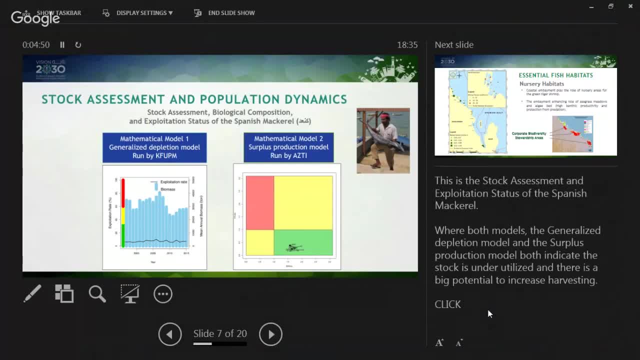 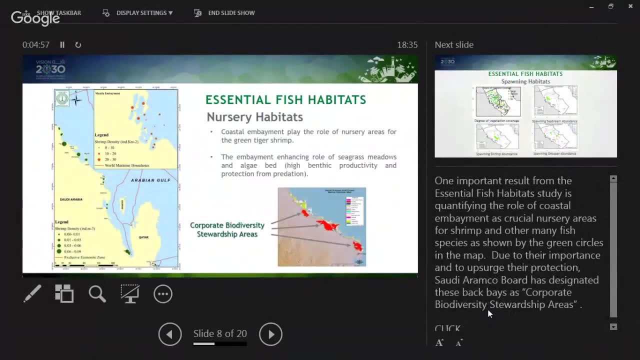 is underutilized and there is a big potential to increase harvesting. One of the important results for the essential fish habitat study is quantifying the role of coastal embayment as a crucial nursery area of shrimp and other many fish species, as known by the green circle in the map, where these are very important. 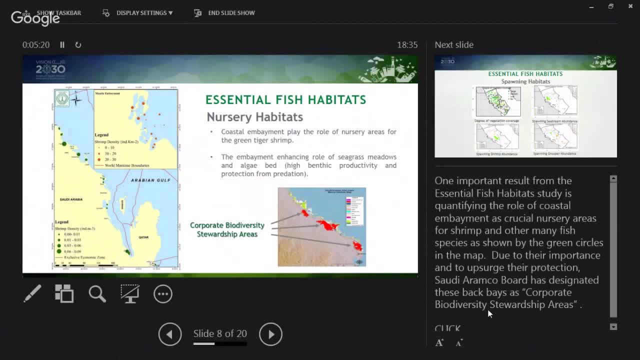 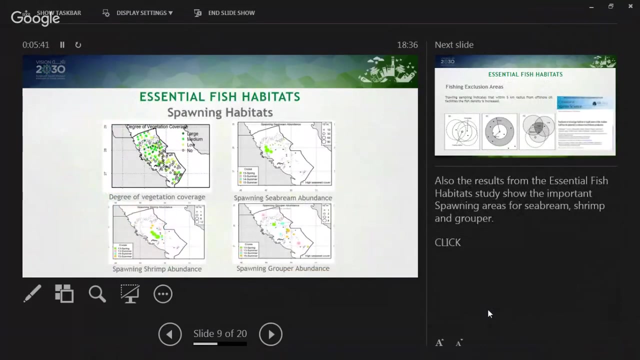 for the circulation and protection of the juveniles. Saudi Aramco Board has designated all of these embayments as corporate biodiversity stewardship areas. These are also results from the essential fish habitat study shows the importance bounding areas of sea bream, shrimp and grobbers. 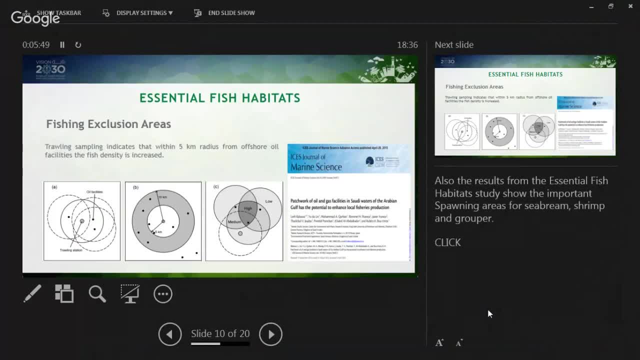 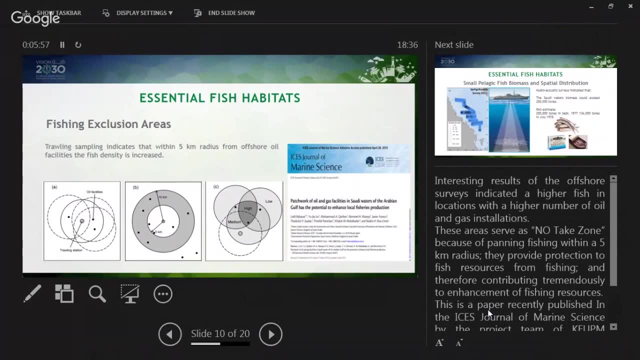 Interesting results of the offshore surveys indicated a higher fish location with a higher number of oil and gas installation. These areas serve as no-take zones because of banning fishing within a five kilometer radius. They provide protection to fish resources from fishing. They provide protection to fish resources from fishing. 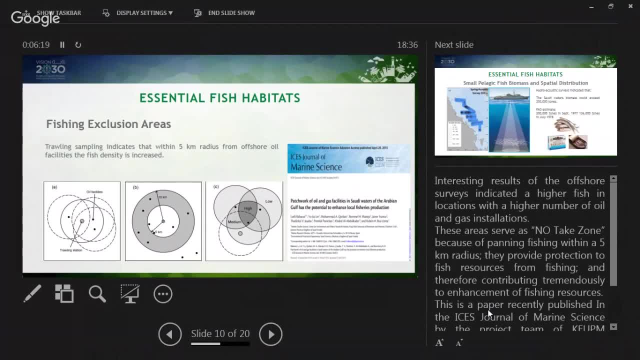 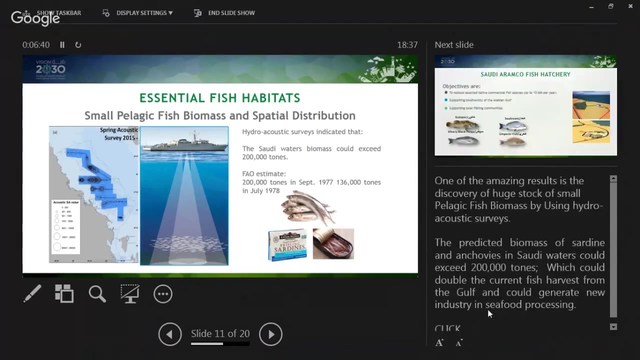 And therefore contributing themselves to enhancement of fishing resources. And here and your right, there is a paper and I SE journal of marine science just published by the team indicating and documenting these as scientific findings. One of the amazing result of the discovery of huge stock of a small phylogenetic fish. 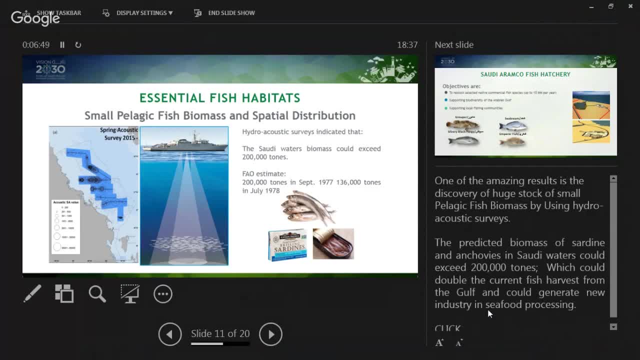 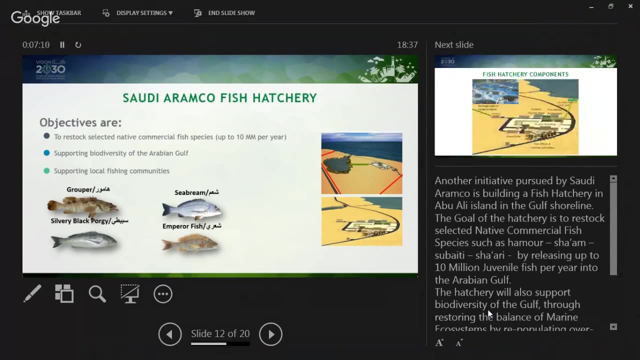 biomass by using hydroacoustic surveys. This predicted biomass of sardines and anchovies in Saudi water could exceed 200,000 tons, which could double the current fish harvesting from the Gulf and could generate a new industry in seafood processing. Another initiative pursued by the company is building a fish hatchery in Abu Ali area. 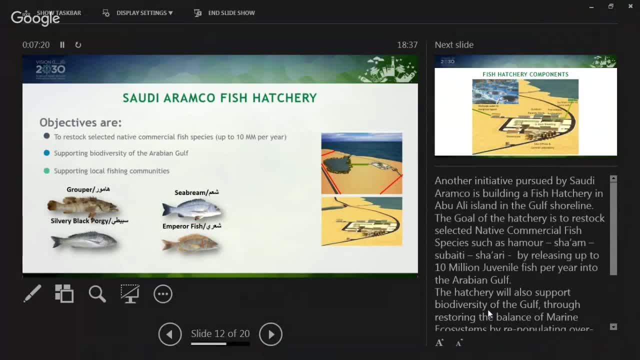 The goal of the hatchery is to restock selective native commercial fish such as hamur, shams, bayti and shari, which is the most popular commercial fish in the Gulf, by releasing up to 10 million juvenile fish per year into the Arabian Gulf water. The hatchery will also support biodiversity of the Gulf Through restocking the imbalance of marine ecosystem by repopulating over-exploitated fish species. and the hatchery also will enhance local fishing community by enhancing the available fisheries resources. These are the fish main components, which are the outdoor parent stock, indoor breeding. 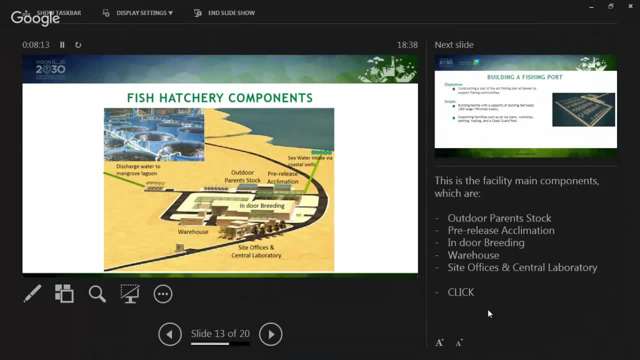 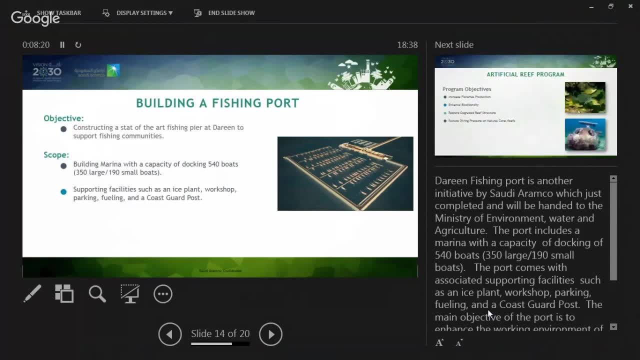 and breeding. In addition, the hatchery's engine, for more than 1.5 million maximum, is built in an Indian fish farm. So with the required capacity, the hatchery of the Hatchery should be able to make a significant 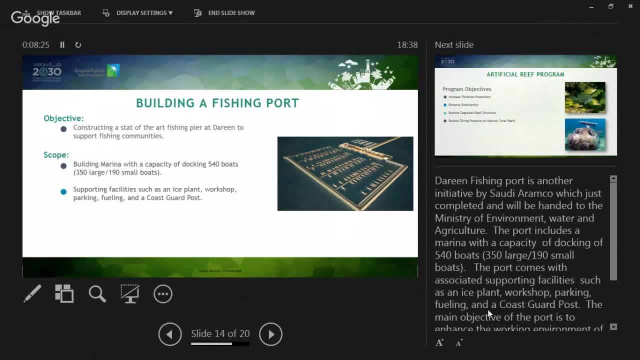 difference in the world's marine fishermen. The O2O2O2O2O2O2 is the company's most famous fishing interpretive technology. It is the first fish farmers to produce these products. The Hatchery Limited Inc. which has the most money in the world, is the company's largest. 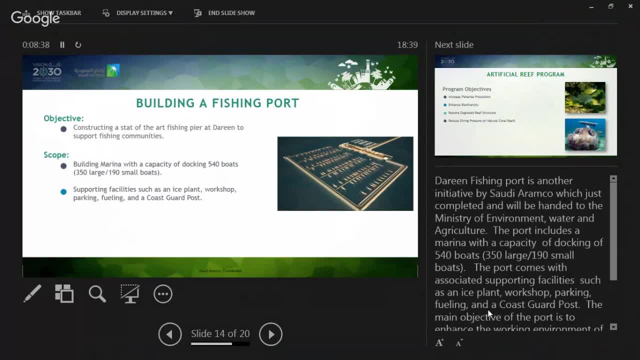 successors and has around 2.2 million fish. In addition, it is the country's largest exporter of морay fish and all the world's largest supporting facilities needed for the fishermen community and the main objective is really to enhance the working environment of fishing community. and, as a result, will encourage also young Saudis to involve in this sector. the fourth initiatives by Saudi Aramco, which is the creating artificial reefs in the Saudi water. the objectives of this initiative: increase fisheries production, enhance biodiversity, restore degraded natural reef and reduce diving pressure on natural coral reef in the Gulf. to conduct this initiative, we have 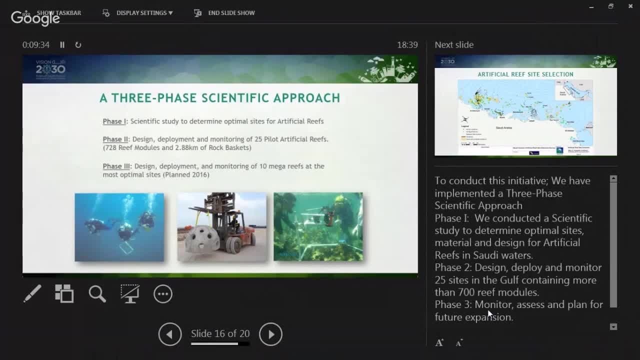 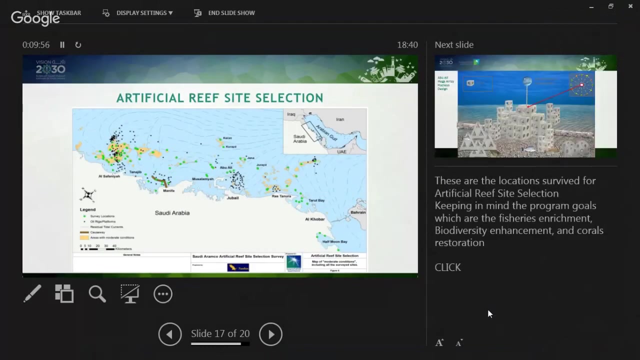 implemented three-phase scientific approach. first phase: we conducted isolation scientific study to determine an optimal site. second, design: deploy and monitor 25 sites in the Gulf with more seven seven hundred reef modules. three, third phase: to monitor and assess and plan to future expansion. these are the locations surveyed for artificial reef sites: selection keeping in mind the 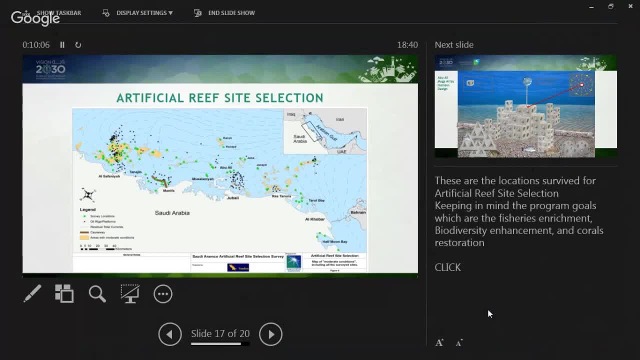 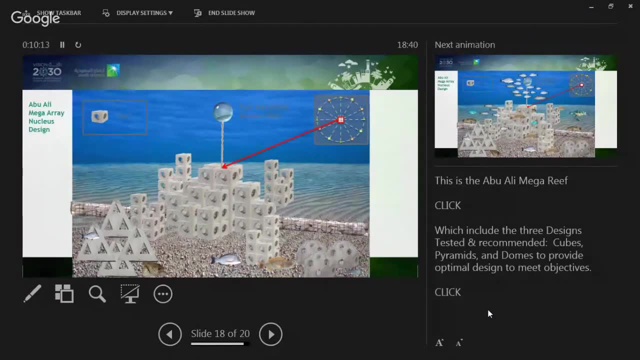 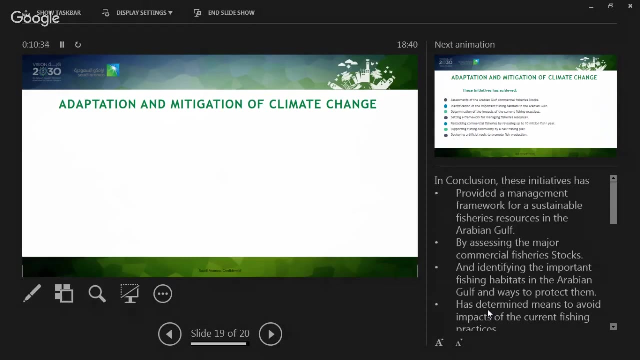 program goal for fisheries enhancement, biodiversity enhancement and coral restoration. this is the mega, mega reef in Abu Ali area, which include the three design, tested and recommended cubes, permit and domes to provide optimal design and to meet objectives for different sizes and species of fish fisheries in the in the area. in conclusion, these initiatives have provided a 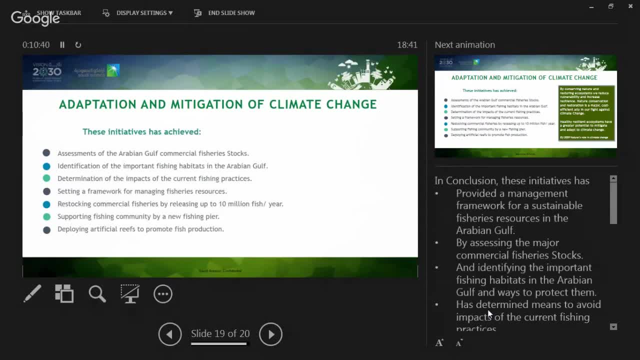 successful mall management framework for sustainable fisheries resources of the Gulf by assessing the major commercial fish stocks and had identified the importance fishing habitat, ways to and ways to protect them, and also determine the means to avoid impact for current fishing habitats and increase the stock of native fishery by releasing up to million buy to 10 million fish per year. 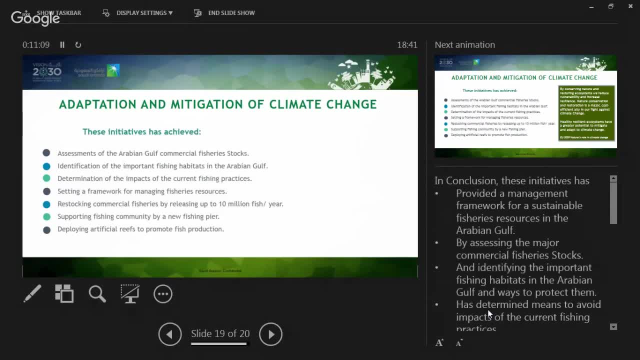 and enhancing the working environmental fishing community life and ten million fish per year. and enhancing the working environment of fishing communities and increasing the strategic走 partis environment of fishing community by providing the fishing board also will promote fish production and biological diversity by deploying artificial reef. 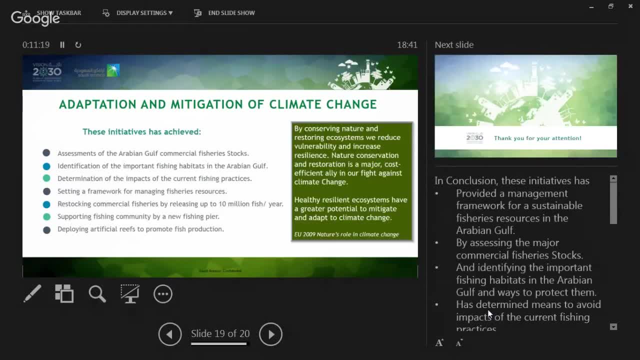 in different areas. and just I would like to conclude with a quote from EU nature role in climate change, which says: by conserving nature and restoring ecosystem, we reduce impact and increase resilience. nature conservation and restoration is a major cost-effective LA and our fight against climate change. 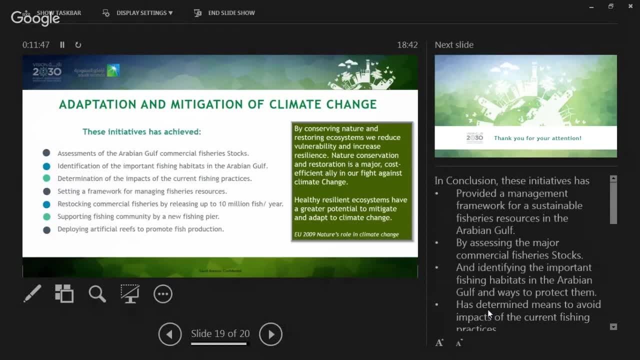 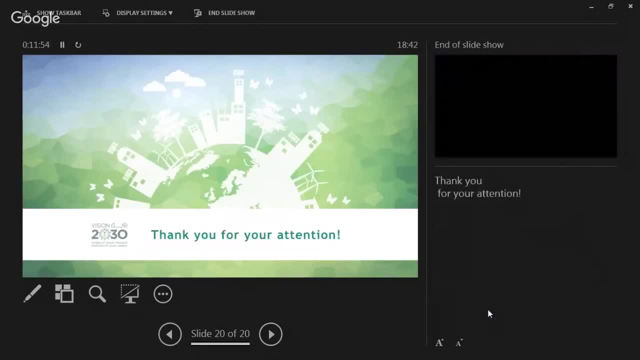 healthy, resilient ecosystem have a greater potential to mitigate and adapt to climate change. thank you for your attention. thank you very much, dr holland. ladies and gentlemen, I would like to ask you to hold the question until the end of our session, where we'll have all the speaker on the podium and later on we'll have all the 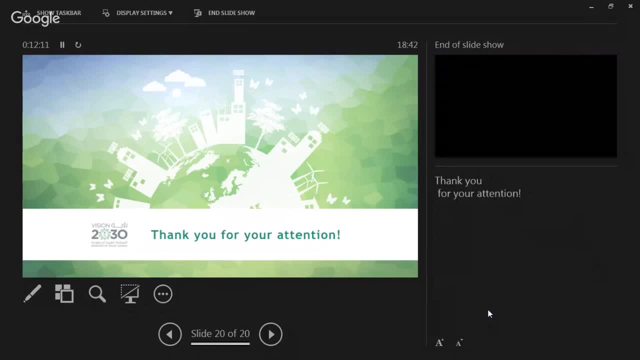 question. I would like to call for our second ski second speakers, miss engineer facial Israel, to go to the podium. engineer facial Israel is a project manager for stormwater strategy network, designer of groundwater lowering control program. he's also a member of the infrastructure coordination committee and he's also a member of the groundwater committee, and I would like 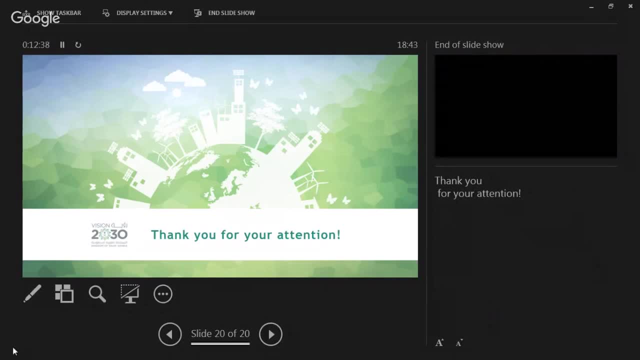 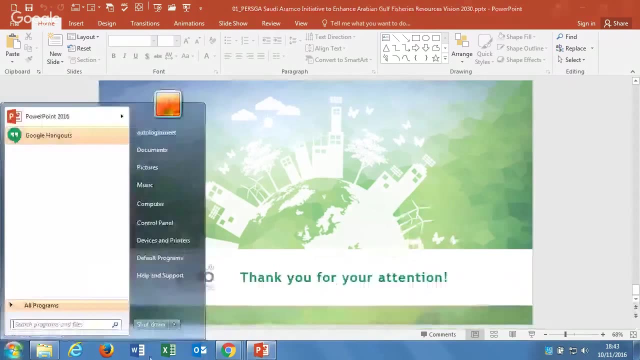 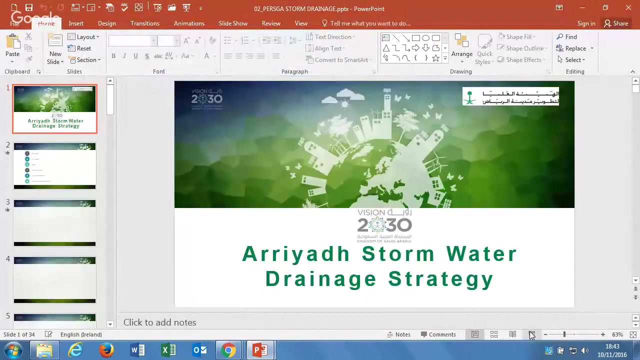 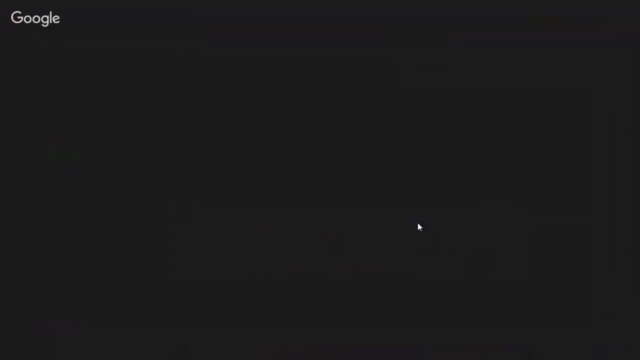 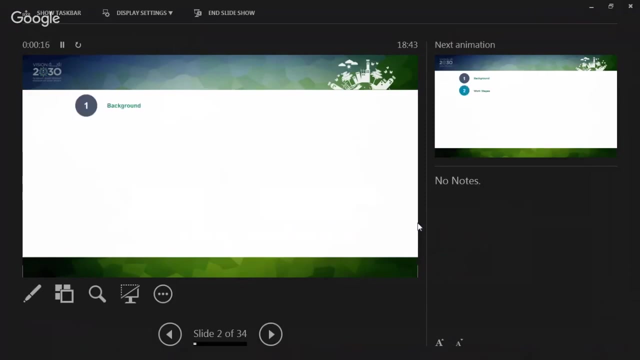 him to go ahead to the presentation. it's a pleasure to present for you the area of stormwater training strategy, the background about react, which is the capital of the kingdom of the United. then we will go through the workstates and the main issues we have faced also. 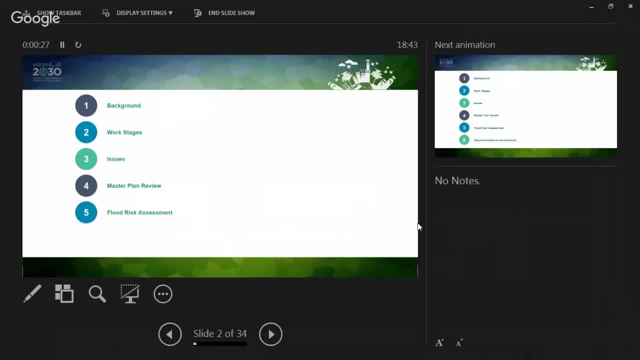 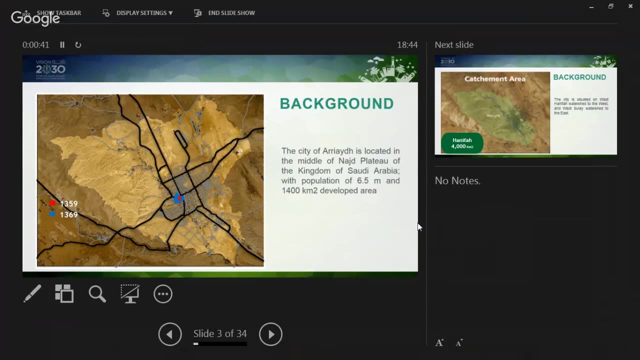 we will present the master plan review. out of that we come up with the flood risk assessment and finally, we will go through the recommendations and the decision. the city of Riyadh is located in the middle of next plateau, which is in the middle of the kingdom, with the population of 6.5 millions and with 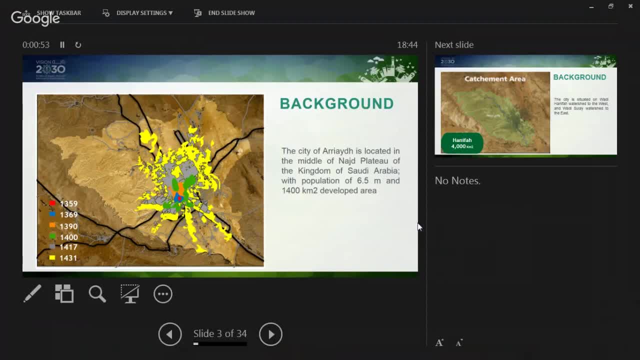 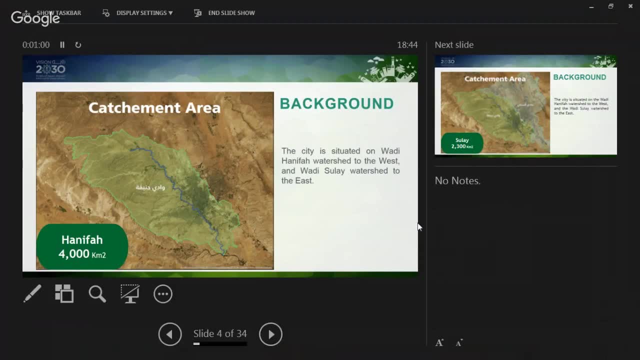 organized or developed area: 1400 square meters. also, the city is situated within two catchment. the large catchment is wadi hanifa catchment, 4,000 kilometers square, and the second catchment, to the east, is wadi as-sulay. these are the boundaries we 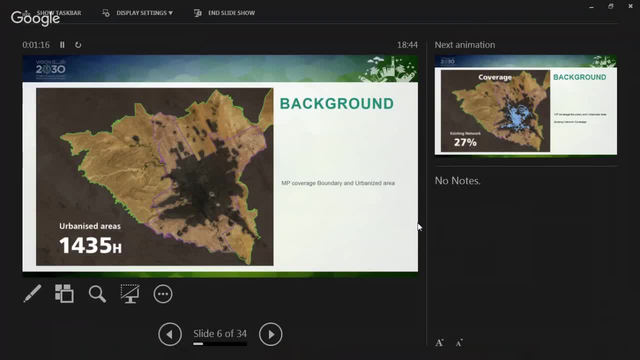 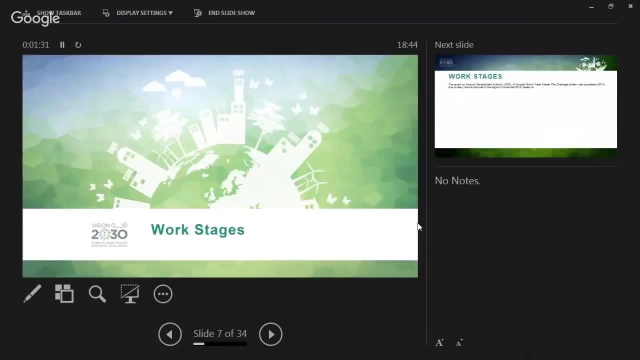 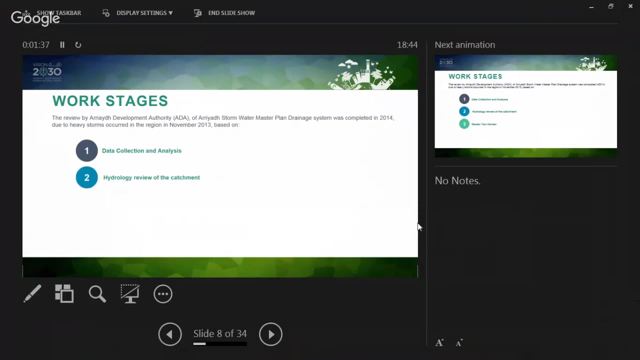 have, which we have done the master plan on, and that was in 1435 hijri, where at that time we have only 27 percentage of the existing network for the drainage system. in the work stage we have went through the data collection and analysis. hydrology helped roll, the review of the catchment and the master plan. if you and 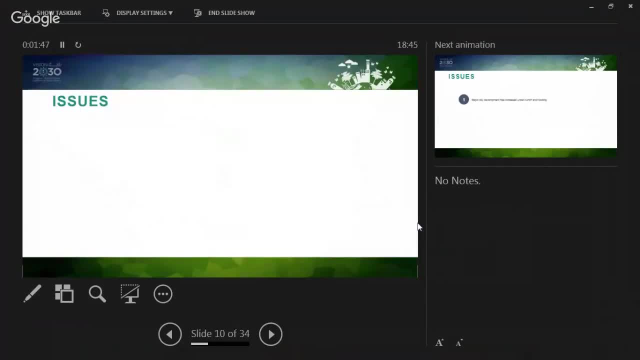 the flood risk assessment. the first main issue was that the rabbit development of the city has increased the urban runoff. also, the master plan principle was to drain all or the water, all of the rainfall out of the urban areas, without taking in consideration any green solutions at that time. however, the design standards 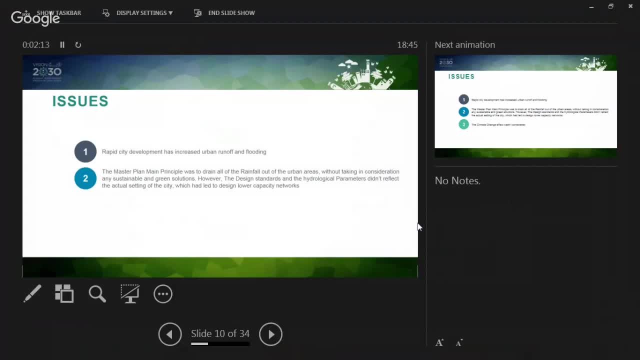 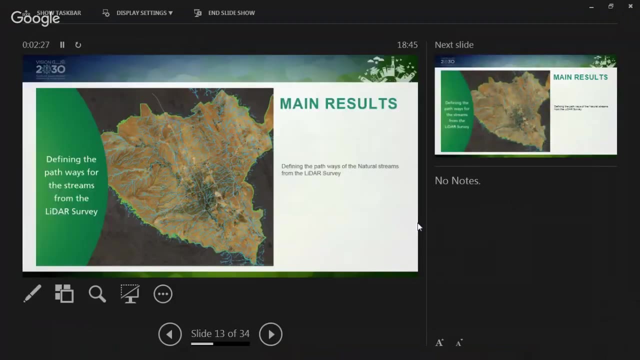 and hydrological parameters did not reflect the actual setting of the city, which had led to design a lower network capacity. also, we did not consider the climate change effects in that time. so the master plan main results was that we have defined the mainstream paths for the way for the waterways and that come 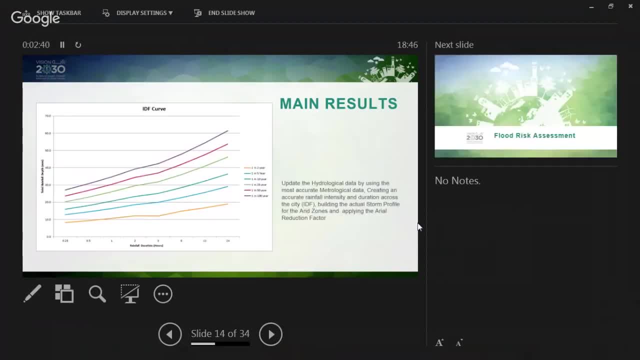 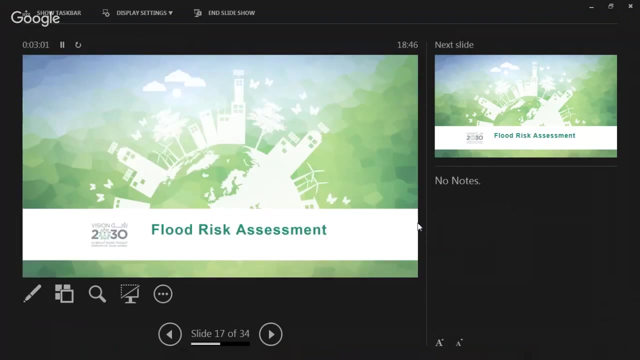 out from the later survey. also, we have updated the hydrological data by using most accurate meteorological data, creating an accurate rainfall intensity and duration actors across the city, building the actual storm profile for the arid zones and applying area reduction factor if needed. from the flood risk assessment, we have simulated the existing network with its. 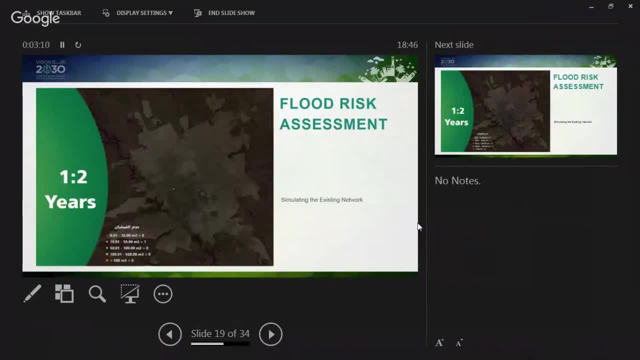 capacity and with the different retain periods. so you will see the bubbles increasing with the different retain periods, as 1 in 10 and 1 in 25, up to the 1 in 100. these bubbles will not stay in the same location, so it will move. 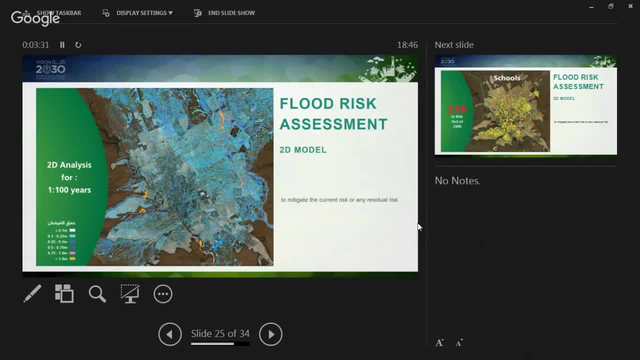 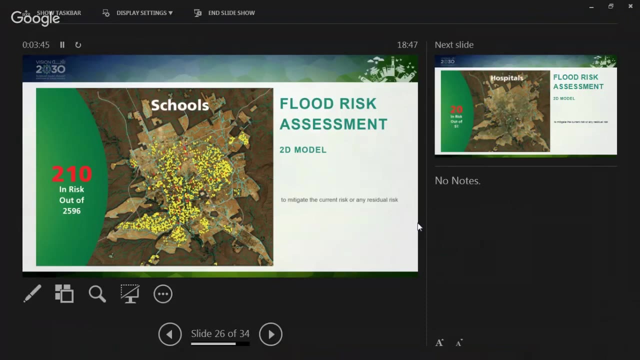 through the pathways which is reflected in the 2d model we have created to mitigate the current risk or any residual residual risk. so we came out with 210 schools are in the risk in the worst case. and we came out also with 20 hospitals, 86 enter passes. 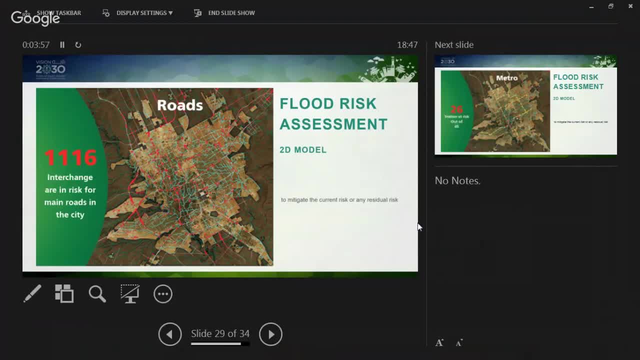 and for the roads and intersections of the roads, we have came up up to 1, 1,100 and more where the stream paths intersect with the main roads and since we have the mega project, we have also assisted that project. to know which metro stations are in the risk, we came out with 26 location are in the risk and 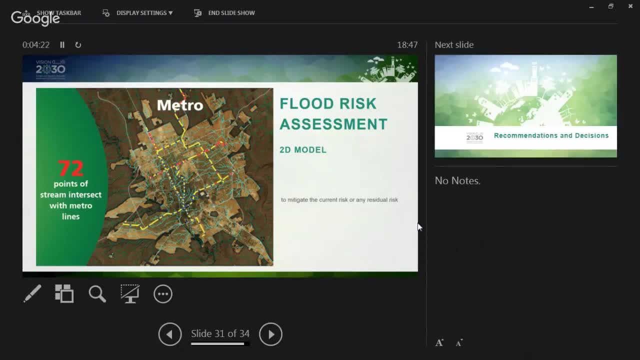 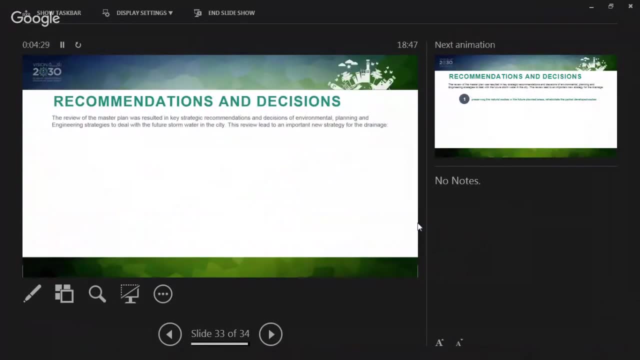 for the metro line itself, there is 72 points. so the main recommendations, the review of the master plan will be available in the next few days. and the review of the master plan will be available in the next few days, and the was resulted in key strategic recommendations and decisions of. 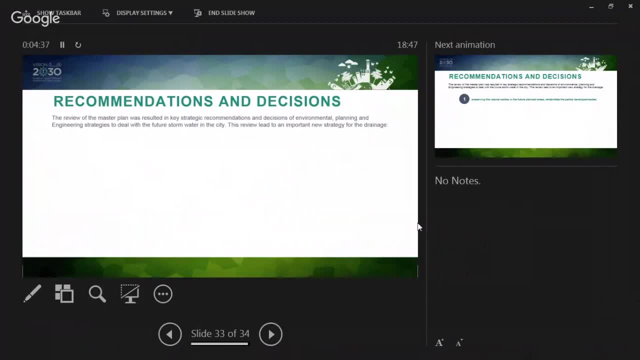 environmental planning and engineering strategies to deal with the future storm water in the city, and this review led to an important strategies. the first one was preserving the natural waters in the future planned areas and rehabilitate the past partial developed. what is use the sustainable urban drainage systems. 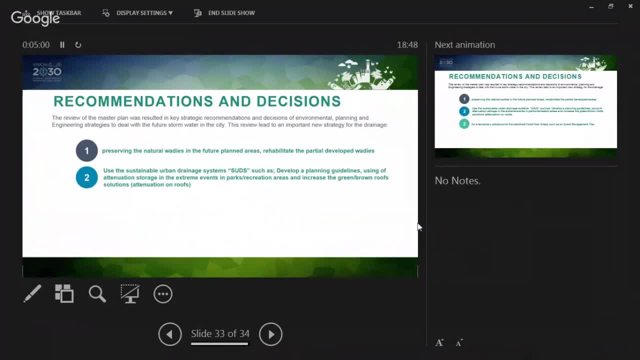 develop a planning guidelines using of of attenuation, storage in the extreme events, such as parks or recreation areas, and increasing the green or brown roofs solutions. also, we have asked to do a temporary solutions for the identified flood risk areas, such as an event management plan. a new strategy of the city is in preparation to handle the risk. 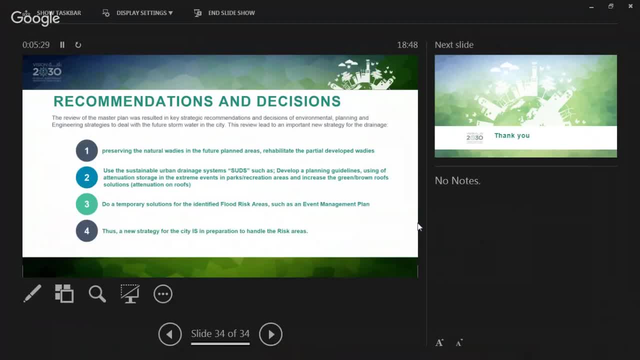 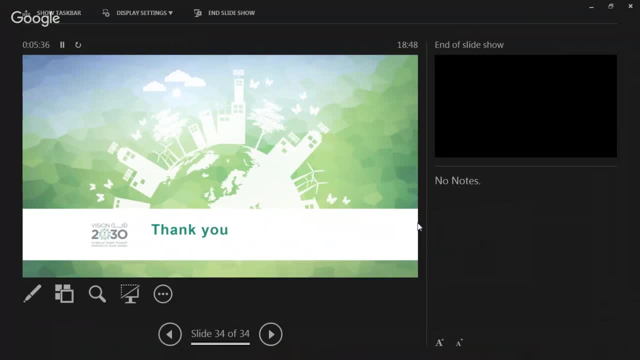 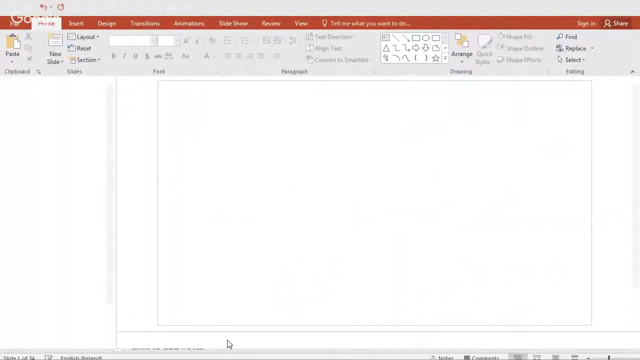 if the risk is there, and thank you very much for your attention and we will see you in the next video. Thank you very much. Thank You, engineer Faisal. I would like to call for the floor engineer Hashim Saad. Thank you, engineer Faisal. I would like to call for the floor engineer Hashim Saad. 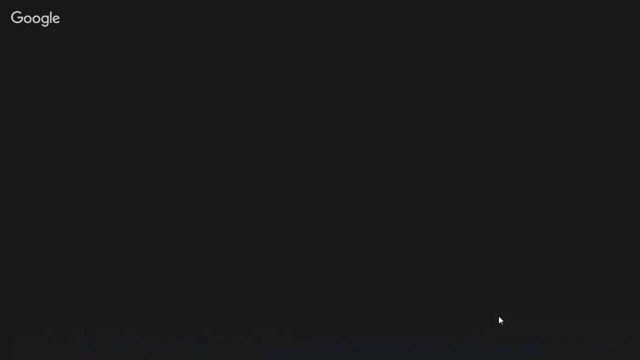 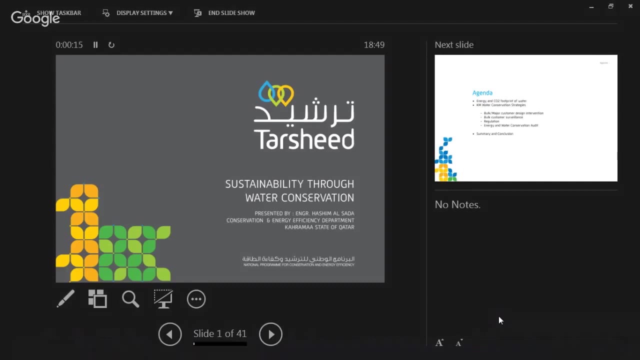 sorry, Hashim Saad, sorry. Hashim Saad is a head of the conservation technology section, conservation and energy efficiency department at Kahraman. he was awarded an MS degree in sustainable engineering from the Luperbrough University in the United Kingdom. engineer Hashim has two patent under his name, and in the solar energy field. and 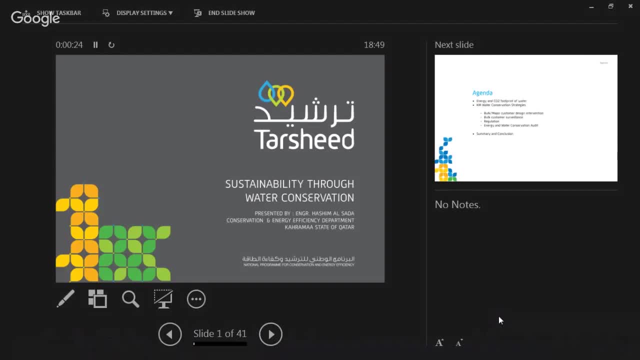 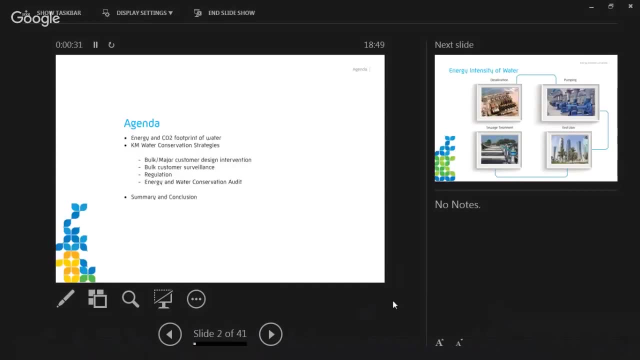 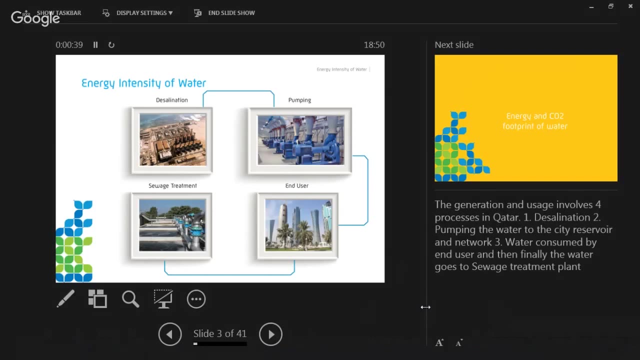 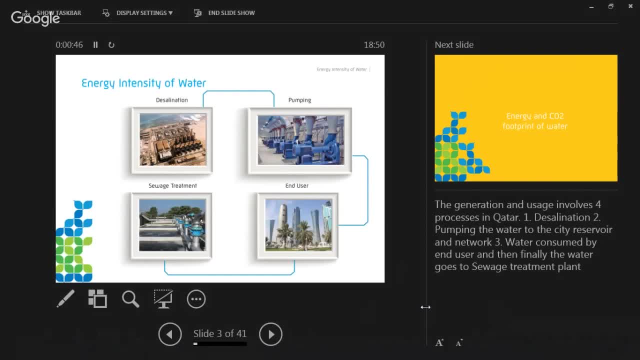 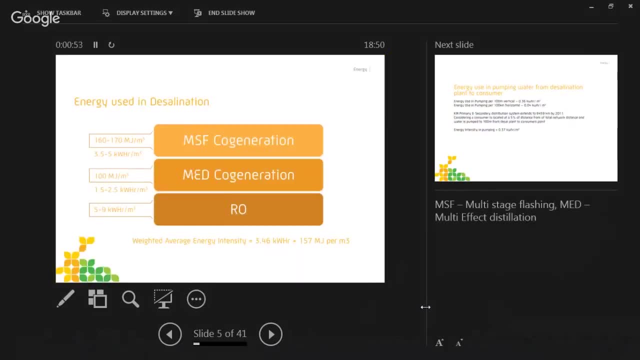 Energy of water. we have four steps. first of all, the destination- pumping and the end user. After that the treatment, Energy and CO2 footprint for water. So MSF is 160 to 170 megajoule per cubic meter. 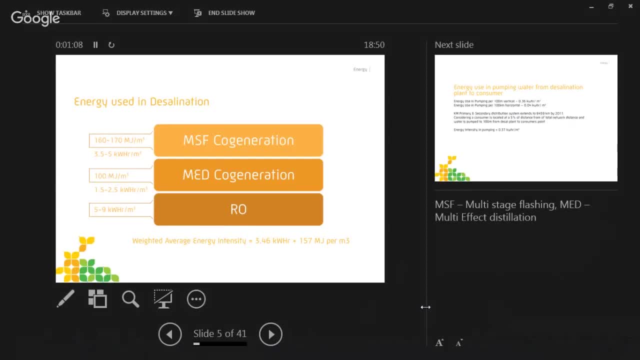 which is 3.5 and 3.5 and 5 kilowatt hour per cubic meter. MED is 100 megajoule of cubic meter, 1.5 to 2.5 kilowatt hour per cubic meter. 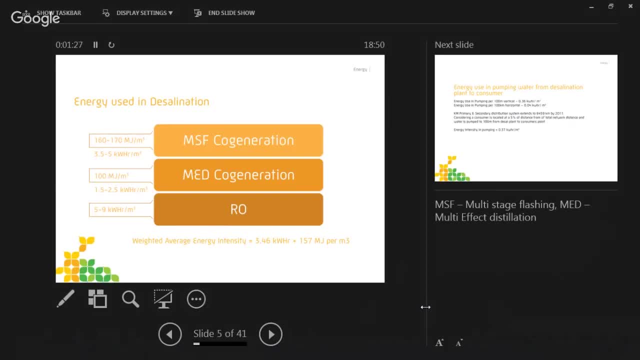 and RO- 5.9 kilowatt hour per cubic meter. So the average for energy here is 3.46 kilowatt hour per cubic meter and plus 157 megajoule per cubic meter. Energy use is pumping water. 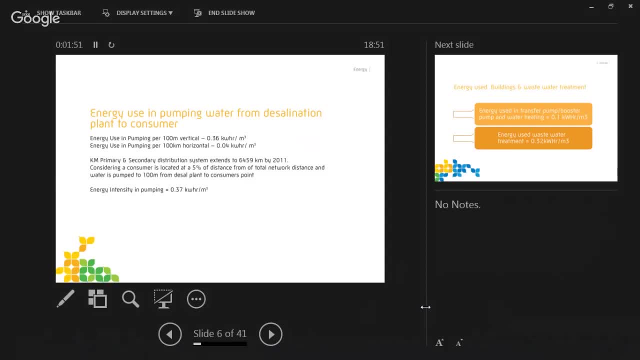 We have vertical and horizontal. The vertical, if we say 100 meter, it's equal 0.36 kilowatt hour per cubic meter. Horizontal: 100 kilometer, it's equal 0.04 kilowatt hour per cubic meter. 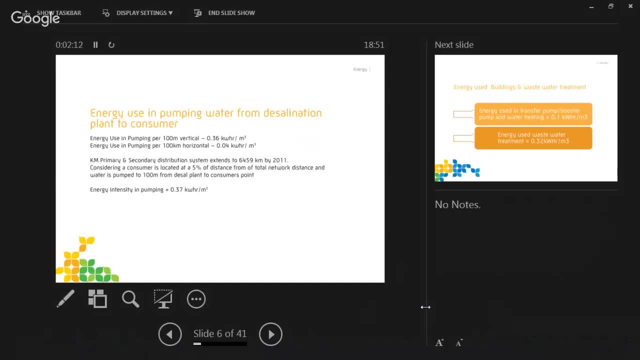 So let's say if we have a customer, he's 5% in distance. The total we have in Qatar for piping the network is 6,500 kilometer. This is by 2011.. So if we say we have a client, he's in 5%. 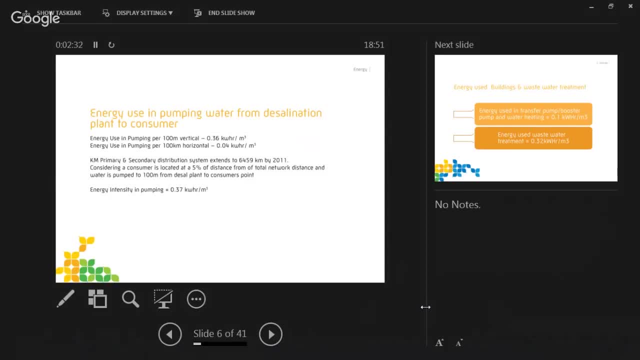 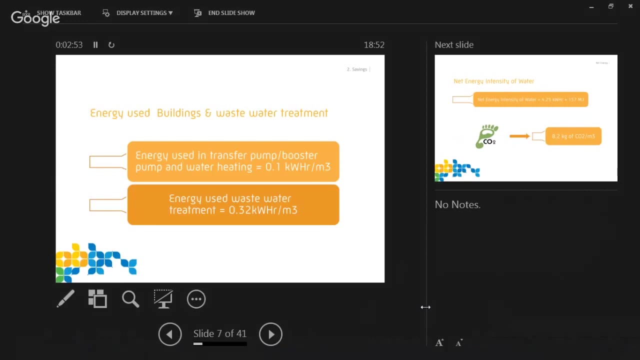 So we have a plant: 100 meter vertical and 5% horizontal. That will equal the energy is 0.37 kilowatt hour per cubic meter. Energy use pumping and the wastewater Energy use and transfer pumping in our buildings and home is 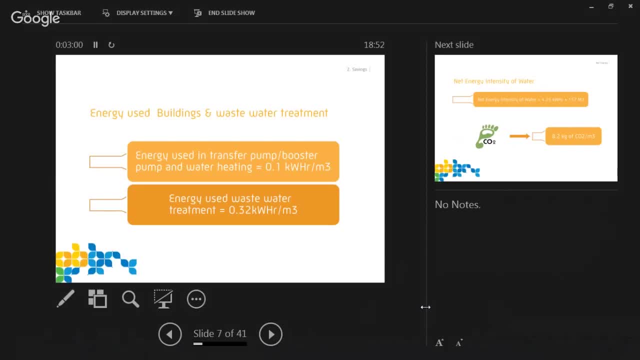 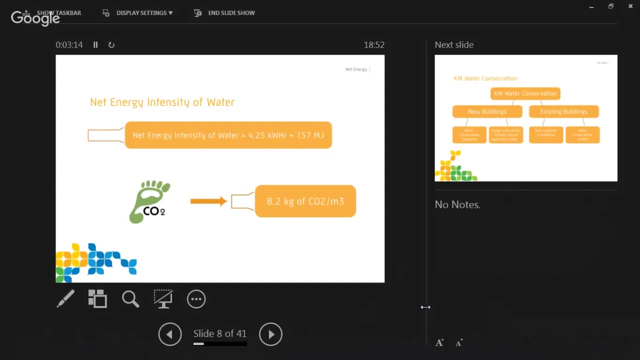 with the heating is 0.37 kilowatt hour per cubic meter. 0.1 kilowatt hour per cubic meter Energy use wastewater is 0.32 kilowatt hour per cubic meter. So the total for all the systems is 4.25 kilowatt hour plus 157 megajoule for the cubic meter. 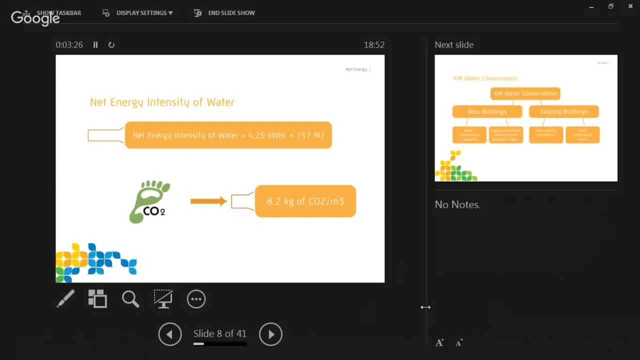 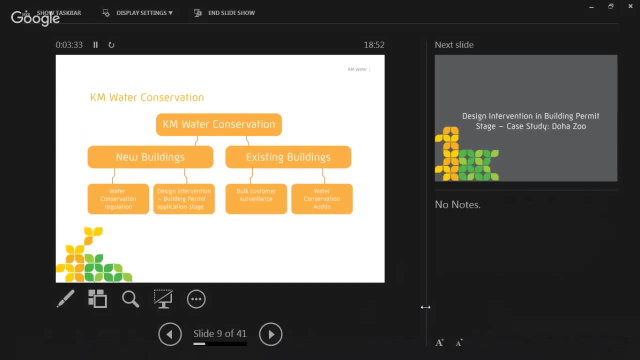 which is equal 8.2 of CO2 per cubic meter, So the total will be 0.6.. KM, which is the organization I represent, Kherama. It has two conservation plans: One for the existing building and one for the new building. 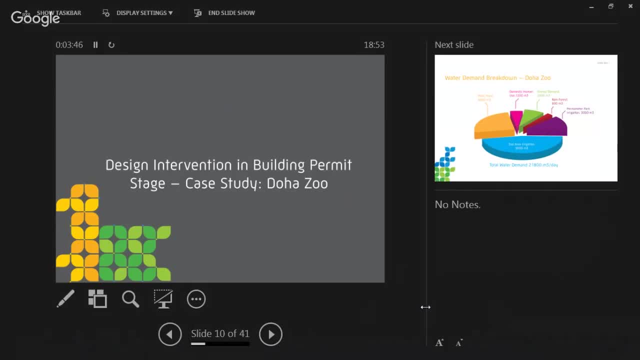 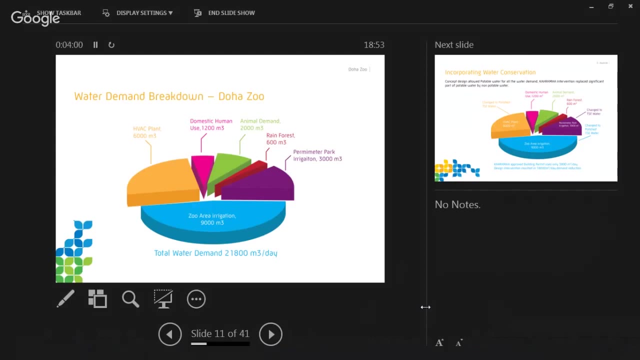 For the existing building. we have a case study. Sorry For the new building we have case study which is Dohazoo. In Dohazoo we have HVAC plant. This is the graph can show for you six thousand cubic meter, the consumption, the demand for the hbac and this is. 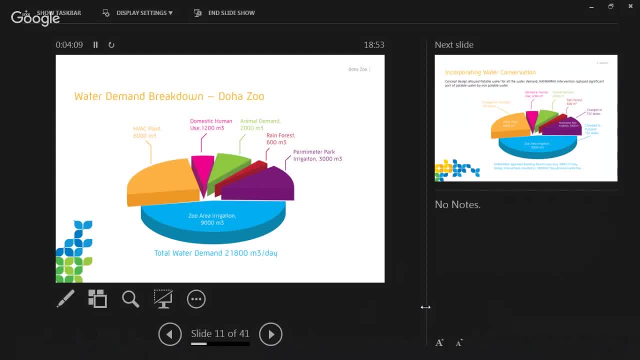 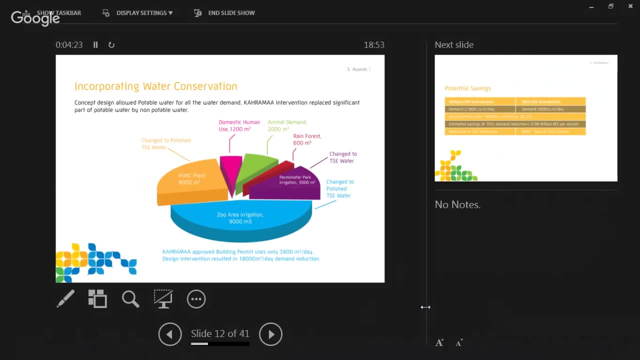 the domestic 1200. so in total of all of these we have 21 800 cubic meter per day. what we done? we change the hbac plant water and the irrigation. we change them to tse, not portable water. what we use it normally we say actually we save 18 000 cubic meter per day for the demand. 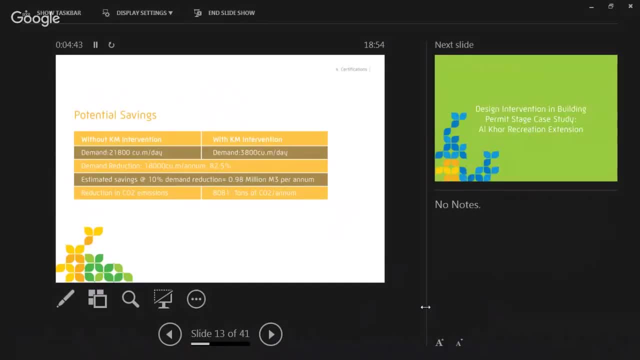 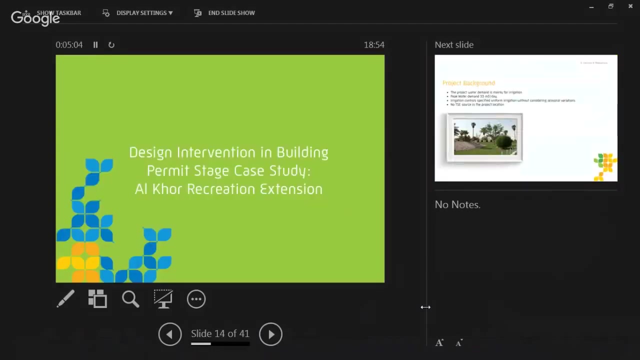 so we save 82.5 percent of the water consumption. what equal, uh? the estimate saving yearly is one million cubic meter and by co2, we are saving 8100 co ton of co2 yearly. there is another example about al-khor, which is a city, al-khor park. 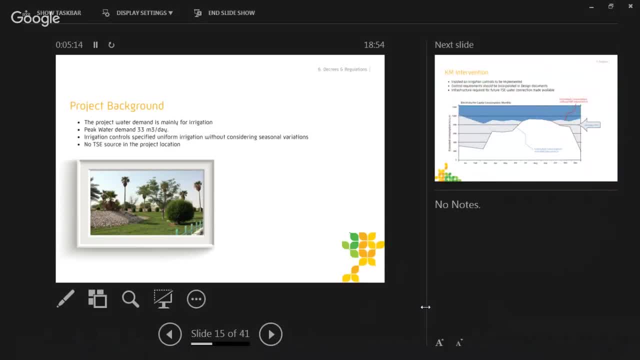 most of the water. the demand is 33 cubic meter per day and the irrigation is is the most consumed there. we change the, the sensor for the water irrigation to seasonal, because we have a different temperature in qatar summer and winter, and we just done that and we 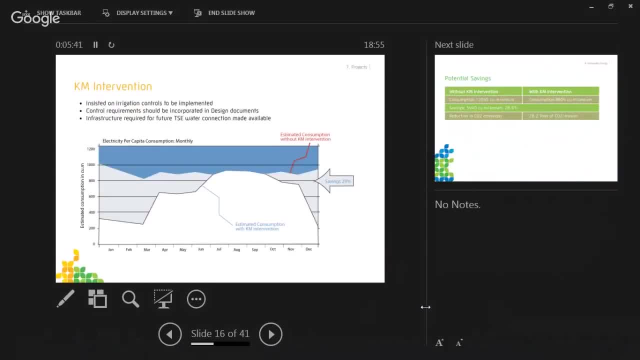 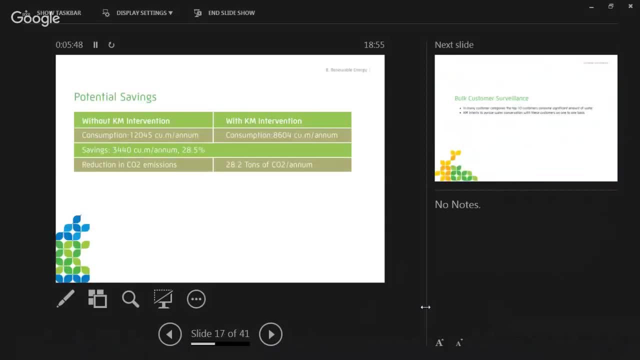 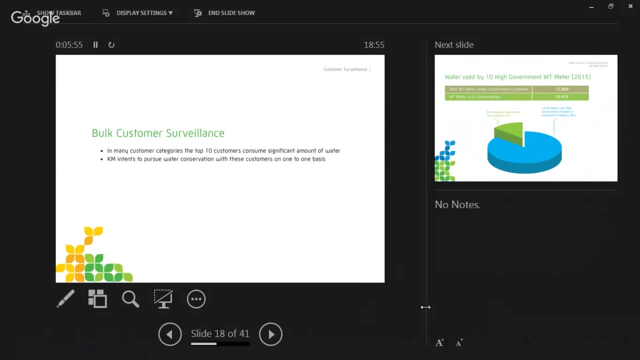 we, we save 29 percent, just to change. we change only the control, which is equal 28 tons of co2 yearly. the bulk customer, the bulk customer back home. we have now a new ideas. we have 10 customer, the the highest 10 customer from each sector. 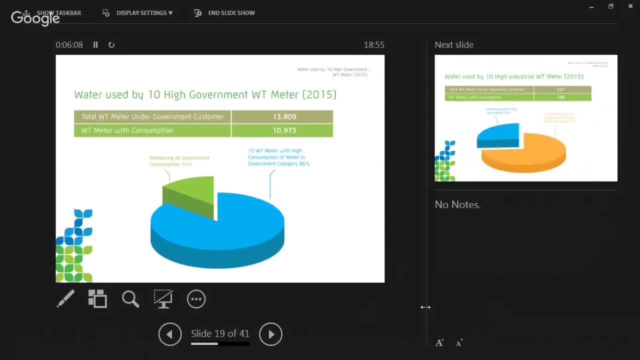 we are uh trying to uh to give only the 10, the 10 customer, the highest 10 customer. you will be surprised of the number. for example, the 10 highest governmental uh customer: it's 86 percent of the total governmental consumption in water. okay and industrial is 77. 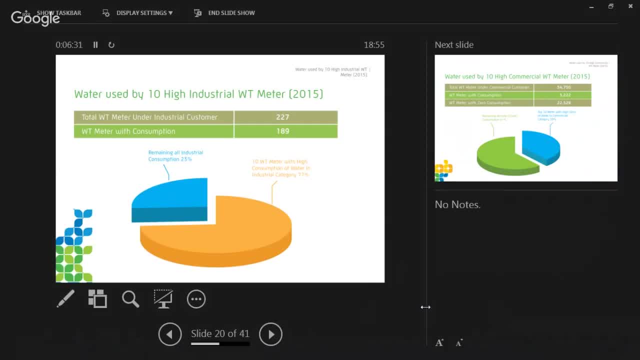 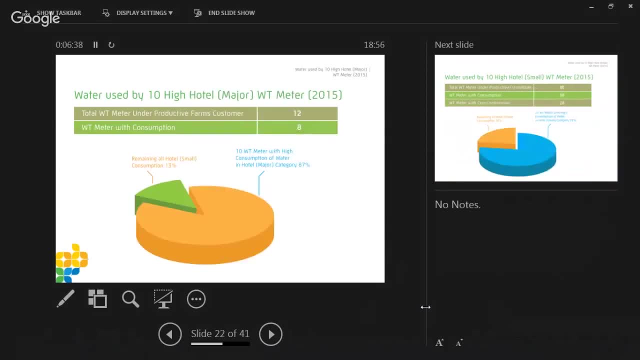 percent, only the top 10.. The 10 high commercial is 39 percent, almost 40. The 10 highest hotel, the major hotel, is 87 percent. The 10 highest hotel, the small hotel, is 74 percent And 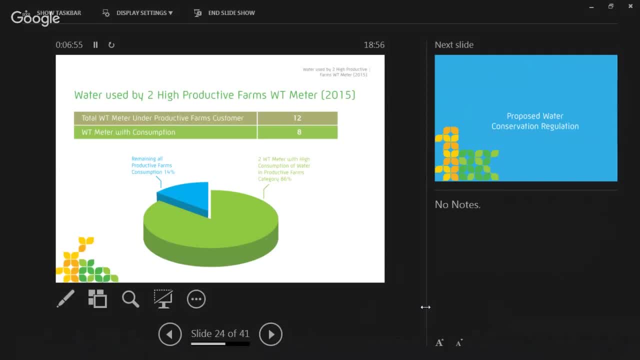 the only two highest productive farm in Qatar. it's 86 percent of the total consumption of water in this sector. So now we are just focused on this: the highest consumption, the highest customer, Protective water regulation. we have a new regulation in Qatar about water. 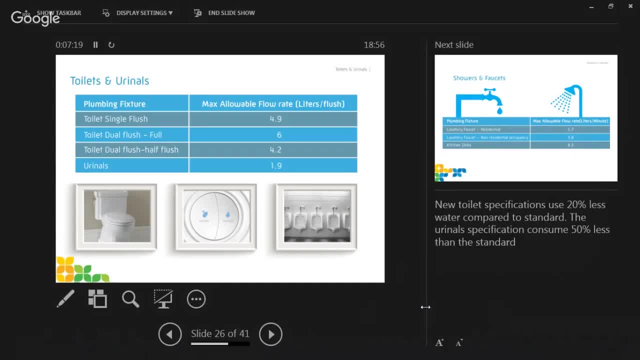 toilet and urinals. We have the toilet: single flash, which is the first one, is 4.9 liter per flush. The total dual flush, the full one is 6 liter And the half one is 4.2 liter, The urinals 1.9 liter per flush. We have also for the shower and factors. 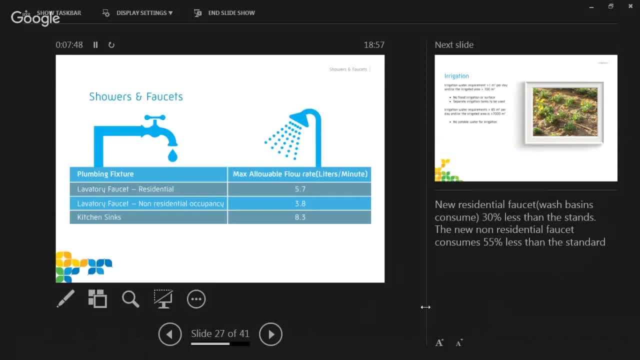 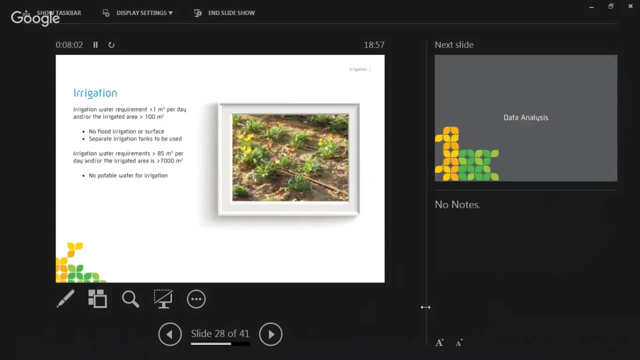 5.7 for the residential factor And we have 3.8 for the non-residential And for the kitchen sink, 8.3 liter. Anything above these numbers will not allow to enter Qatar. We have also a new system for irrigation in Qatar. If the plan is, use one cubic. 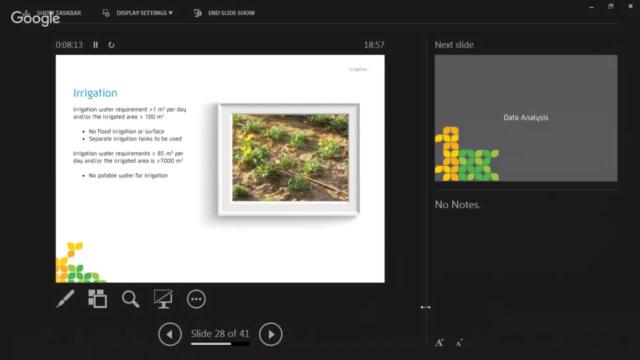 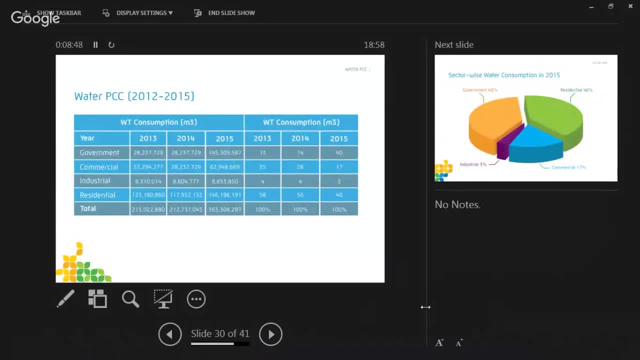 The data analysis. we start from 2012 to plan to do the conservation in Qatar In 2013, and 2014,, 2015,. it's shown here with all the governmental and commercial, industrial and residential. It show here all the data which is here in the graph. It can be: 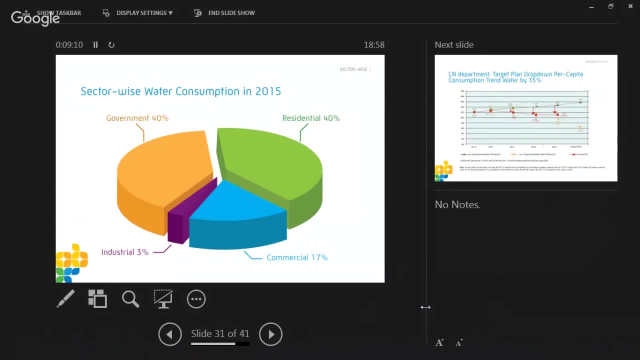 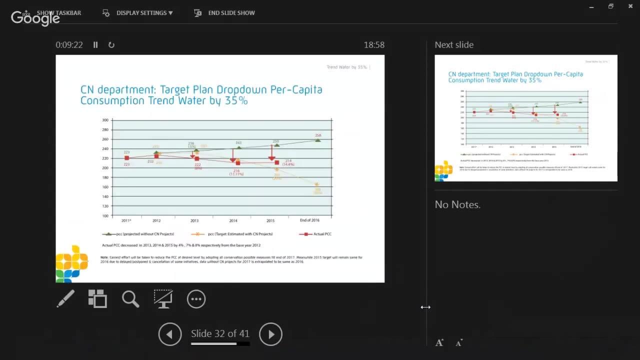 more easier for you You can find. the governmental and residential is 40% each of them. The commercial is 17%. The industrial is 3% of the total consumption in Qatar. The water is 3% of the total consumption in Qatar. 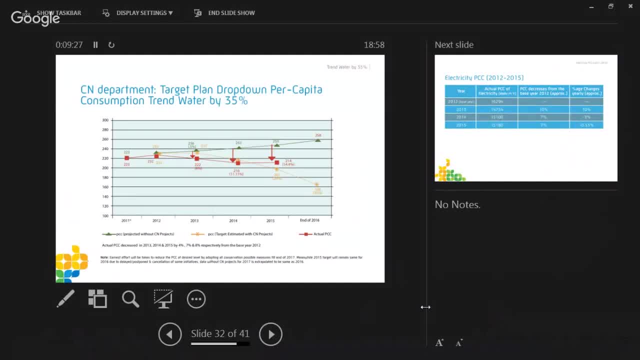 The actual BCC. as you can see the green line, this is the actual BCC. We supposed to have in this day 250 liter per person, a meter of a person yearly, but we save until now 14.4%. our target is very high is 35%. reduce per capital consumption, which is very high. 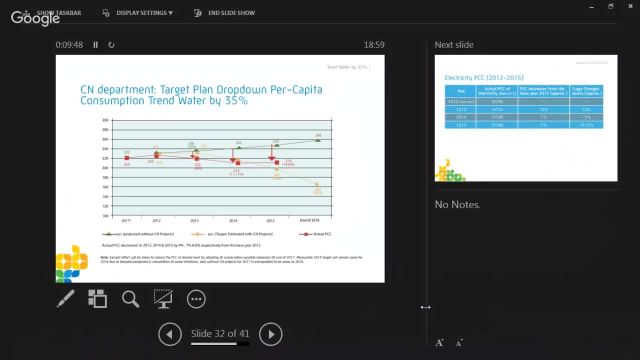 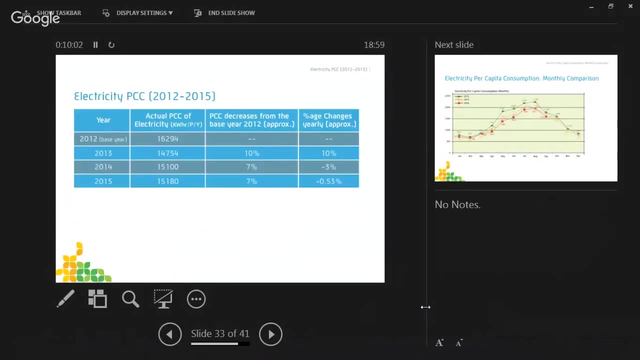 Our target is very high is 35% reduce per capital consumption, which is very high and we know it's possible to reach it. but we challenge ourselves and we put big target for us. the actual bcc- it was in 2016, which is the base year- 16 294. this is for the electricity. 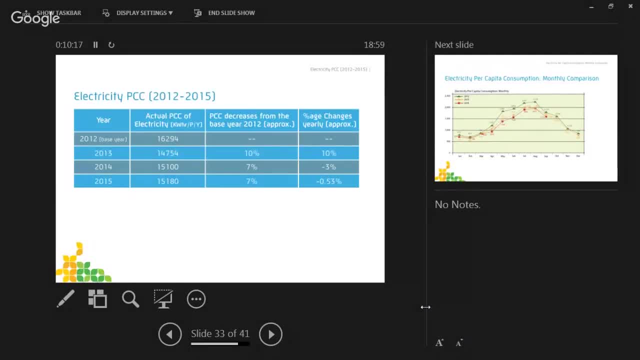 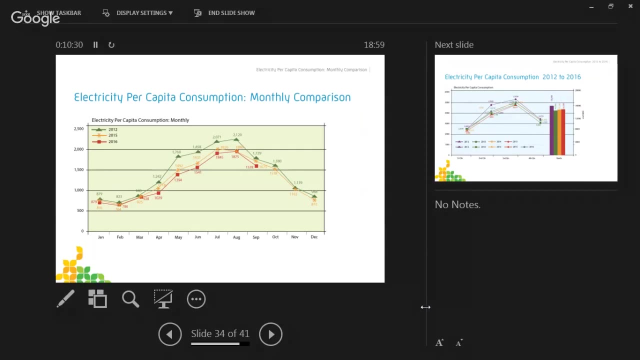 in 2013, we reduce it 10 percent. 2014, we reduce it seven percent. 2015, we reduce it seven percent. and this is the electricity consumption. you can see also the green line, which is the actual what's supposed to be, and the red one what we are doing right now. 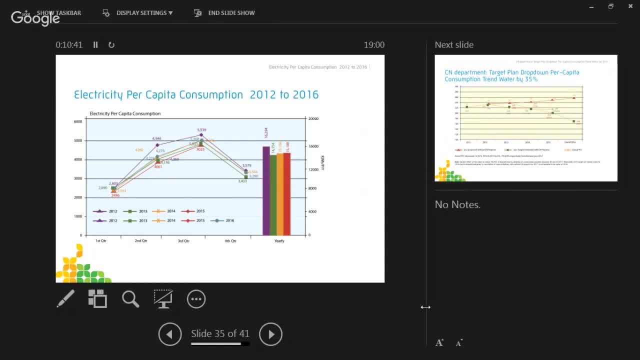 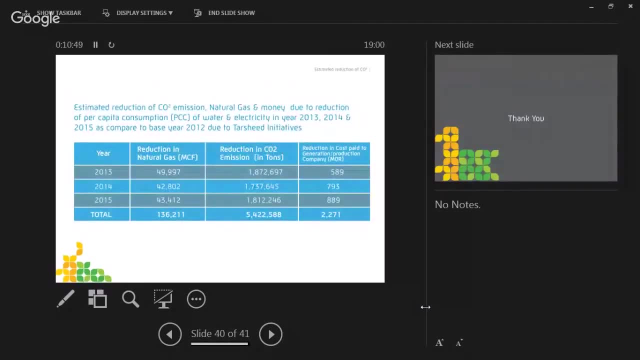 engineer actually have one minute, okay, so this is the demand. uh, this is the total here in this graph will show what we uh our goal until 2015.. we save for national gas: uh 163 000 million cubic feet and we save 5.5 million tons of co2. 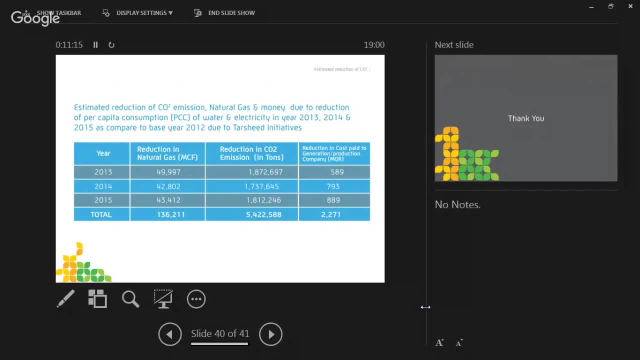 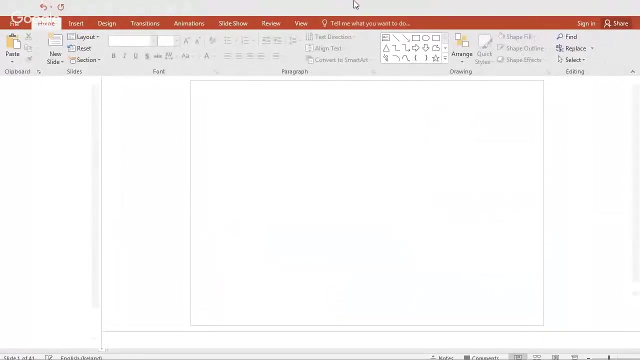 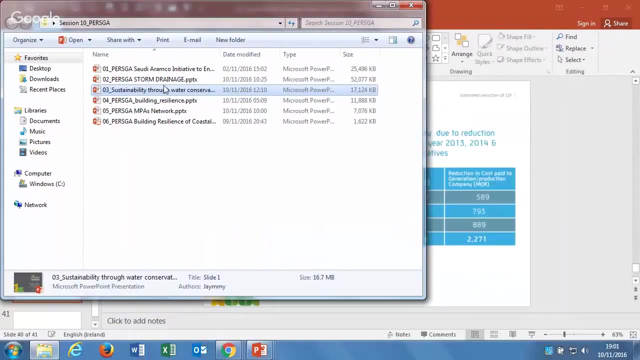 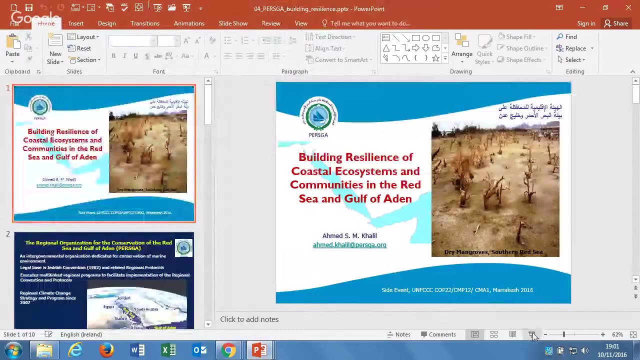 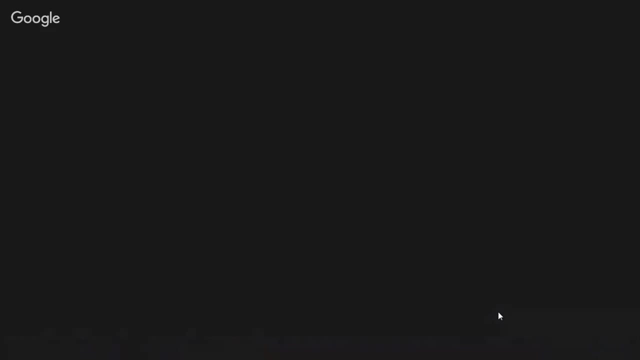 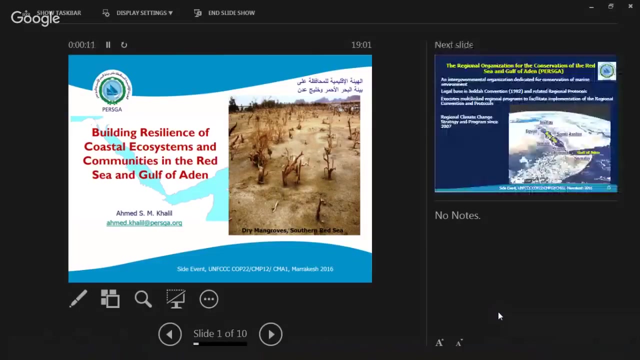 2 billion 270 million real, which is equal 622 million dollar. we save in this three year by only saving the consumpt for water. thank you very much. thank you, engineer, thank you, thank you, thank you, hello hello Persica, for conducting regional mangrove assessment and development in the region. 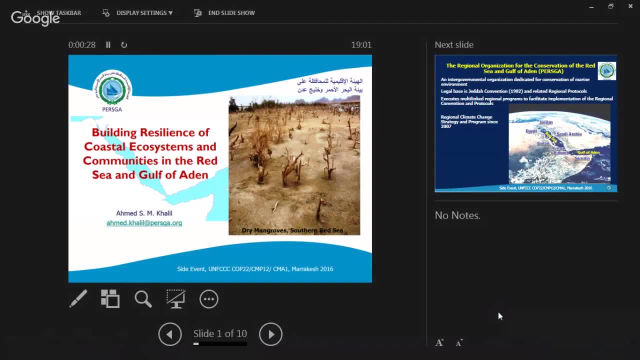 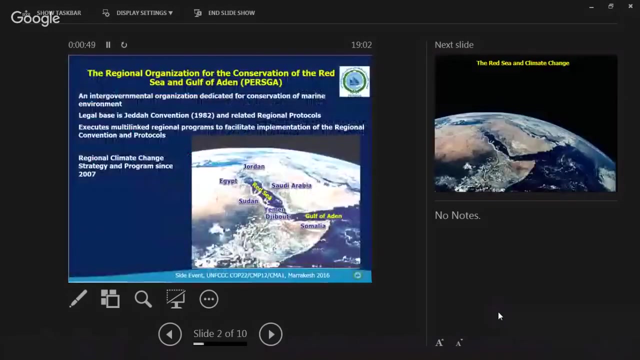 by the time somebody. so I will focus on my presentation on efforts of Persica, the regional organization for the conservation of the environment of the Red Sea and Gulf of Aden, in building resilience of coastal ecosystems and communities in the Red Sea and Gulf of Aden. the legal organization for the 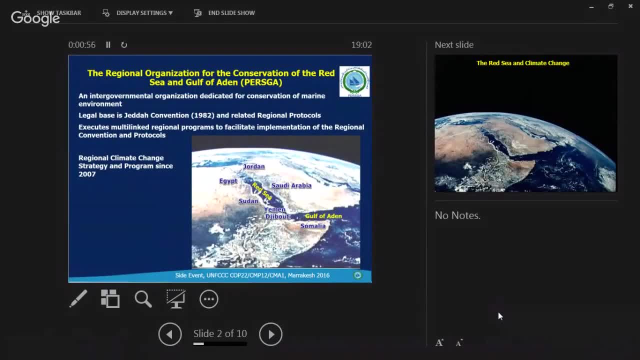 conservation of the environment of the Red Sea and Gulf of Aden is an intergovernmental organization dedicated for conservation of the marine environment in the region. it has legal base is ghetto convention signed in 1982 by the member states- seven member states bordering the Red Sea and Gulf of Aden. 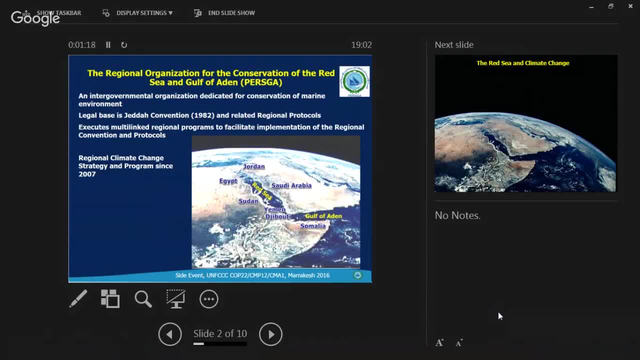 including the Red Sea and Gulf of Aden, and the Red Sea and Gulf of Aden are in Jordan, Egypt, Saudi Arabia, Sudan, Djibouti, Yemen and Somalia, Persica. the regular convention also has four related regional protocols and action plan, basically developed a regional climate change strategy and 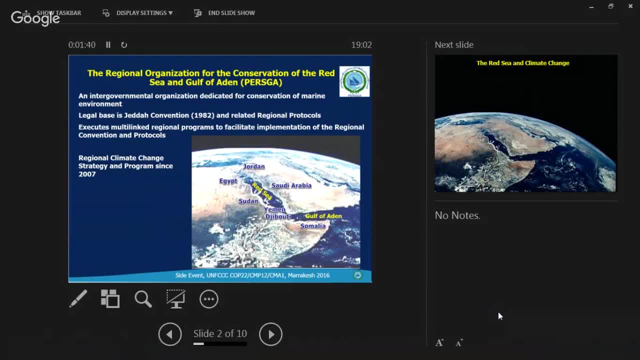 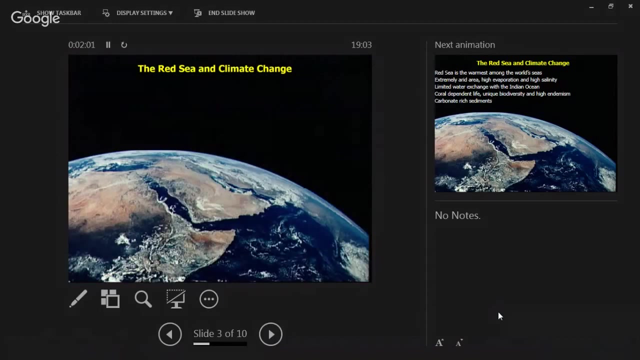 program since 2007 and this program conduct capacity building and sinn of winning, resource contribution and detailed action plan and many other aspects of building zillian's adaptation and also because system based mitigation activities. let us first maybe I will summarize some of the features the Red Sea related to Pokemon change. we should have implications. climate change in love is war is war and they were human beings against climate change- a lifetime change, as the Red Sea is the Red Sea. in談��うرہ 틈. 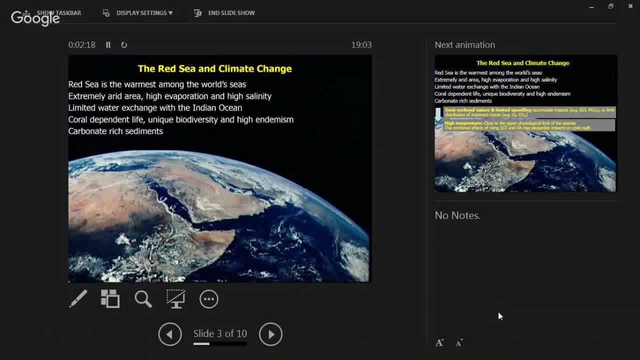 warmest among the oil it sees. it's extremely. it's located in extremely dry area with high evaporation and high salinity. there is limited exchange with the Indian Ocean, throws a narrow and shallow bubble, Mendeb and the Red Sea is a coral dependent. see, life in the Red Sea depend on coral and it has unique 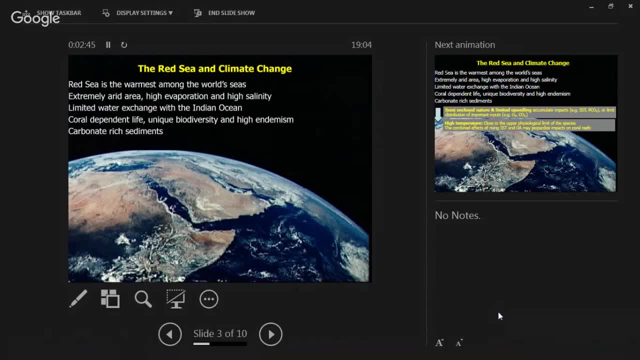 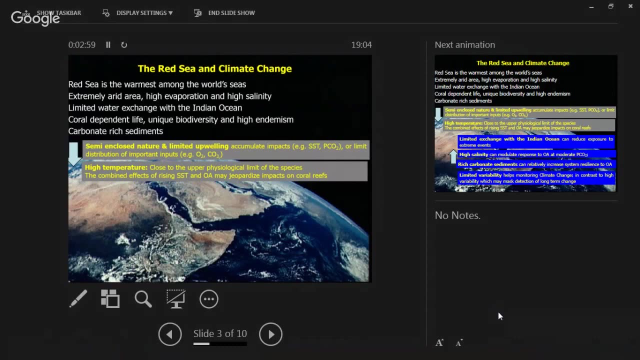 biodiversity and high endemic gel. many endemic species in the Red Sea is. the Red Sea area also has rich carbonate sediment. this could have some medications. the negative ones are that the semi-enclosed nature of the Red Sea may also limit and the limited upwelling or as well could accumulate impacts any. 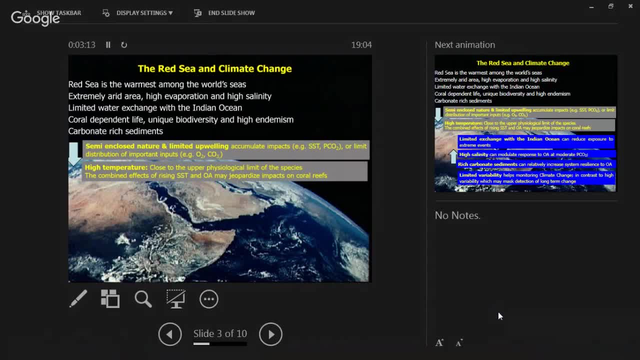 kinds of impacts, including climate change. impacts on also limit distribution of important inputs like oxygen and carbonates, which are important for corals. the high temperature also is close to the other psychological limits of of the species, and the combined effects of increasing surface temperature of the sea or the 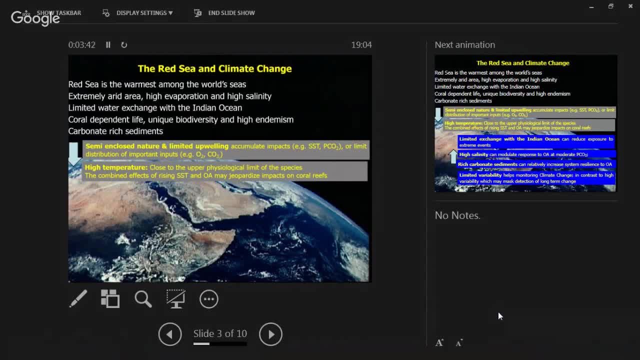 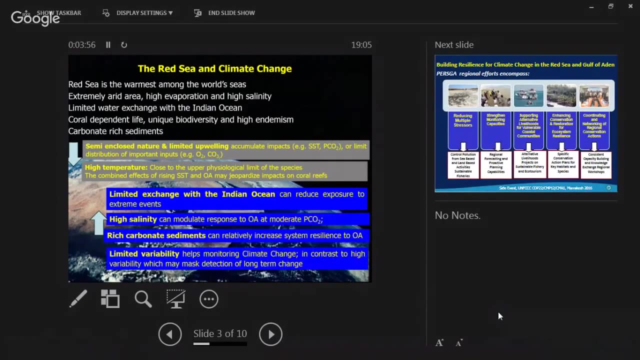 warming of the sea water, with the ocean acidification, have impact on the corals and could jeopardize the life in the Red Sea. they are also some positive aspects of these features that the limited exchange with the Indian Ocean can reduce exposure to the extreme events such as Nino or extreme climate change impacts, and the high salinity can. 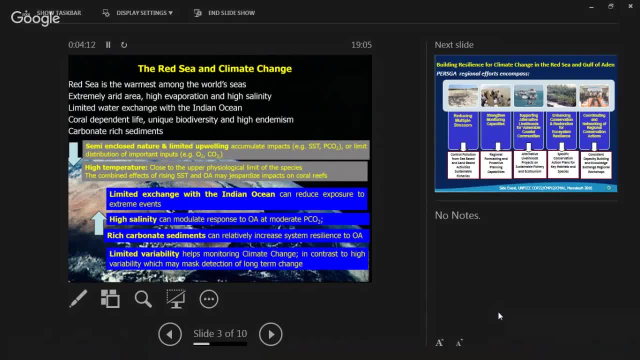 modulate ocean acidification, but at moderate pressure of carbon dioxide. the rich carbonate sediments provide relatively some resilient system or some resilience for system to adapt or to be resilient for ocean acidification. the limited variability, the seasonal variability in the Red Sea helps in monitoring climate change and detection. 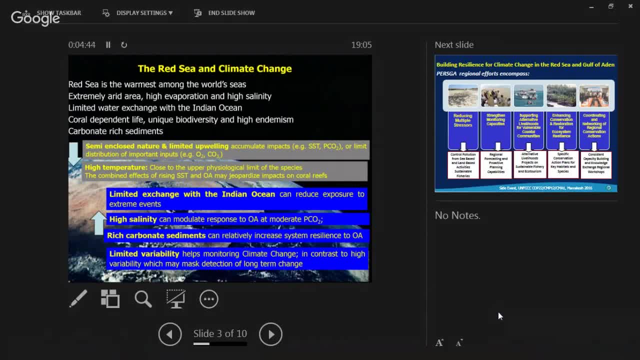 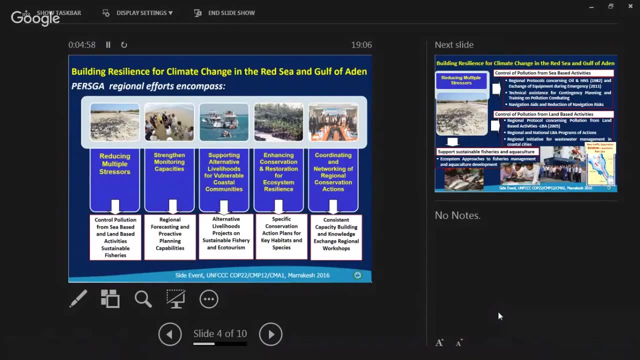 of climate change in the Red Sea and in the Indian Ocean, as well as the climate change which is maybe variability is very high in other seas. which mass detection of long-term change like climate change. these are some features of the Red Sea. now what Bersiga is doing for building resilience? this: 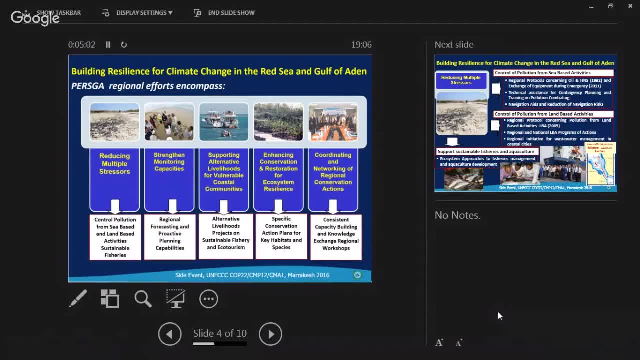 encompass many areas: reducing multiple stressors to increase the resilience of the ecosystem. strengthening monitoring capacities to strengthen also capacities for forecasting, proactive planning capabilities. and also supporting alternative lifehood and vulnerable communities, especially coastal fishermen communities. and enhancing conservation restoration for ecosystem resilience. and coordinating the regional efforts for regional conservation of the member states and conservation actions. 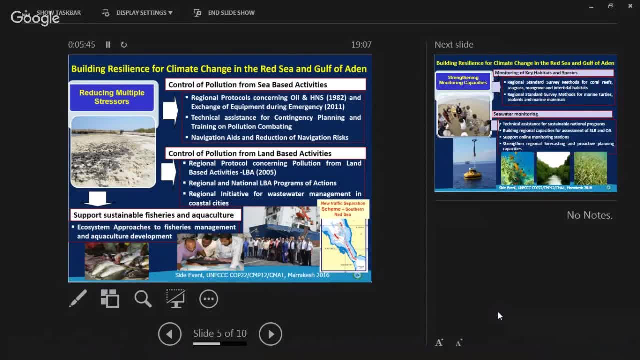 concerning reducing multiple stressors, Bersiga has three programs control of pollution from CBS activities and these are based on regular protocols concerning oil and hazardous uh. this is what signed in 1982 and emergency on contingency plans were developed for the countries and regular has also developed. this will also provide technical assistance for continuous learning. 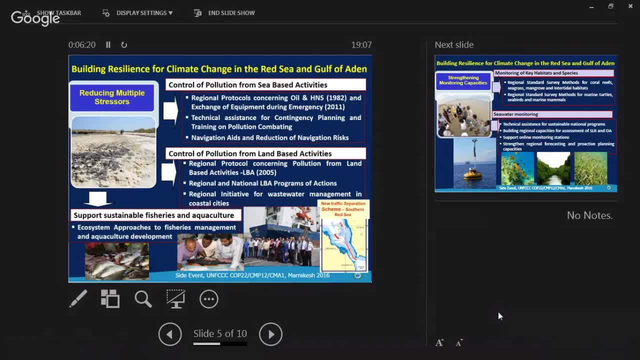 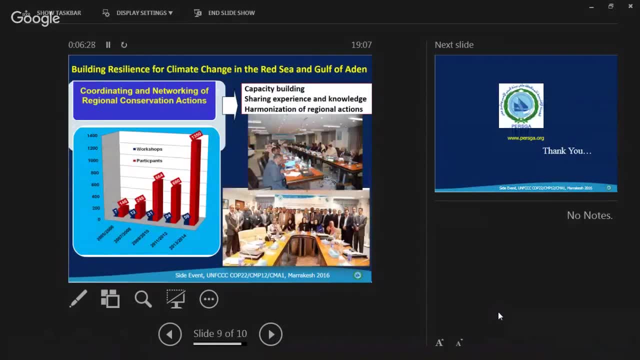 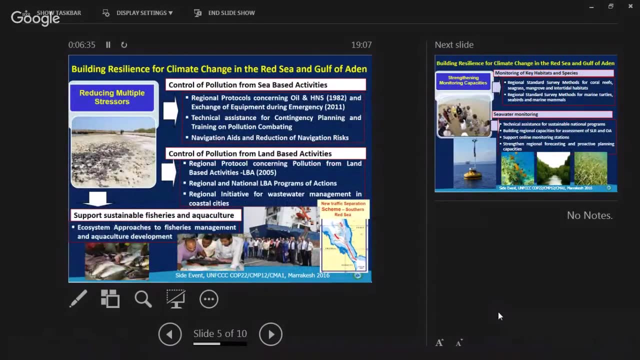 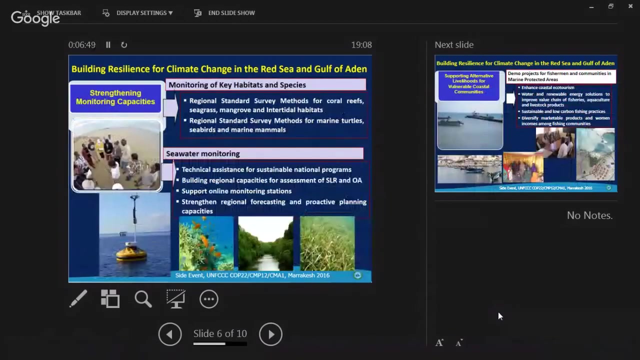 and training on pollution combating and navigation aids, reduction of navigation risk and especially in the southern red sea. and also there is program on fisheries and now focusing an initiative on implementing ecosystem based fisheries, to fish, to management of fisheries and development of aquaculture, strengthening monitoring capacities. they are programs for monitoring key habitats and species. 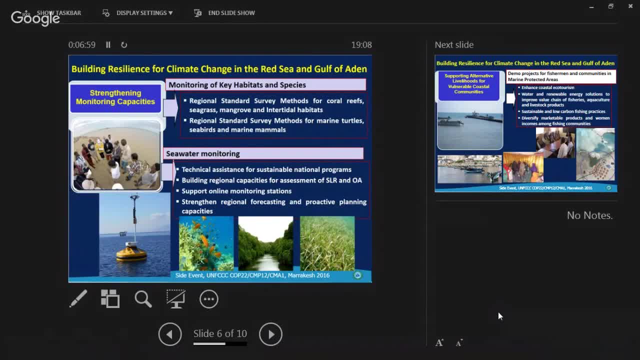 the main key habitats are mangroves, seagrass beds and coral reefs- basically developed regular standard methods for monitoring such habitats and also for key species, key animal groups like marine turtles, seabirds and marine mammals. there is also technical assistance for strengthening national monitoring of sea water and also training capacity building. 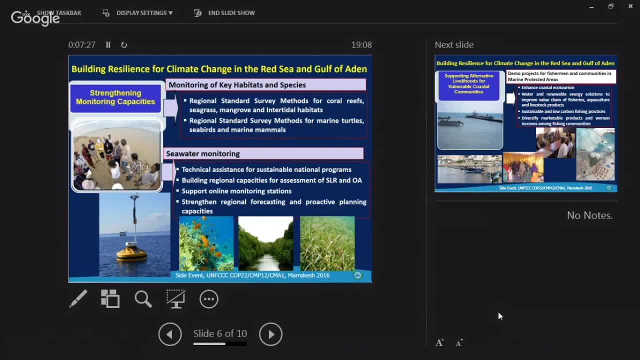 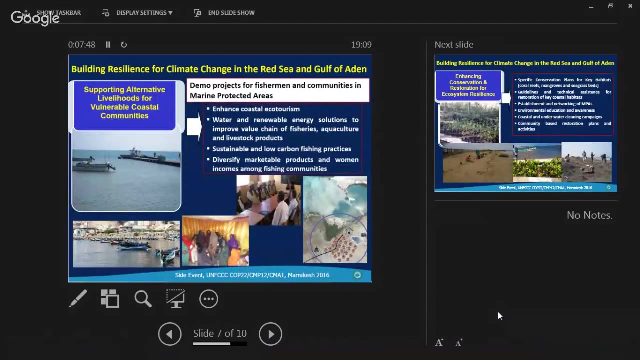 to monitor a ceiling rise and ocean acidification, and also recently was even supported online in the selling of online monitoring stations, like in jordan, and also strengthening the focus on non-extractive use of marine living resources, enhancing coastal ecotourism and providing also water. 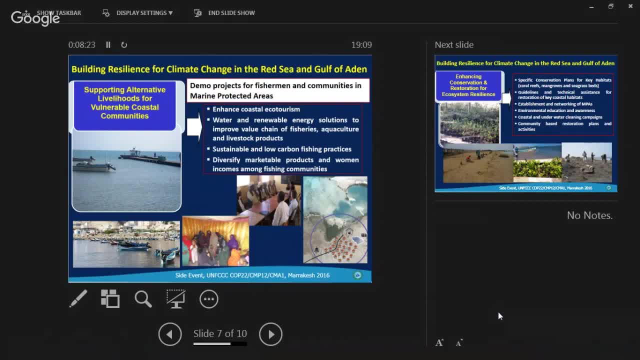 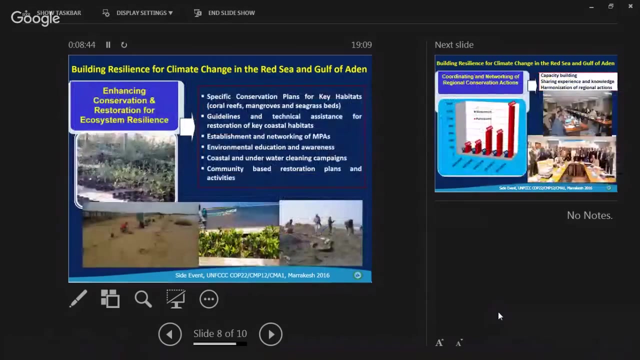 and renewable energy solutions to improve value chain fisheries, agriculture and livestock products, and also provide technical assistance for low-carbon fishing practices and diversify marketable products, especially for women, to increase women's incomes and empower women among fishing communities. 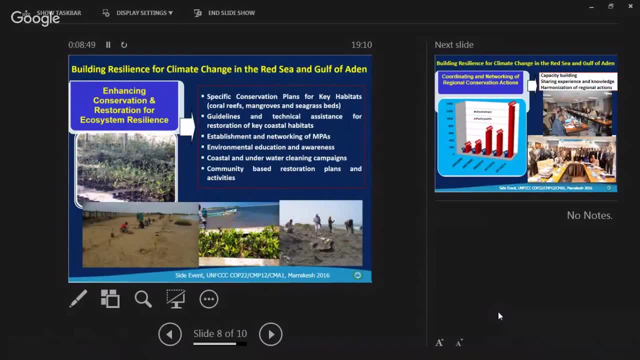 Also enhancing conservation restoration for system resilience. This is based on specific conservation plans for key habitats developed also at national and regional levels, and there are guidelines developed for technical assistance and technical assistance provided for restoration of key coastal habitats like mangroves and coral reefs. 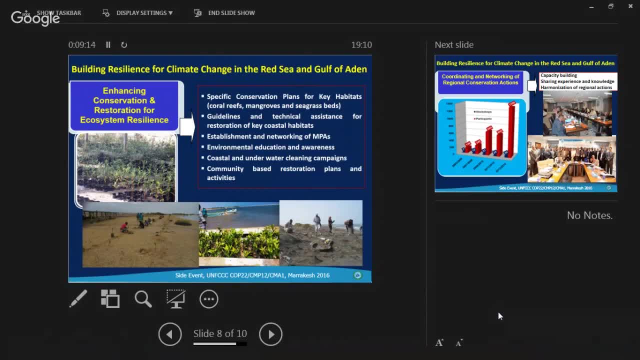 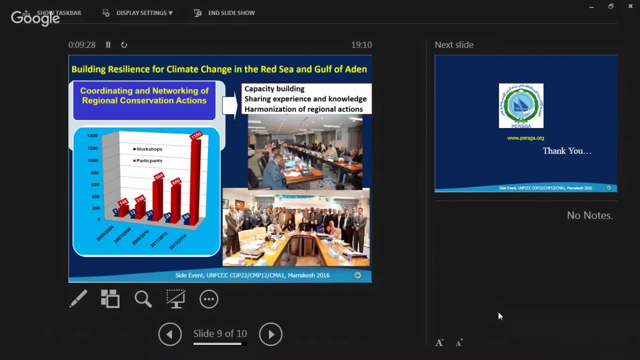 One minute, Ahmed Okay and environmental irrigation program. and there's also coastal and water cleaning campaigns, awareness campaigns and community-based restoration plans. And finally, the Versiga is a forum for conducting regional forum for conducting regional meetings, coordinated meetings and training. 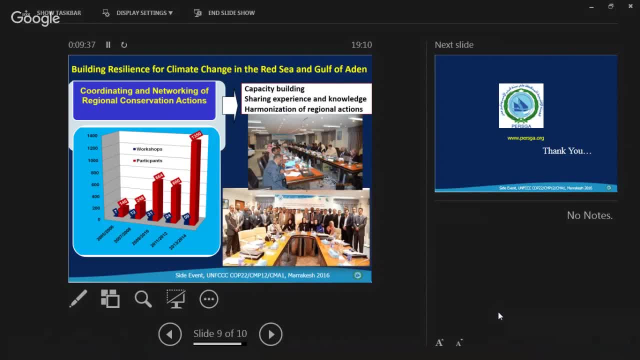 annual training program. This provides capacity building, sharing experience and knowledge among member states and also with neighboring regions, and harmonizing of regional actions, And actually this has been this role has been increasing The number of workshops and participants in Versiga forum. 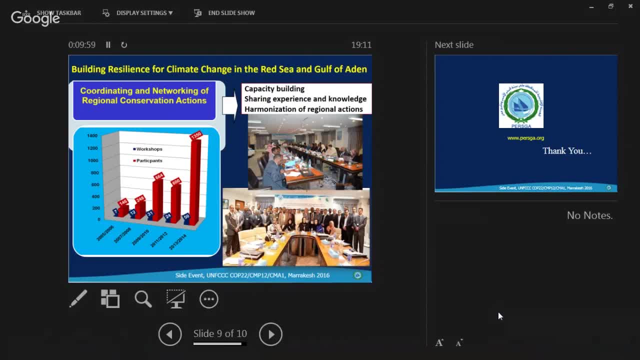 has been increasing in the last. we almost conduct now around 50 workshops per year or meeting, regional meetings, And in the last pandemic the participants are exceeding more than a thousand participants, experts and stakeholders in Versiga meeting. Thank you very much. 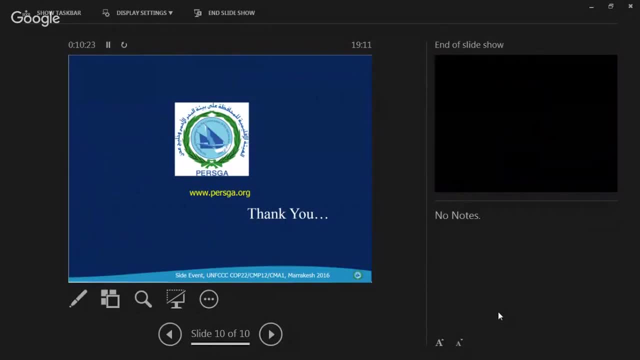 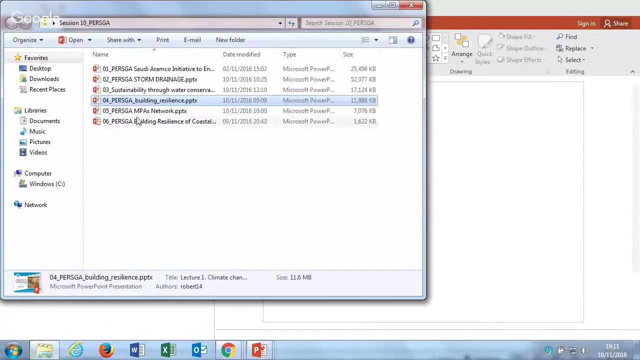 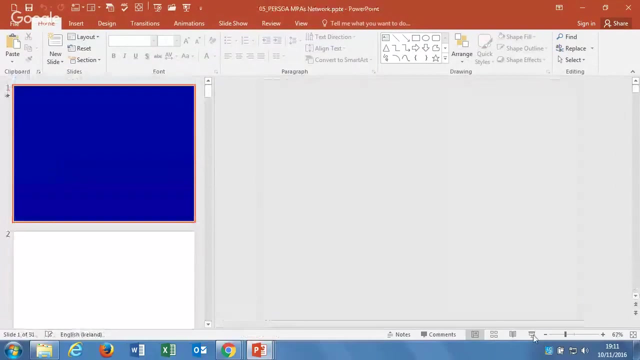 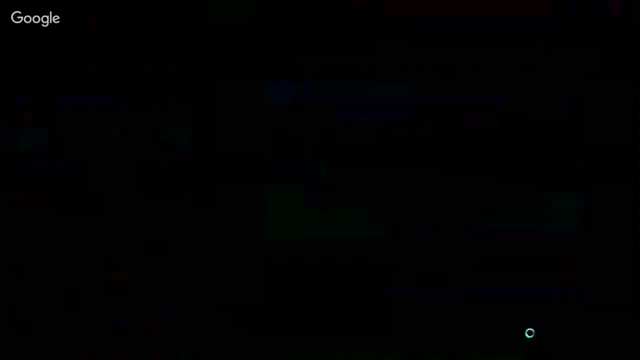 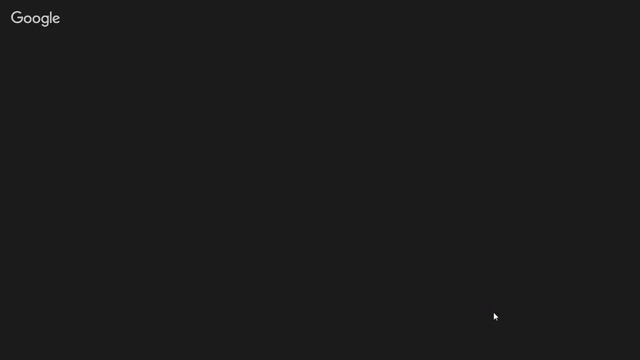 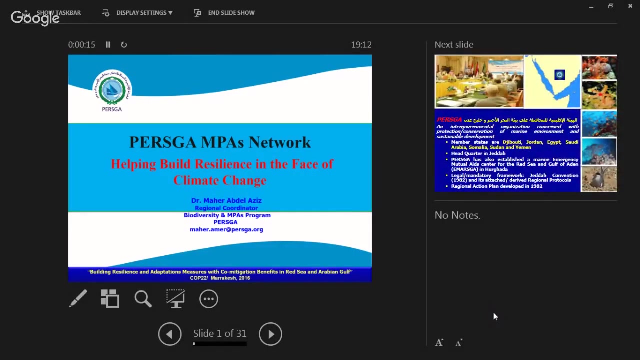 Thank you. I would like to call for the floor Dr Maher Amr. Dr Maher has an over 23 years practical experience, mainly along the Red Sea, in marine environmental investigation, planning, baseline surveys and monitoring program, Starting from 2011 until now. the Department of Marine 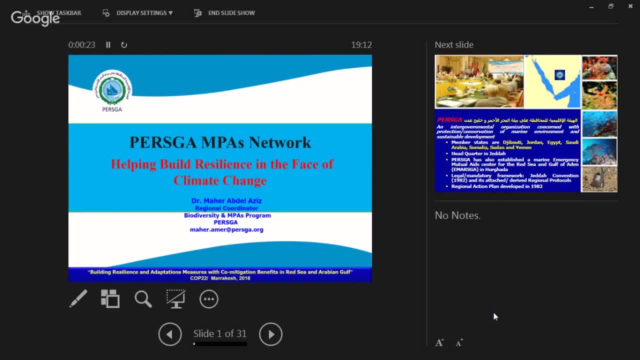 Thank you, Dr Maher worked at the Persica Regional Coordinator of Biodiversity in Marine Protected Areas Program. Good evening everyone. I am going to throw some light on Persica Marine Protected Areas Network for helping build the resilience in the face of the climate change. 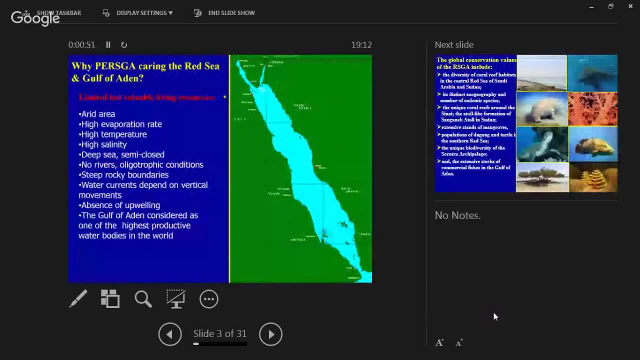 As we know, the Red Sea is located in an arid area. like my colleagues, Ahmed said, The Red Sea is located in the most warmest area in the world, characterized by high evaporation rate, high sea surface temperature, high salt content, and it is a deep sea, semi-enclosed. 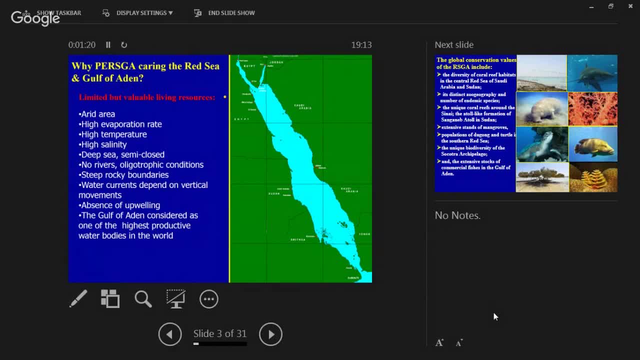 And it is a deep sea semi-enclosed. And it is a deep sea semi-enclosed. We are trying to maintain the rocky boundaries. There is no rivers flowing in the Red Sea. that leads to an oligotrophic sea. 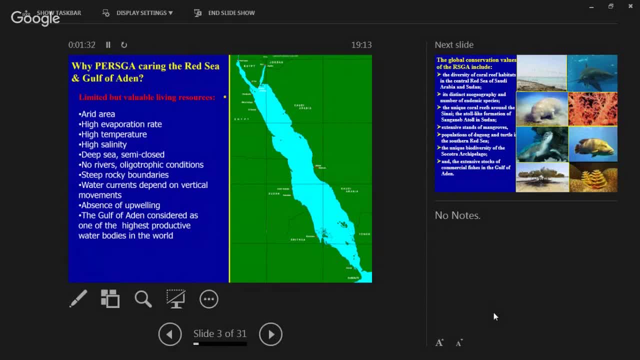 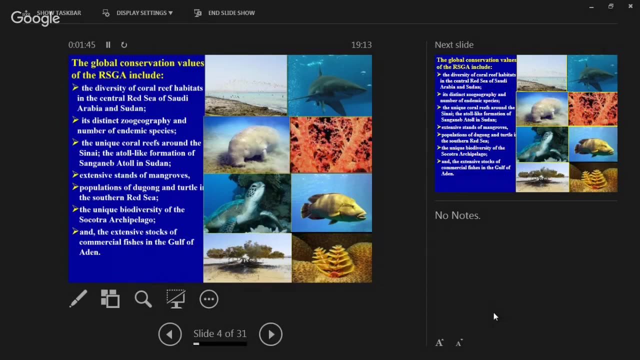 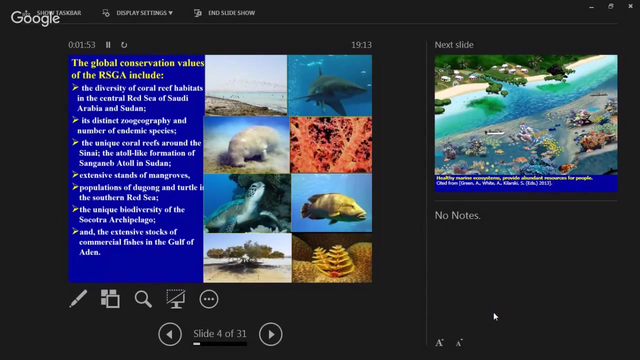 and this condition is perfect for the occurrence and flourish of the Kura Reef. On the other hand, the Gulf of Aden is considered as one of the most productive water-based in the world. first, the original, the global value of the this sea coming from the diversity of coral reef. 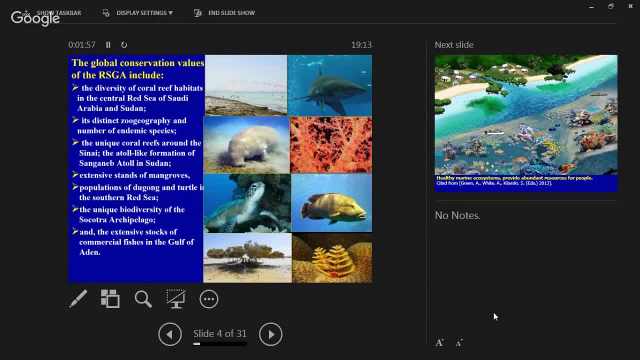 habitat in the central sea, on the in saudi arabia and sudan, the distinctive geography of number of endemic species and is in the middle. the unique coral reef around the sinai in egypt and the atoll-like formation in sanganib in sudan, and the extensive 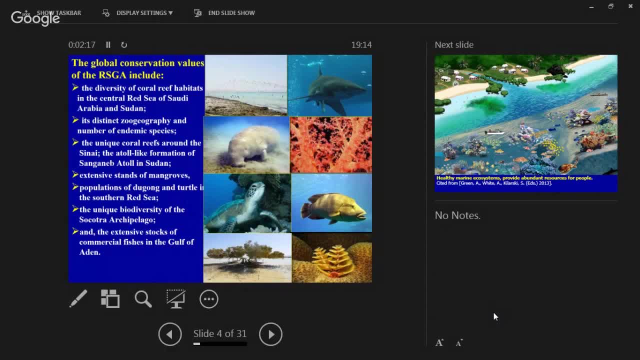 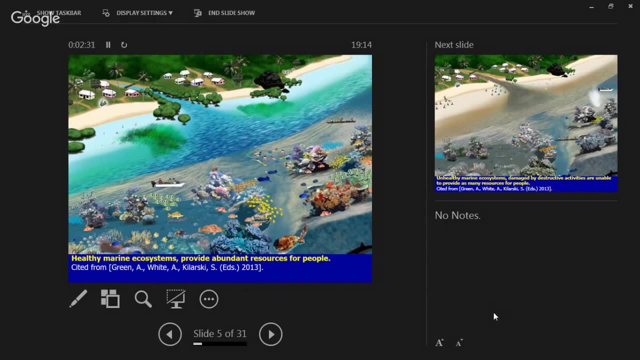 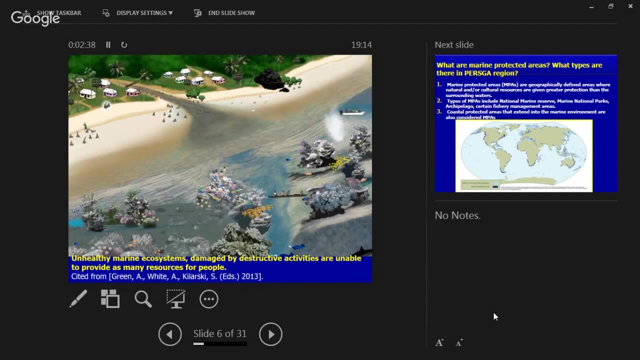 stance of mangrove along the whole courses of the sea, the unique biodiversity of socotra archipelago in yemen and the extensive stock of commercial pieces in the gulf of adam. so healthy marine ecosystem provide abundant resources for people, while unhealthy marine ecosystem, damaged by destructive activities, are enabled to provide as many resources. 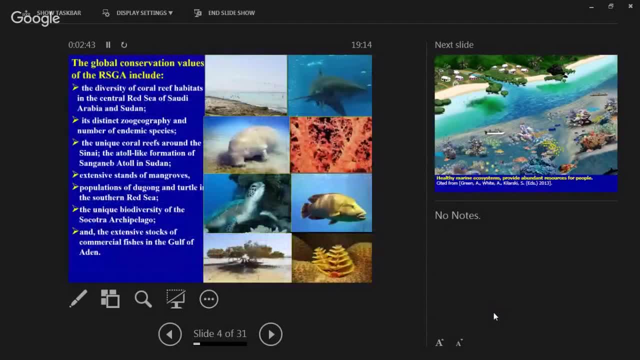 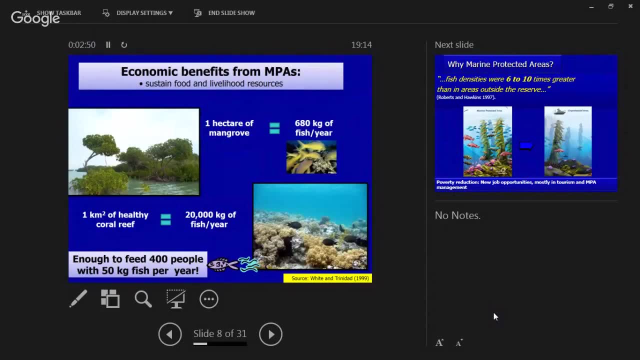 for people. the economic benefit of mpas to sustain food and livelihood resources. for example, one hectare of mangrove may produce more than 600 600 kilogram of fish per year, and one square square kilometer of uh. healthy coral reef may produce 20 000. 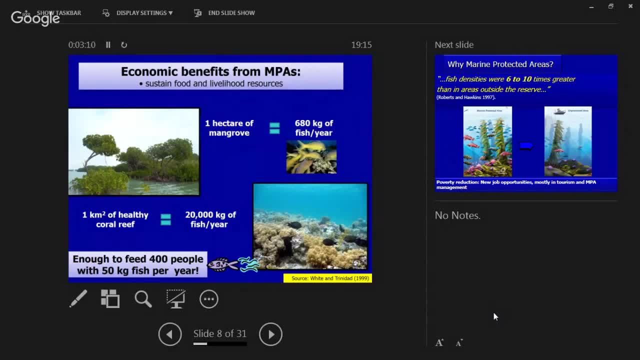 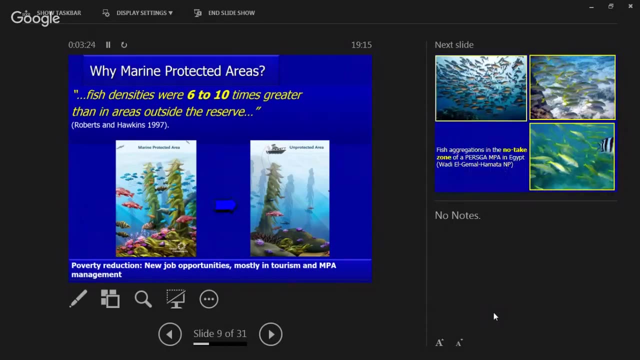 kilograms of reef. that is enough to feed the marine ecosystem and the marine ecosystem of the sea to feed 400 people with 50 kilograms per year. also, the dynasty and the abundance of fish increased inside the mpa more, six to ten times other than outside of. 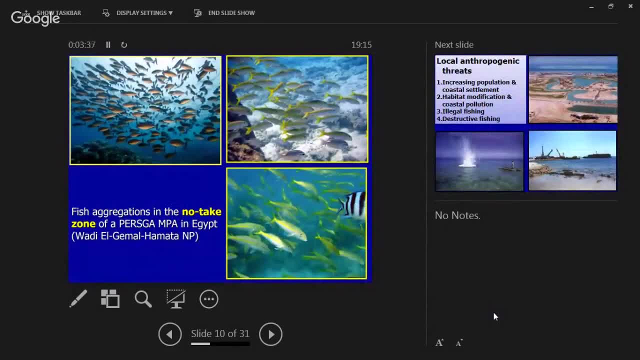 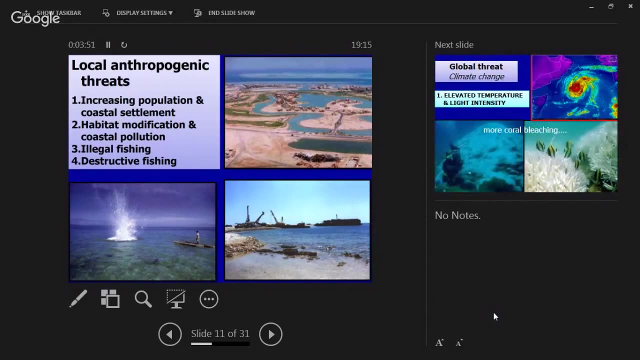 the mpa. that's the need uh. mba may reduce the poverty by creation of job opportunities in mba management and the tourism. but mba's faced many anthropogenic and the natural impacts like increasing population and the coastal settlement, habitat modification and coastal pollution, illegal fishing and destructing fishing. 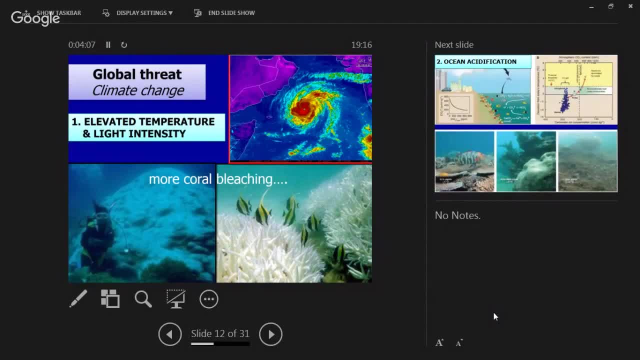 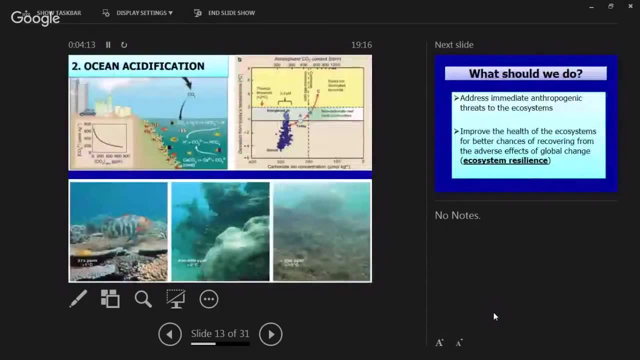 while global threats like climate change, the elevated temperature and the light intensity may lead to mass bleaching of coral reef, and this ocean acidification may destruct all calcareous ecosystem. like reef and the mollusks, all species that have external calcium carbonate gluten may be destroyed by increasing the ocean acidification. 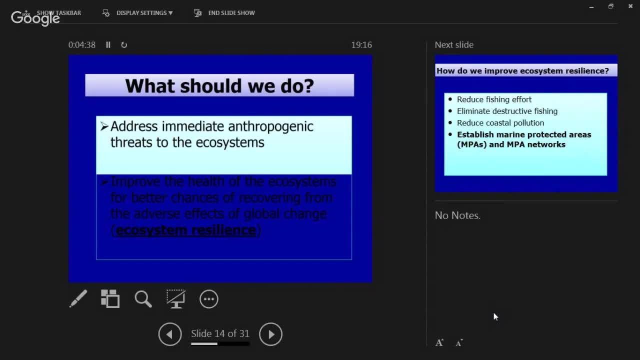 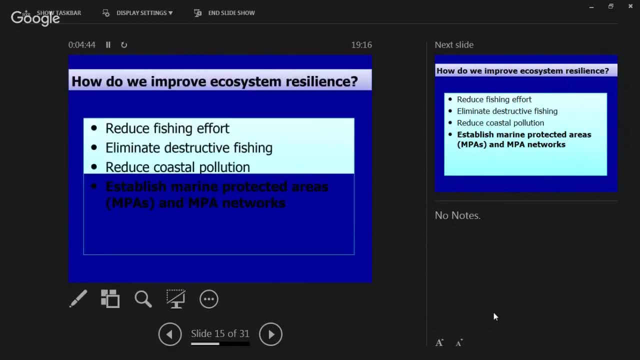 what should we do is address the immediate anthropogenic threat to the ecosystem or increasing try to increase the resilience of this ecosystem and improve the ecosystem resilience by reducing efficient effort, eliminate destructive fishing and reduce coastal pollution and establishment a resilient mba's network. so persica member state signed on a protocol for the conservation of. 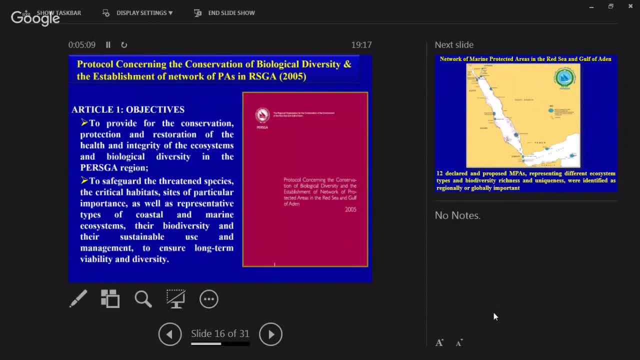 biodiversity and establishment mba network, along with the sea and gulf aden. the objective of this protocol is to provide for the conservation and protection and restoration of the health and the creativity of the ecosystems and to safeguard the species, critical habitat type of particular importance and all ecosystems, along with 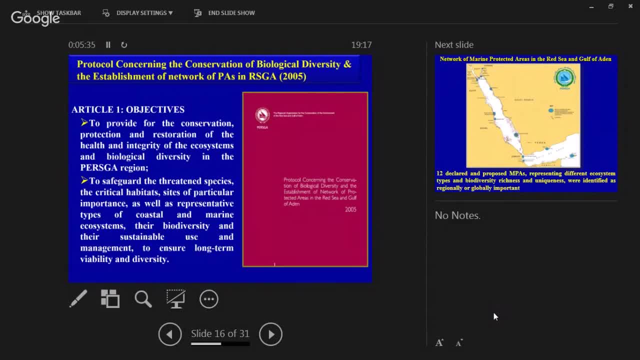 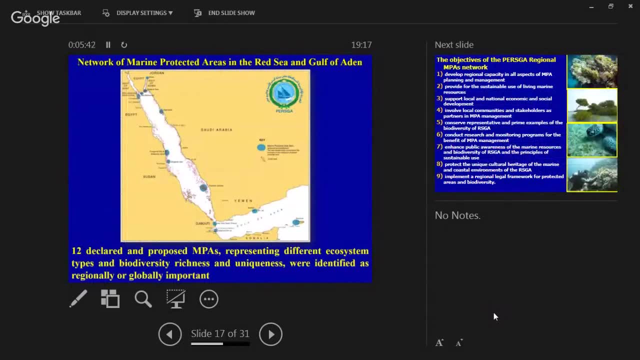 the red sea and the gulf. after signing of this protocol, uh 12 mbas declared, along with the red sea and gulf aden, and they represent all the ecosystem and the fragile system and the species occurred inside this persica mba's network. the objectives of this regional network. 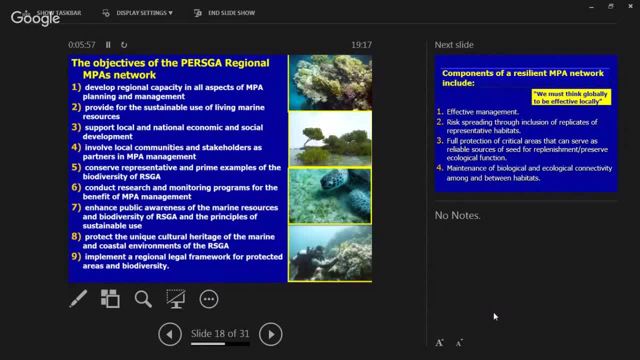 is to develop regional capacity. provide sustainable use of living marine resources. support local and the national economic and the social development involving local communities and the stockholders as a partner in bas management to their representative and the private example of ecosystem conduct, research and monitoring. enhance public awareness for the 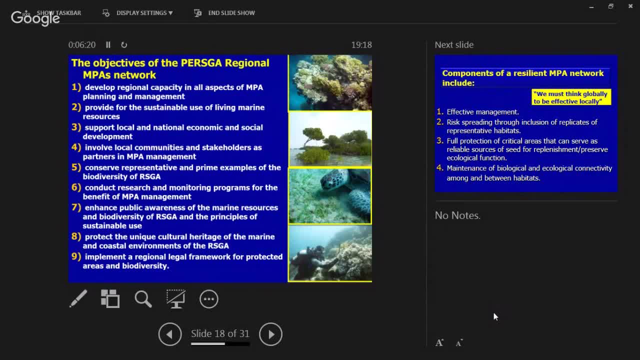 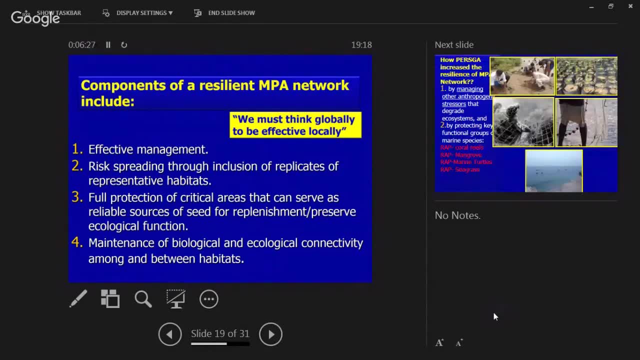 marine resources, protect the new cultural heritage, along with the ritz and gulf aden, and implement original legal framework, the for to create a resilient mba network, it must contain effective management. so persica annually evaluate the management effectiveness of all mbas, along with the inside the network. 12. 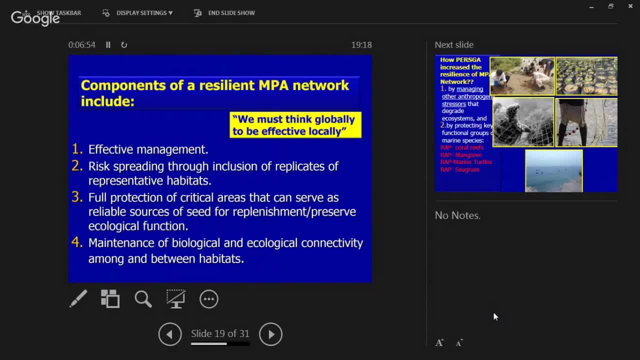 mbas evaluated for according to management effectiveness annually, and also the resilient mbs must contain how able to risk breeding through inclusion of replicates. so all fragile and decay habitat, specifically protected areas, are left neglected and coated with the current stereotype of wild and polluted species. the resolution of a branch of species. 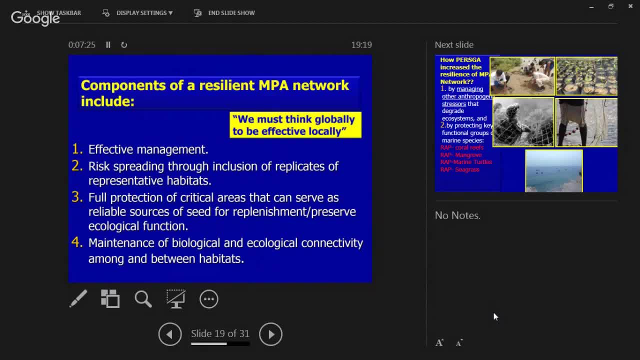 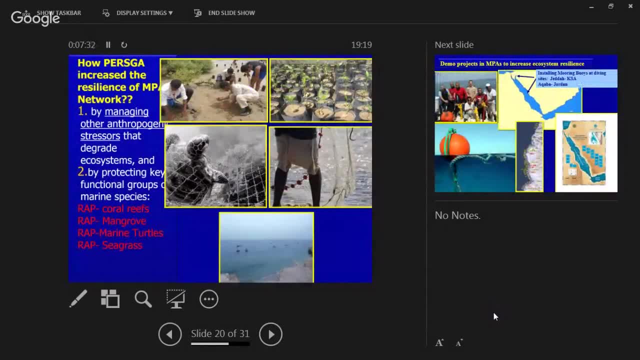 is identical to the population of a species. so we are thinking about how do we lead this community well in this area and we continue to work on this. so, as you see here, our number of species in a day is approximately 348 of. the population is about 30 percent of the population. 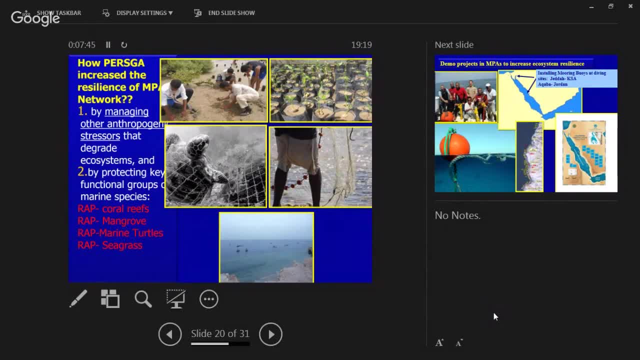 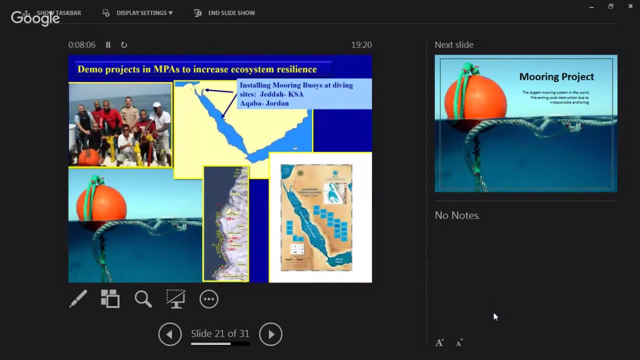 uh function group marine habitat. so we have a regional action plan for coral reef, for mangroves, for sea grasses, for dogong and the marine turtles. oh and this original plan based on a national action plan in all bershka region also try to raise the resilience of coral reef. so we 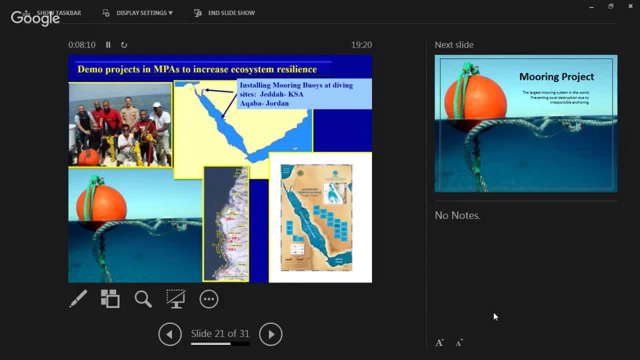 install mooring boys for the protection of the submerged reef from from anchoring of ships. we install about 50 mooring boys in the coast of jeddah in sudia arabia and about 22 mooring boys in the aqaba. on the other hand, the egyptian side installed the largest mooring system. 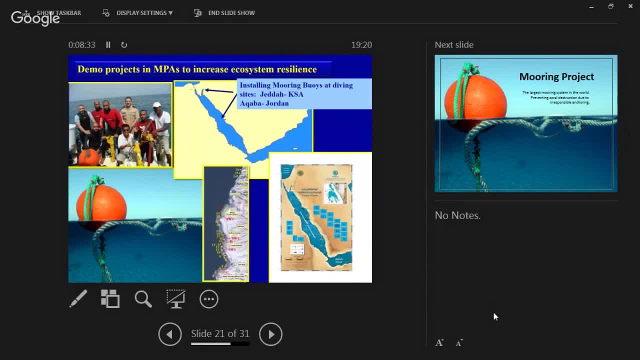 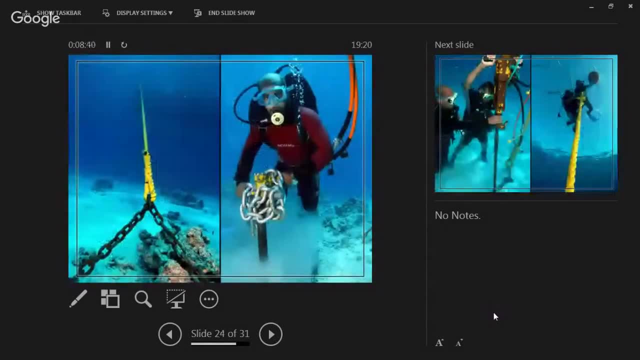 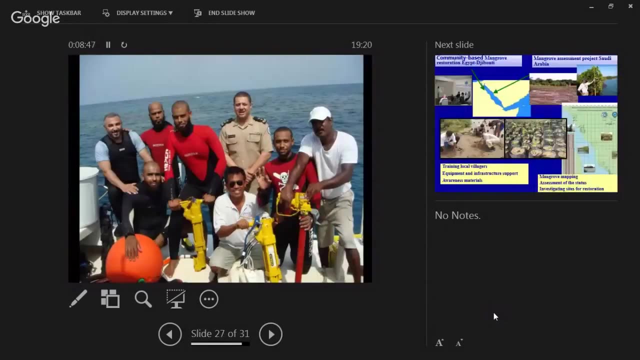 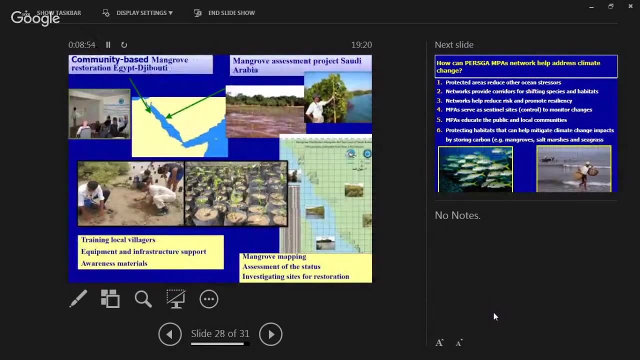 in the world more than 1 000 mooring boys along the egyptian submersion reef. this mooring restoration try to protect the coral reef from the destructive activities by divers and snorkels. also we try to restore some ecosystem- crystal ecosystem like mangrove, and transplant and 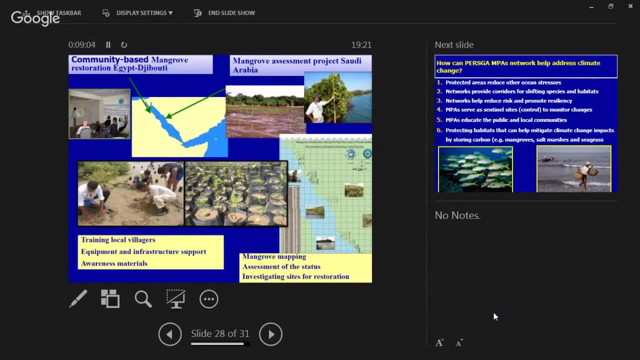 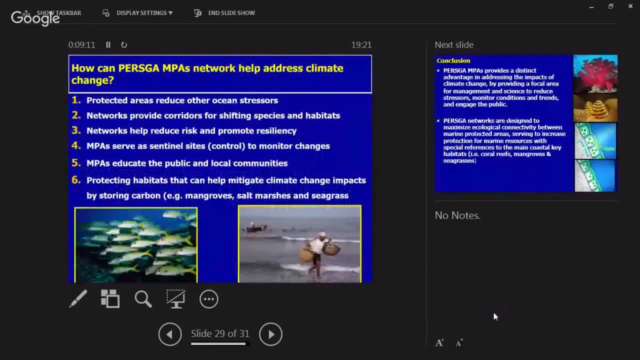 restore mangrove- degraded mangrove in djibouti and egypt and assessment all the mangrove with the uh. sweden arabia pre-sequence: one minute at least. climate change by in protected areas reduce other ocean resources. network will provide corridors for shifting species and the habitat. mba served as a control site for monitoring. 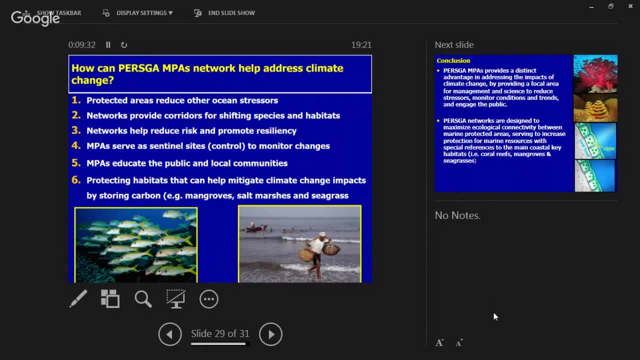 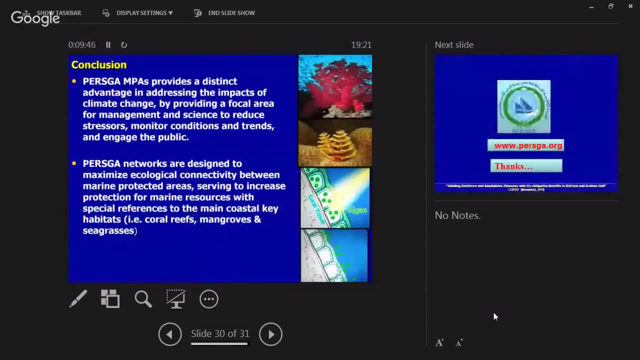 change mba educate and the public, and educate the public and local communities, protecting the habitat that can help mitigate climate change effect by storing carbon, like mangrove, seagrass and salt marshes. finally, iris can be able to provide a distinct advantage in addressing the impact of climate. 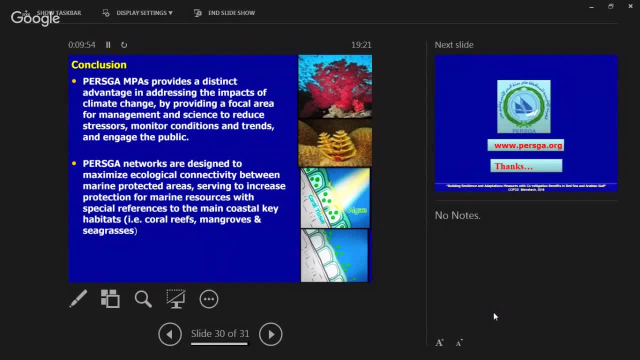 change by providing a focal area for management and defies, to reduce stressors, military condition and the dreams- and engage the public in the process of the management of the air. and also the starύ are designed to maximize the political connectivity between marine protected areas, serving to increase the protection of marine resources, with special references. 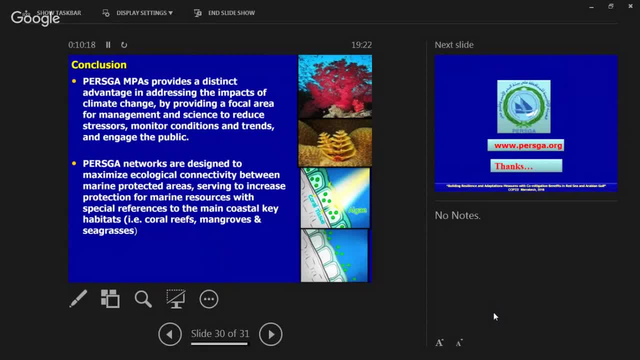 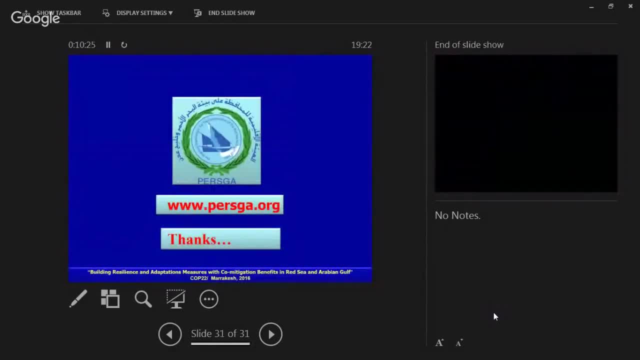 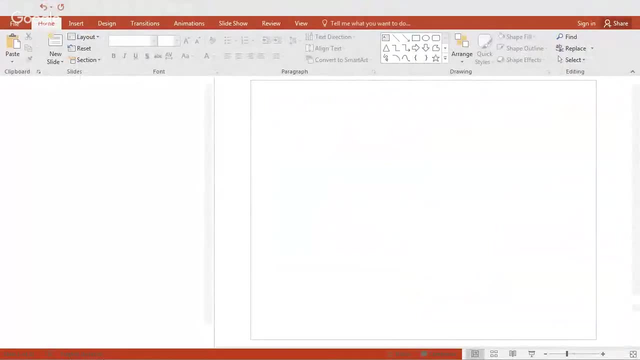 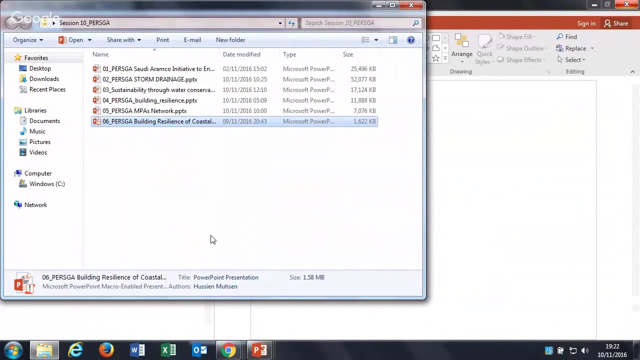 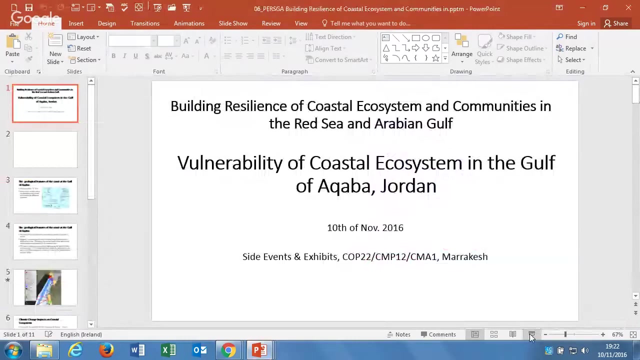 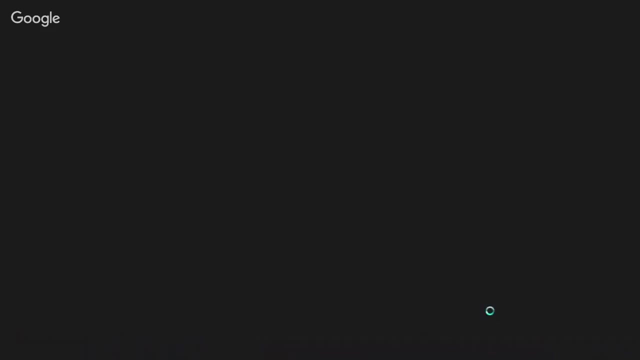 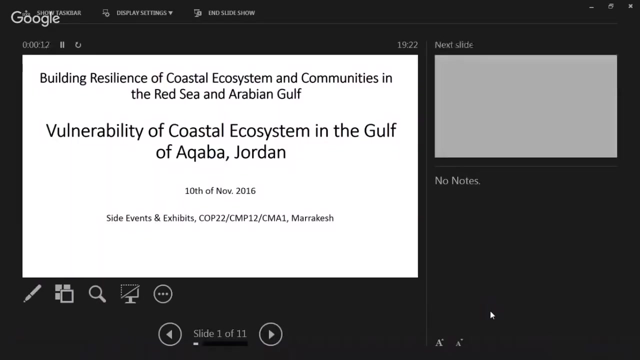 to the main coastal case: beaches, coral reef, mangrove and sea grass. thank you. presentation for this session. uh, it will be demonstrated by mr hussein. mr hussein has a master degree in marine science and environmental science management from the university of jordan. he worked with the royal 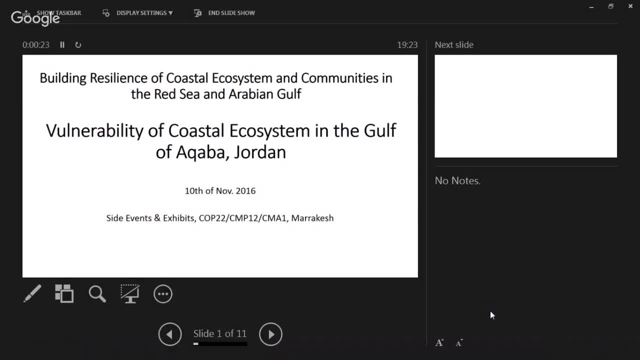 society of conservation and nature for seven years and he's also working on introducing element climate, climate proofing and biodiversity conservation with the protected area in a special conservation area. recently, he worked with the international expert in producing the strategy for climate change adaptation and implementing for two pilot projects for biodiversity. 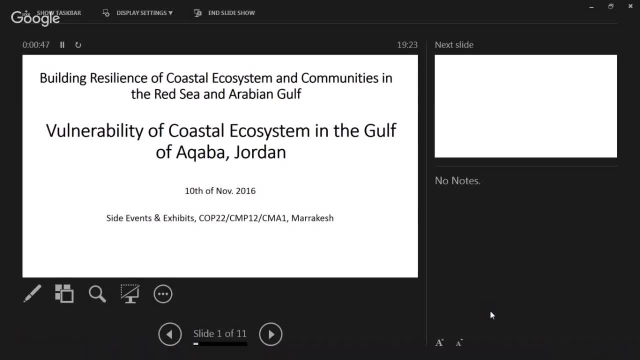 adaptation with the climate change. so good evening. uh, i think you're a little bit tired at the end of the day, and i'm the last speaker and i will promise you that i'll not be long. i'll be short and direct to the point, so cheer up. so. 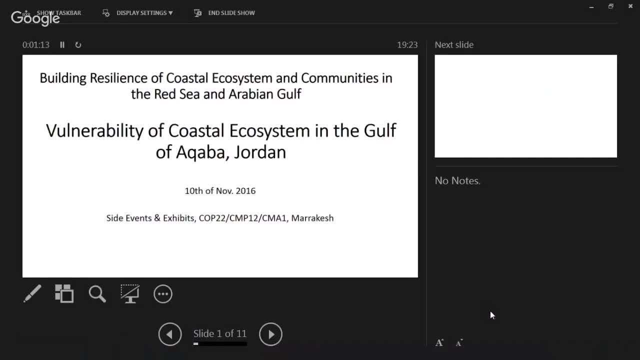 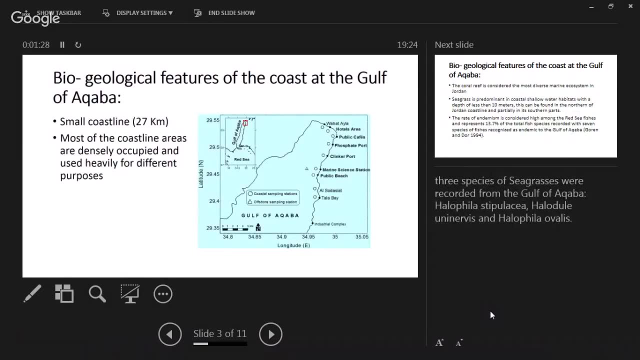 so what i'm going to present today is a case study of the efforts done by persiga partners in the region, and especially in jordan. so what you're going to see now is the activities that recently had been done in aqaba. so first of all, i will give you an exam and a brief about the aqaba itself. so 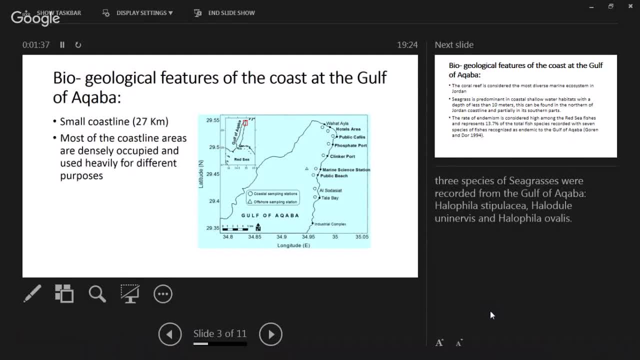 aqaba has a small coastline, it's almost only 27 kilometers, so a lot of things happening there as well. so most of the coastline areas are densely occupied, as you can imagine, and so far no, uh for different purposes, uh, fisheries and tourism sites and hotels, and you can see some examples on the. 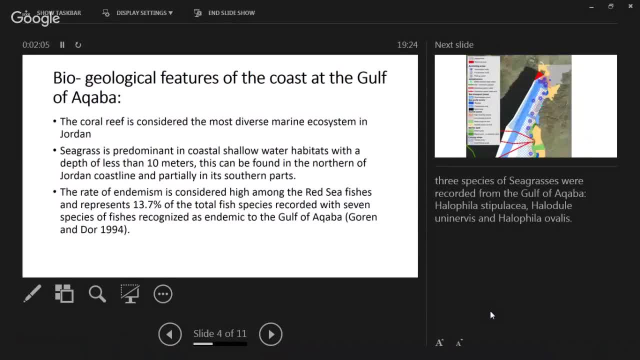 picture here. the coral reef is considered the most diverse marine ecosystem in jordan because the coral reefs itself and it's the most diverse marine system. seagrasses also is predominant in coastal shallow waters, uh, with depths of 10 meters. so seagrasses play major role in mitigation. as you know, they are the most. 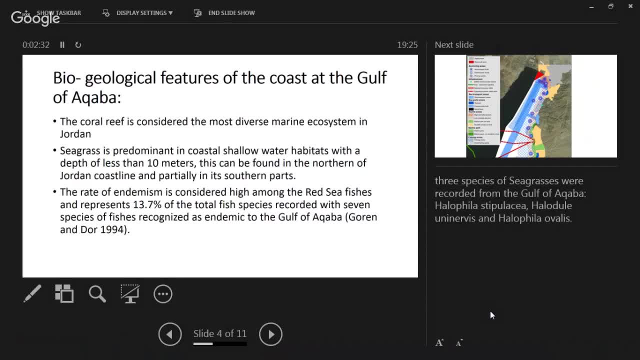 existing thinks for who whom thinks the carbon and the water? the rate of endemism is very high among very red sea fish fish and represents three, 13, almost 14 percent of total species. so it's a lot of fish and it's a lot of heart. 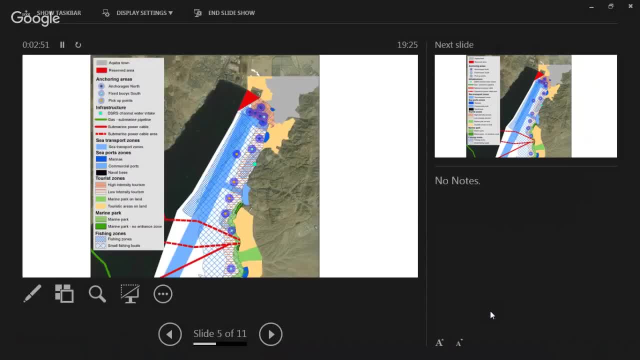 which is high. so this is to brief you about the activities happening in the Gulf of Aqaba. you can see in the dark grey is the city of Aqaba and this is the shoreline. so this is the activities happening. so you can see that there's marine parks in the area and there's many places for fishing around. 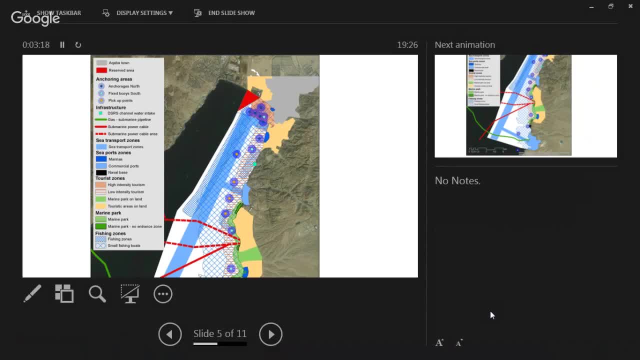 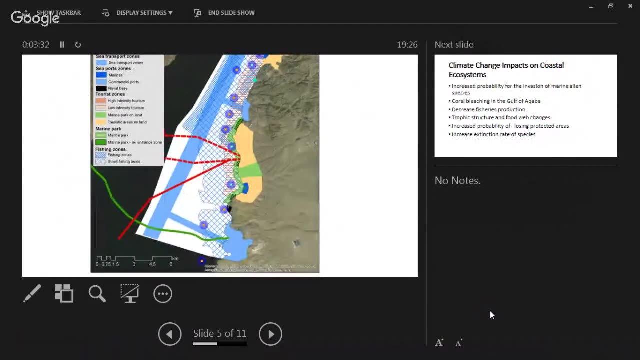 the place. so it's as I told you before. it's condensed and a lot of activities happening and you can see there's some places for which is protected as well in different zoning. if you go to the south as well, there's the extension of the marine park, so you can see that it's a long, long area and it's a big area to. 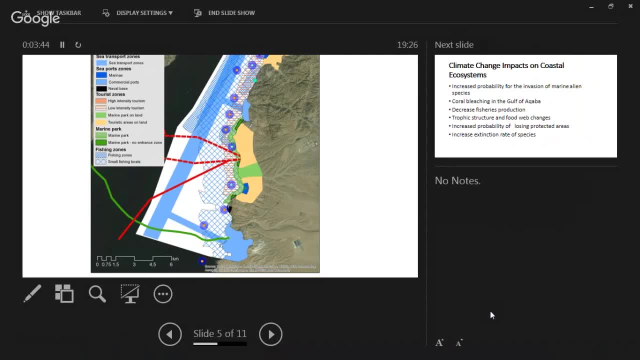 conservation speaking, but what I can uh focus on is that the many activities happening here is that is about restoration, and restoration is the tool that we are using in Aqaba to increase the resilience of the existence. we had the case that the port they located a. 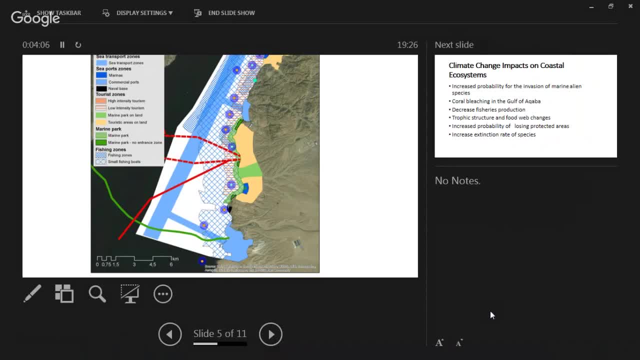 port in a very sensitive area for coral reefs. so the Aziza- that which is the Aqaba authority, that who is running the place- they decided to restore the area and they decided to restore the area and they decided to remove and relocate the corals- sensitive and endemic corals- to the to. 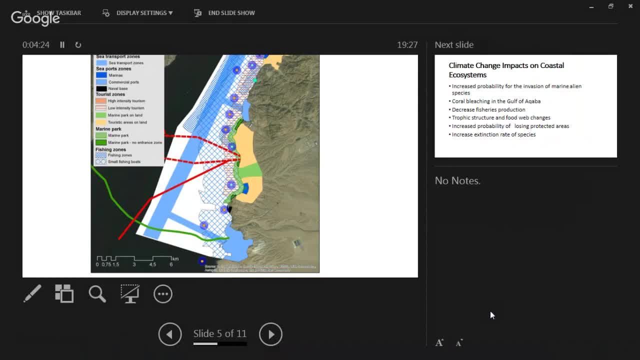 another area which is protected now, and they had a very successful experience in that, with the success rate of more than 90 percent of the coral reefs replanted were successful. that well, and that is what we need to build on. so what such the impacts of? of the coral reefs replanted were successful, that well, and that is what we need to build on. so what such the impacts of on such the impacts of on 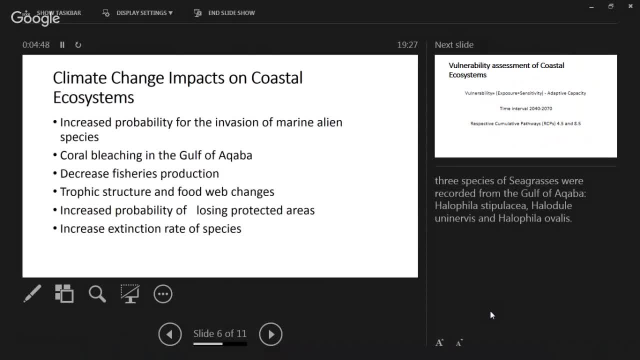 on such. the impacts of on such. the impacts of on such. the impacts of on coastal ecosystems in Aqaba can be summarized. coastal ecosystems in Aqaba can be summarized. coastal ecosystems in Aqaba can be summarized in the following: uh. according to a recent 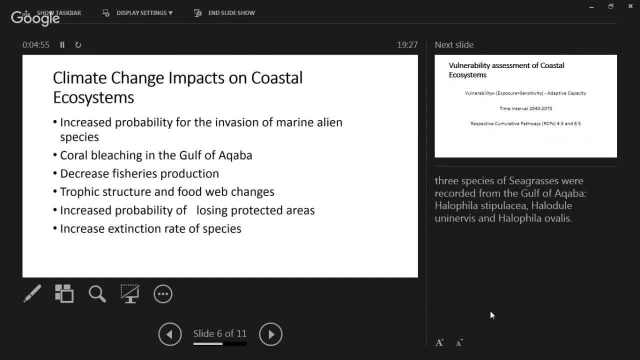 in the following uh according to a recent in the following uh according to a recent study in the third communication report. study in the third communication report. study in the third communication report of Jordan: uh increased probability of of Jordan. uh increased probability of of Jordan uh increased probability of invasion of marine Alliance alien species. 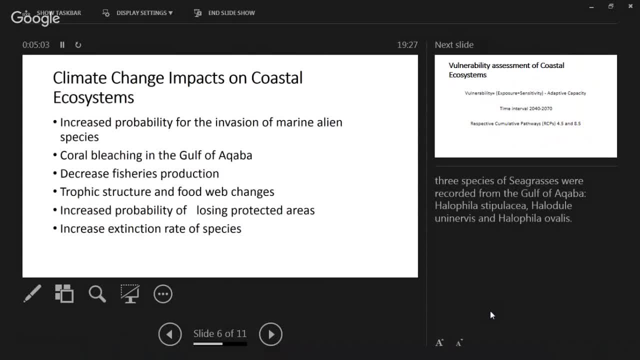 invasion of marine Alliance alien species. invasion of marine Alliance alien species. I'm sorry, a coral bleaching which is, I'm sorry, a coral bleaching which is, I'm sorry, a coral bleaching which is happening in such some cases decreases happening in such some cases, decreases. 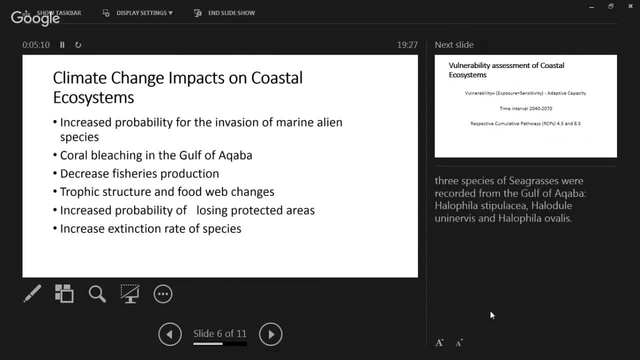 happening in such some cases decreases fisheries production, which is very fisheries production, which is very for local people, traffic structure and food web changes expected and starting to happening to happen. increased probability of losing protected areas that we are dealing with now because of changes of that I'm saying, I'm 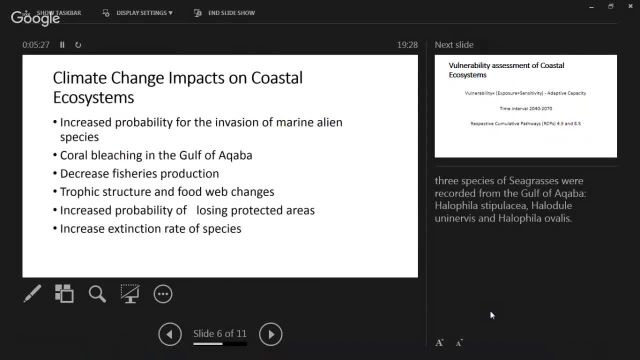 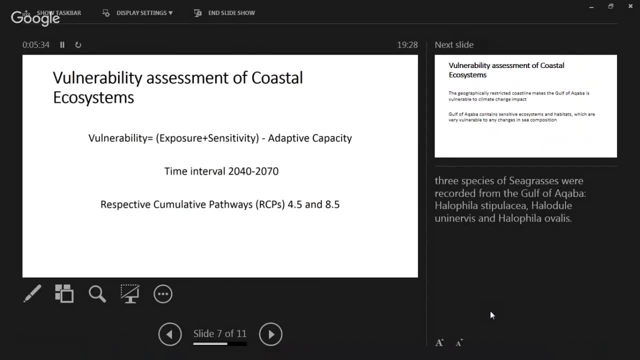 mentioning for increased extension rate of species. so what we did actually is the vulnerability assessment. it included three components, as you can see in the map and slide: the exposure and the sensitivity, composing the impacts and removing from that the adaptive capacity of this species or the system we use. the 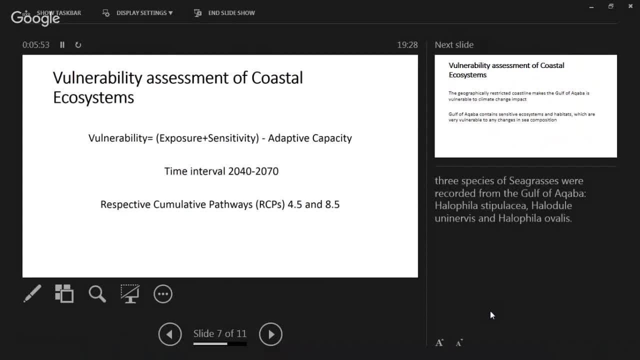 time interval of 2048 till 2070, using two emission emission scenarios: moderate, four point five RCPs and 0.5 the most, the worst case scenario. so the vulnerability. I will brief it into the results of the vulnerability. I'll brief it in two sentences only. the 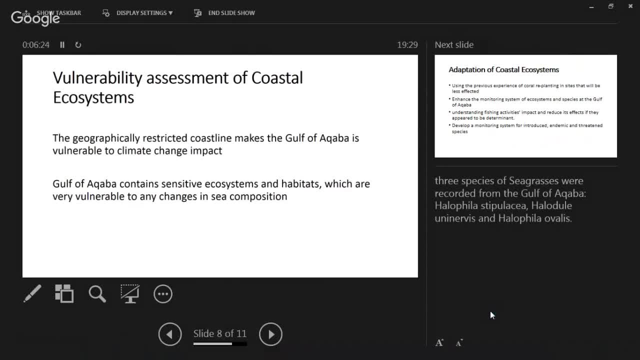 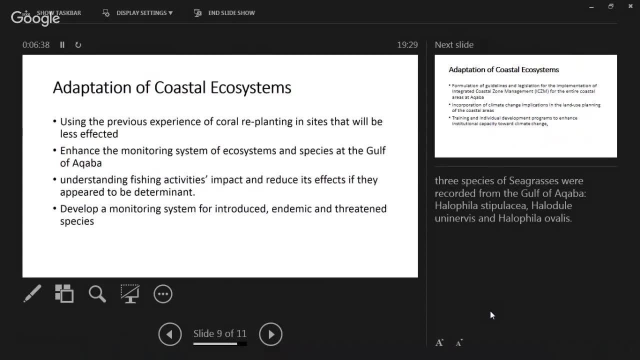 geographically restricted coastline makes the Gulf of Aqaba is vulnerable to climate change. in fact, this is the bottom line. the Gulf of Aqaba contains sensitive ecosystems and habitats which are very vulnerable to changes in the sea, in sea composition. for that we recommend the 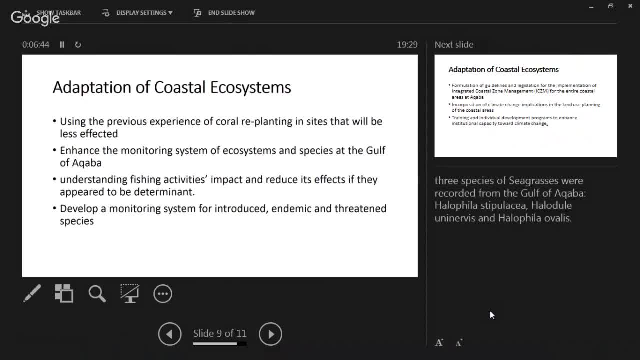 adaptation measures as follow: using the previous experience in coral replanting, as I said before, an insight that will be less affected so we can increase the resilience there. enhance the monitoring system of existing and species at the Gulf of Aqaba and, like the previous speakers, told us some experiences. 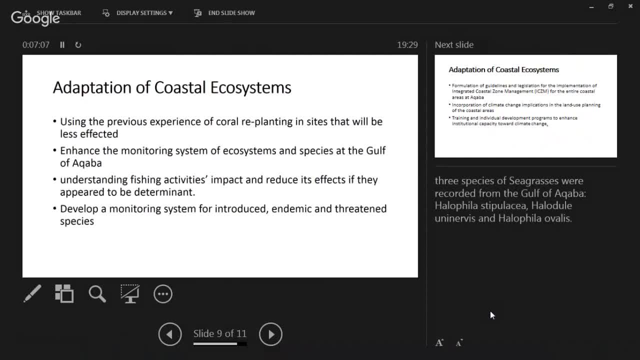 happening in Aqaba by having more devices there and which is starting happening to happen, understanding fishing activities impact and reduce its effect. by and by that, we remove the anthropogenic people, develop monitoring system for introduced and never to introduce the endemic and threatened species, as happened in Saudi. 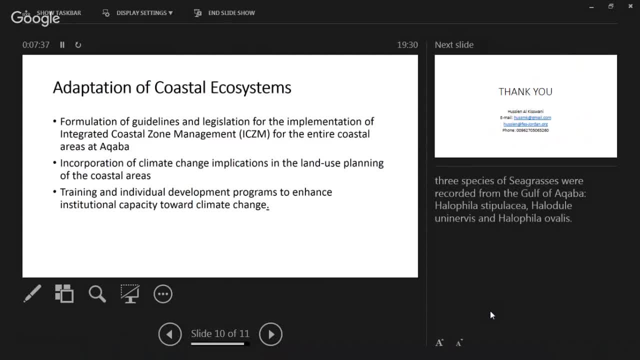 Arabia, example in the beginning, the first presentation. formulation of guidelines and legislations for implementation of integrated course management for the entire coastal area at a cover. incorporation of climate change impact implications- sorry on- in the land use planning of the coastal areas and, last but not least, training and individual development. 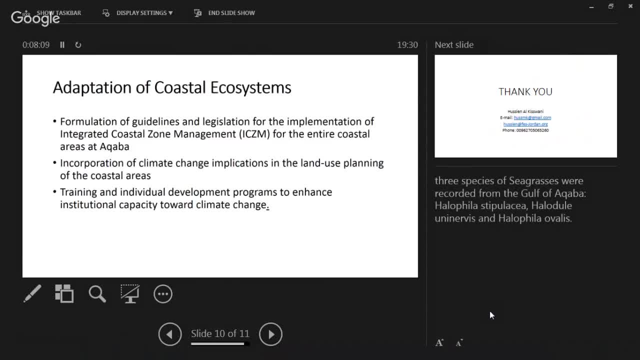 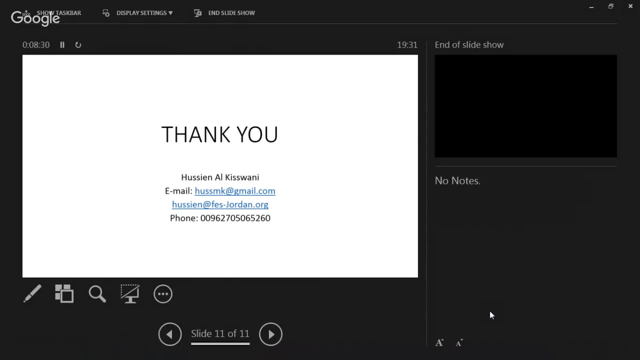 because we believe that human are the most valuable resource in Jordan. so we always focused on capacity building and this is the most important thing- to enhance the social capacity toward climate change. and these are everything you think. now I leave the floor for you, ladies and gentlemen, to ask the question. 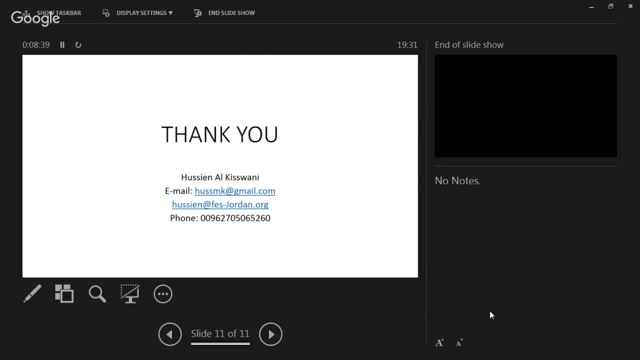 that you want. all our speaker are here now. we have about 30 minutes for all of them to answer your questions towards yours, so I have a question for engineering. This is quite unusual, partner, but actually it's the first time that wouldn't you be able to export any form of? 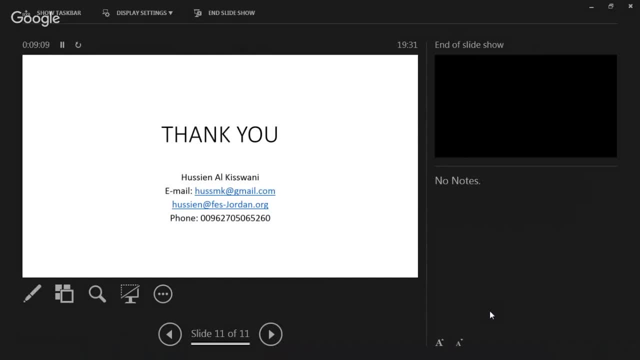 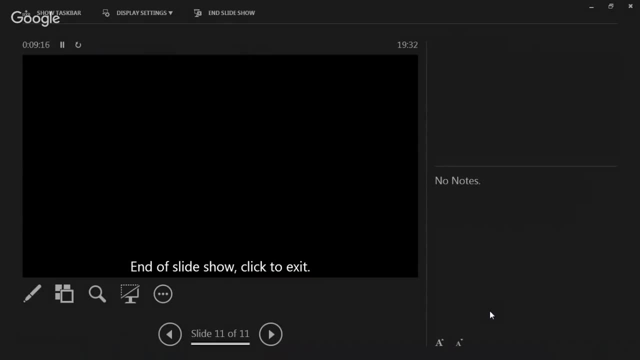 data from this is water. is the next step at least affected by climate change? け Hi, So there was a question. K, director of engineering, I was wondering- sobre- behaviours, but in focus by a lot of the members earlier in our lesson- to see how you think about your own stakeholders and to set your own goals in the future. as softhe yolks, the one thing that 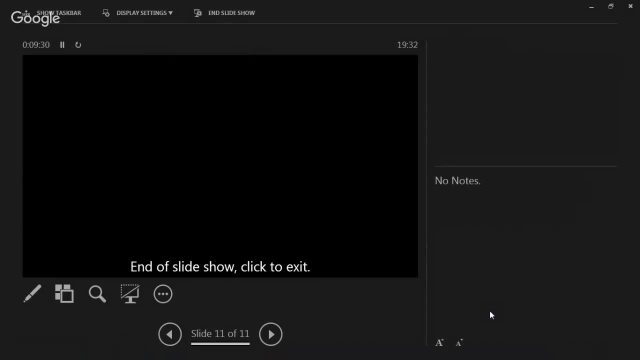 this line, the primary one, the primary line from north to south, and that's it. we just give some access to new building, like for the mondial 2022, the stadium. they have already access, but not the rest. so if I will say in percent, I will. 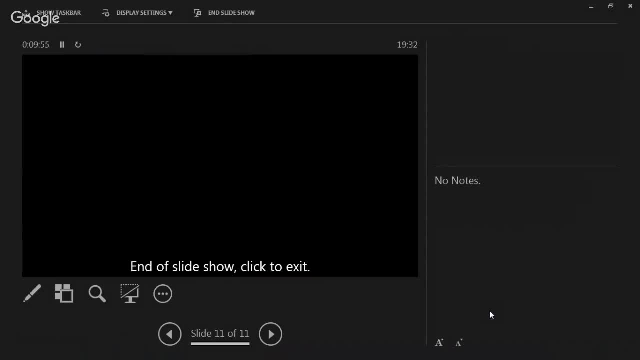 say two percent, three percent, not more than that, because we just start. but hopefully in two years we will complete TSE in all exists and new building. thank you for all the presentation which you have. it is very good and I'm very interested in your experience. but actually we could, we. 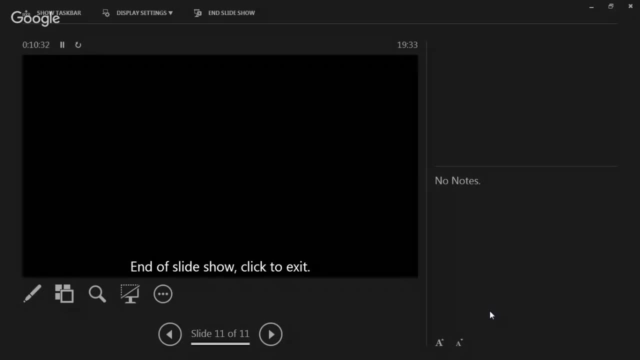 couldn't get it. we didn't know what is the methodology and what is the abbreviation which you have said, for example, this TSE. what TSE, please? after we use the water, we treat it. we don't just put it away, we treat it and we put it back for irrigation. 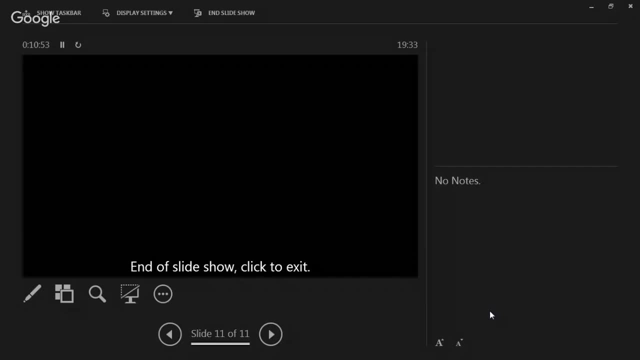 and HVoku AC system. you talked about water conservation are also on the energy for the gas and second electricity and in residential areas and in the industrial areas, but we didn't tell us about how. okay, I will talk about cattle and the Gulf country, the water. we use energy not just for the destination only, also for 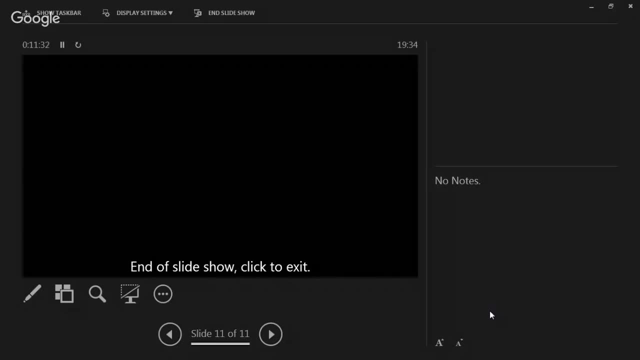 pumping. this is stage 2. stage 3, the user itself in our existing building. the fourth thing is the TSE, the treatment water. we treatment the water, so we will use it again, not not, for example, for direct for a human or something. we can use it for HVAC. 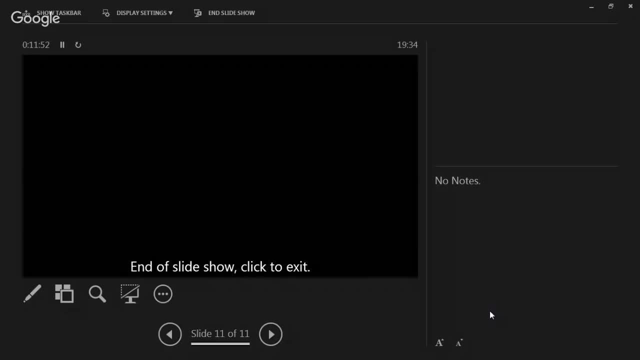 C system and irrigation system and, by the way, the irrigation system in Qatar is 25% of the total consumption in the country. so we are, when we will complete the, we will save 25% of water just to treat it again. I hope this will be clear. 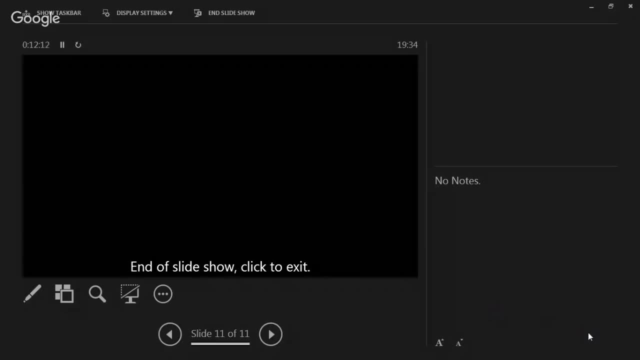 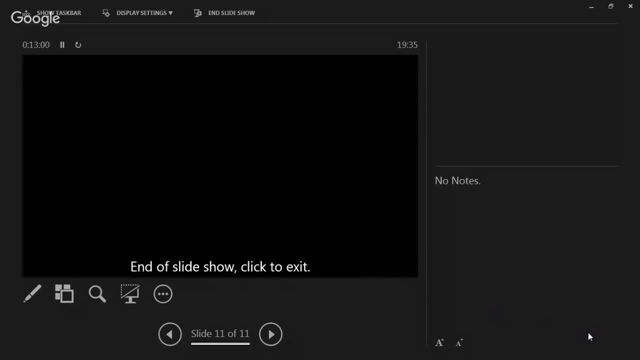 what about the low one? i think at least you have to use the rcps to give you a picture from low to high. thank you, okay. uh, yes, you're right, but uh, what happened that we used the moderate? and uh, because what we realized that we looking to the future, we, we will not be sure that the, the low. 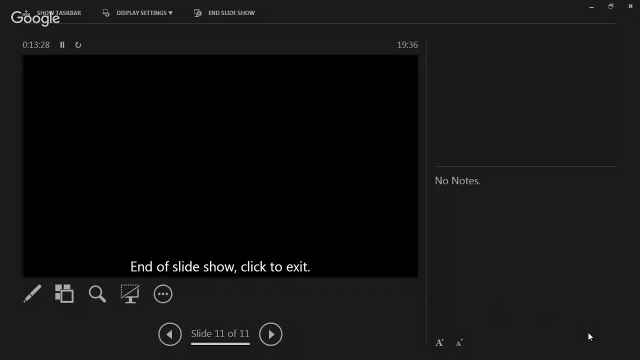 emission scenario will be the fact. looking at the scenarios happening now and, uh, what we call it the business as usual, we are going to the highest scenario. so, after this long discussions- this is a discussion that happened in jordan for- with the experts and the team that they worked with us- 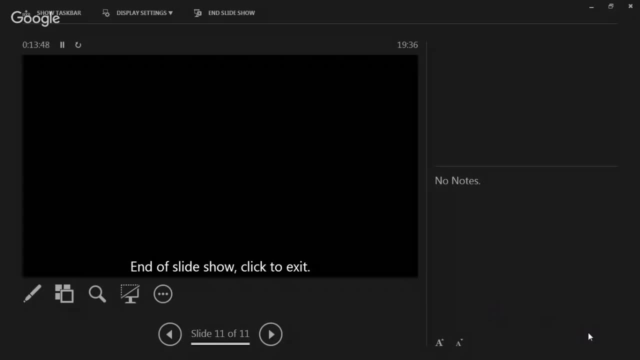 it had a very long discussion and you are right. some people believe that we should look at the lowest and highest, and this is the usual thing. but what we would? we thought about it because, because the lowest is not really reasonable anymore, to put it like this. so we thought that we should study the 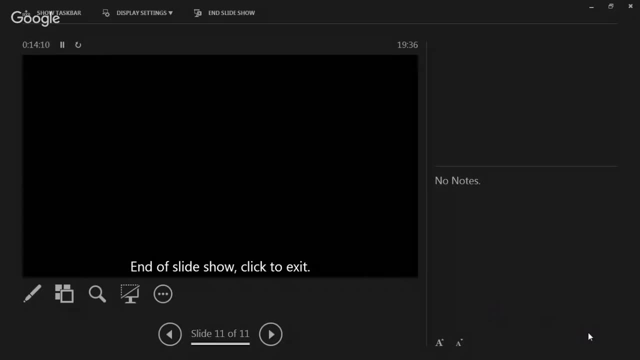 moderate and this is the only explanation. so for this reason, the low alone and the mid clear is the n here. so we just, we just, Nazir, we are historically had a very high popped, largely lowYeah. really lose aeronautical. what we nerves that breakfast at $60 a아아. 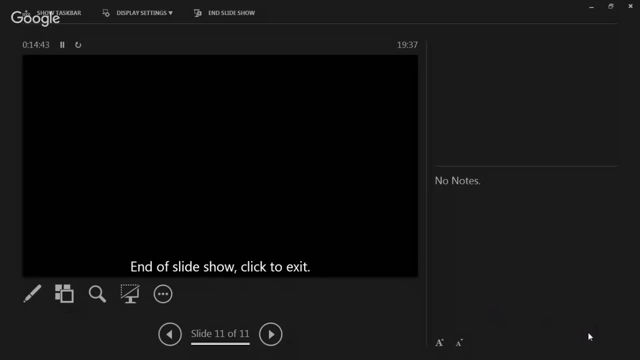 my final question is just: uh, when you speak about biodiversity in one level the population is in. local population is implicated and contributes to the sustainability of the resources. answers local population. in different countries, Are they implicated or the government only do what is done or the population local is not? 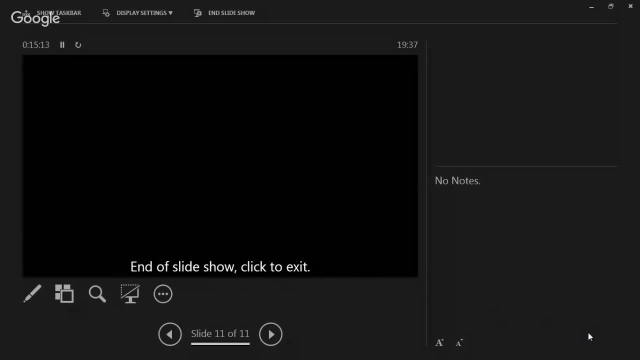 The question was about pollution, population, Involvement of population, involvement of the population, local population, Involvement of population, yes, Even fisheries and fishers and others, As my colleague mentioned, and also I mentioned that we have strong collaboration. 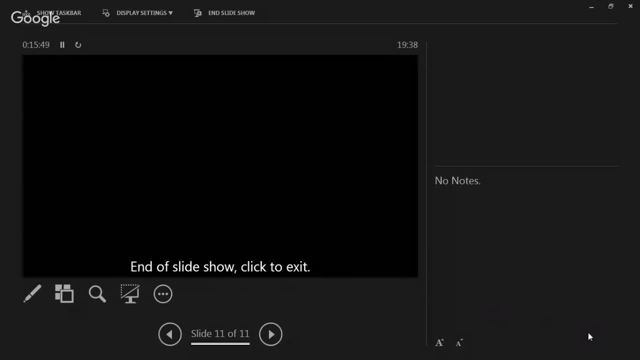 with local communities, especially in protected areas. So in the protected areas the local community are part of the management plan. They are considered the management plan of the MBS. They are participating in conservation activities, restoration activities and also in monitoring and surveillance of the protected areas. 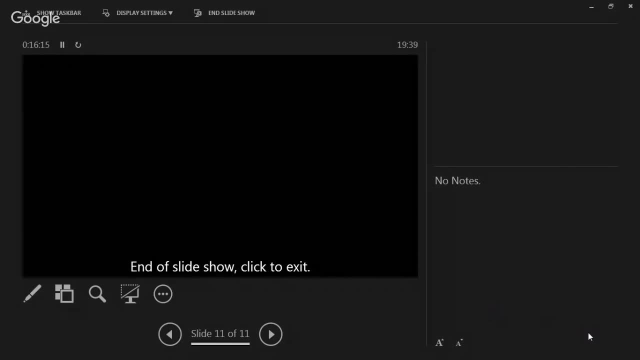 They are also the fishery program, also have direct communications and direct collaboration or involvement of local fishermen And they are also receiving training. We have special programs for community training And also in the awareness education We have the awareness, regional awareness. 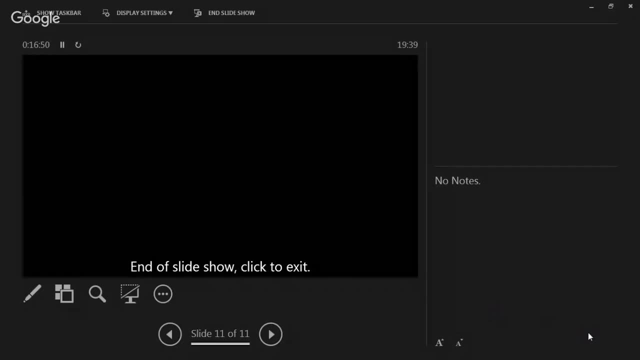 environmental education strategy, which involve schools in coastal cities and also media and other sectors of the local community. I have another question for from the ADA. The way I understand Riyadh is that, as you described the, there are two wadis. 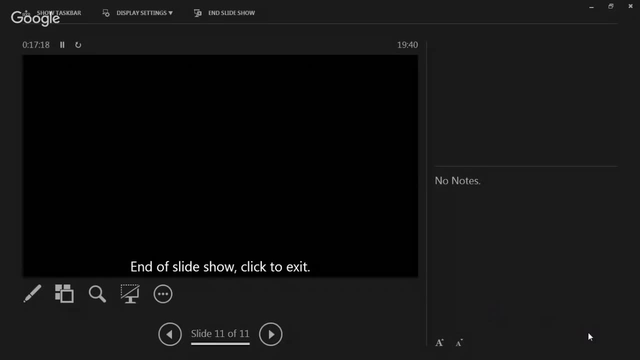 the Hanifa Wadi and the Sulayh Wadi. The Sulayh, the Hanifa Wadi is quite, quite empty. There's no overdevelopment on the wadi. It was easy to redevelop and restore it as a. 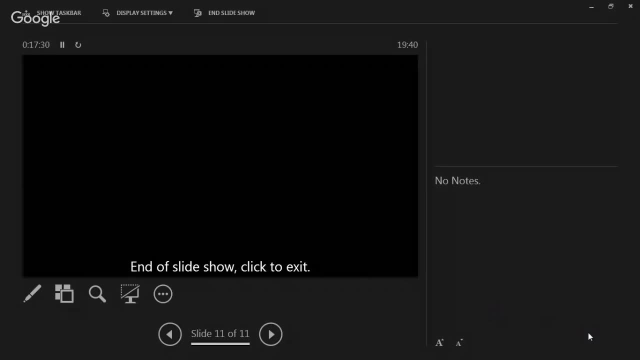 as a water system, While Sulayh seems to be overdeveloped And there's also some buildings over it. So how do you, how do you plan to go about managing that? You spoke about suds, So I couldn't imagine really how you're going to do this. 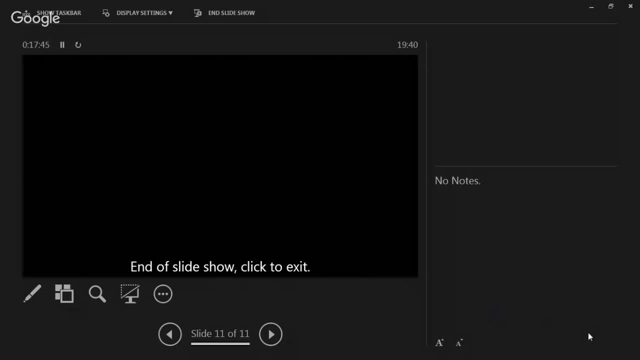 With the wadi partially covered with buildings. Okay, That's a good point, because the project is live. now, Wadi Sulayh is another project which is the, let's say, the second arm for the city, And this is with Riyadh municipality. 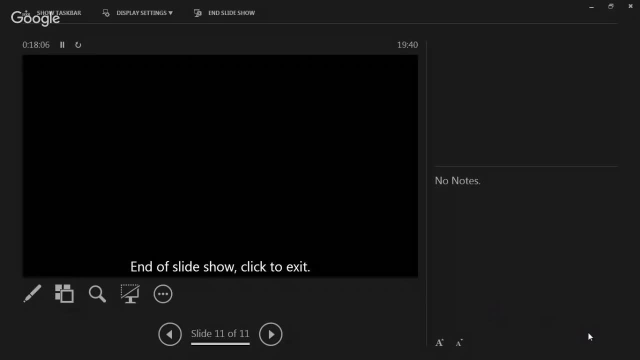 They are developing the wadi, as what you said. Wadi Hanifa is very well defined wadi, since it's deep, But wadi Sulayh is flat, But still we have the main drainage channel for the wadi And it has been identified. 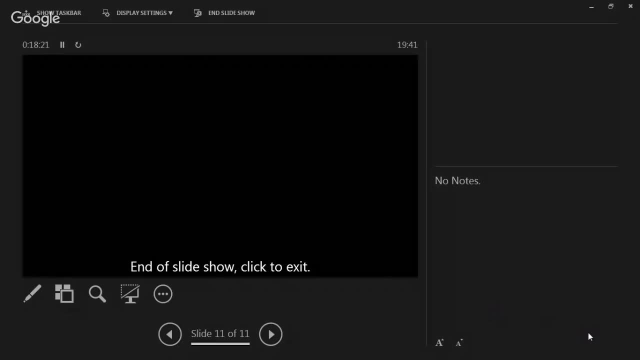 Also there is some difficulties to solve it, but it is easy to divert in such cases or just to go through main infrastructures If there are using box, box or others. Thank you very much. Thank you, Thank you, Thank you. 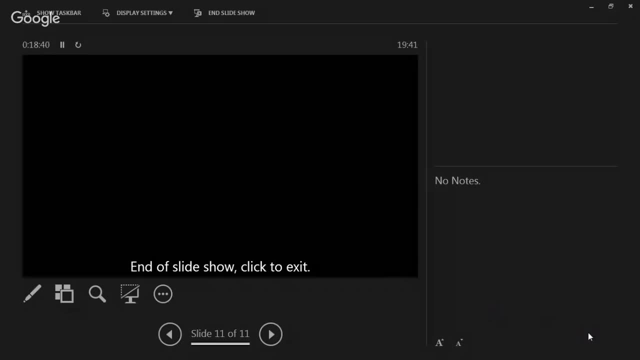 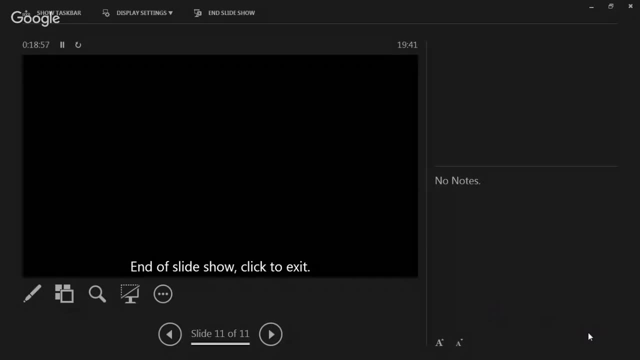 one of the highest per capita carbon and water footprint in the world. So is there any other policy that you're considering or like so, removal or public campaign, awareness campaigns that you know about? okay, sir she. first of all, i just want to make clear what is the sheet. the sheet is a department. 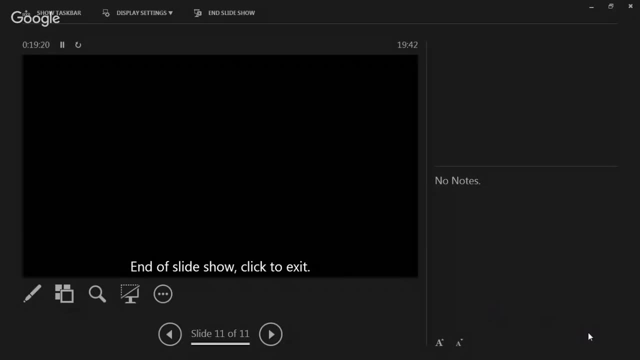 it's a program, but we are sponsored directly from his highness amir of qatar. we have authority to tell each ministry to what to do to conserve water or electricity. about qatar, it's actually doha, not qatar, which is have the highest, because more than 90 percent of 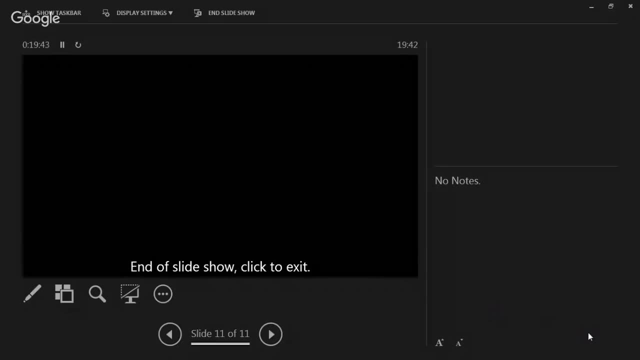 the people. they are in doha itself and it's a small area. so we are talking about per capital in in the kilometer. this is the only reason, but if and we have a dust most of the of the days in the year and this is also effect, so it's 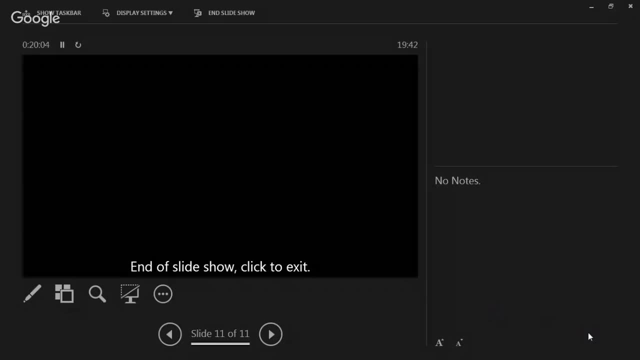 not the only reason, but if we have a dust most of the of the days in the year- and this is also effect, so it's not about really we are consume a lot because we don't have a lot of manufacture in industrial in doha to to make this issue happen. we don't have a diesel. 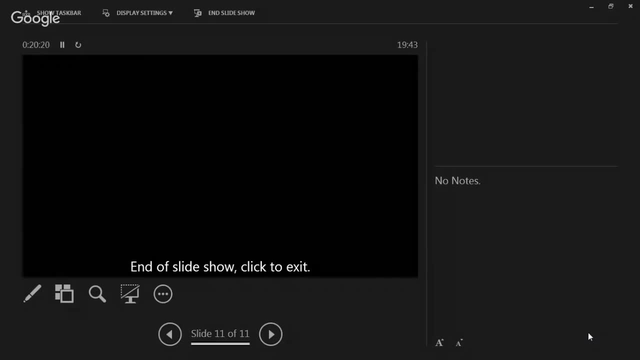 just like one percent of the big trucks, they have a diesel. so the reason is because they all in qatar, in doha and it's small area, less than five percent of the total uh size, the total uh space in qatar and, as i mentioned, we have dust most of the days in the 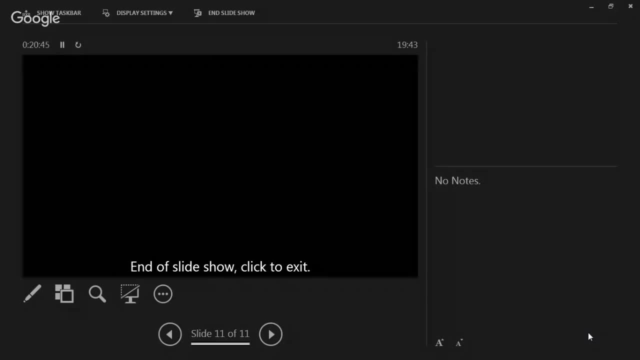 year. this is the only reason. yes, and actually there's um. we have another uh company. they- i hear from the environment ministry- they brought some company from um- i i forget from where exactly- and they make their study and they say there is very big gap between the reality number and what's published. so it's not really. we have this issue. 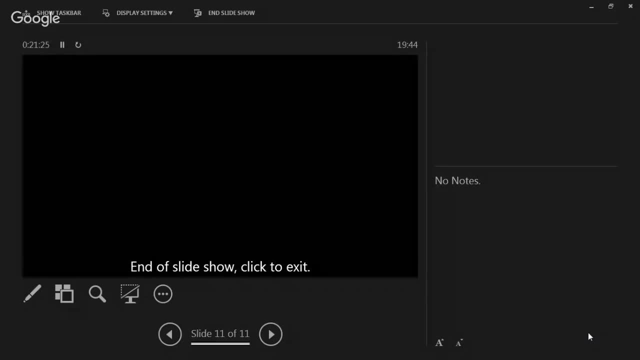 is it possible to make a comment or is it just if you have a comment you can. you can discuss it to the speaker after the session. if you have a question directly, may i come back again. sorry, may i ask a question? of course, thank you very much. 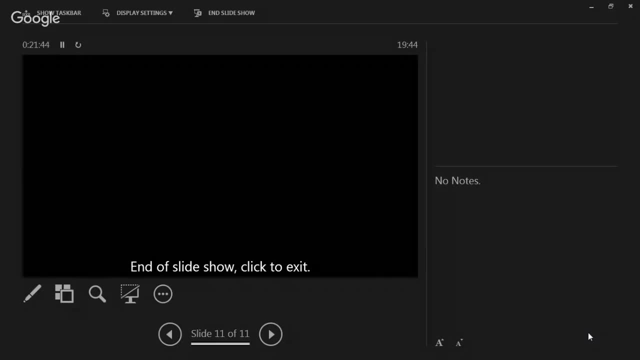 this goes to bersiga actually. uh, they have studies and on ground work. i must ask about the sustainability and replication of this, this work. is there any any measures taken for sustainability for this uh uh series or this diving or replicating this in other area? thank you for the question. 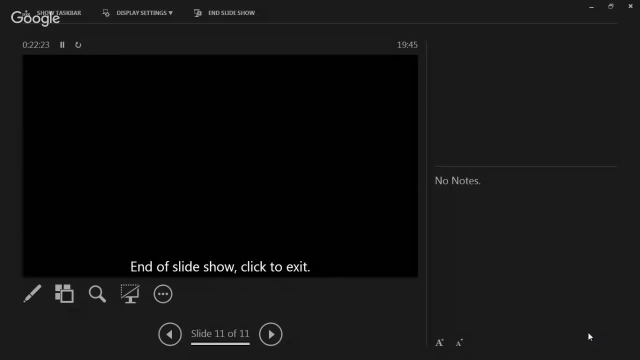 sustainability, actually the, the, especially for this community program, we have usually sustainability strategy and for each project, we have sustainability strategy to sustain the, uh, the, the, the project activities and this strategy, uh, i'll give you some examples. we, we make it in in consultation with, with, with the stakeholders. 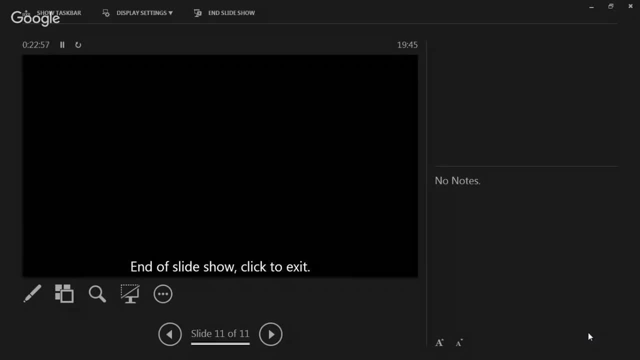 themselves, like now in we have uh. there are uh sub projects for some community-based projects in donggunab marine protected area and also in in egypt protected area. we have some projects developed for generating incomes from non-extractive use of marine resources- mainly non-extractive use of marine resources, mainly 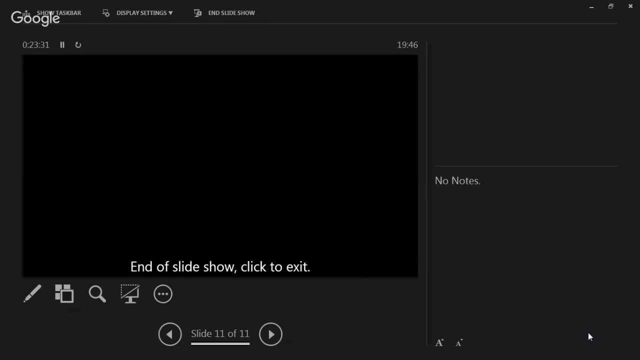 ecotourism, enhancement of ecotourism, involving fishermen in ecotourism, and also sustainable fishery based on, especially for some commercial species, based on management and of spawning, spawning grounds and spawning populations. The design of this project has considered sustainability. 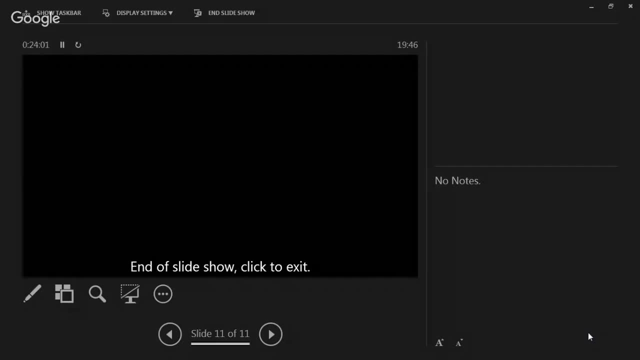 and they have sustainability plan, for this Sustainability plan was developed in consultation with, which involve, which include also all the, even the funding, financial aspects and this training for the local community themselves- That's the process- will be community driving in the future. 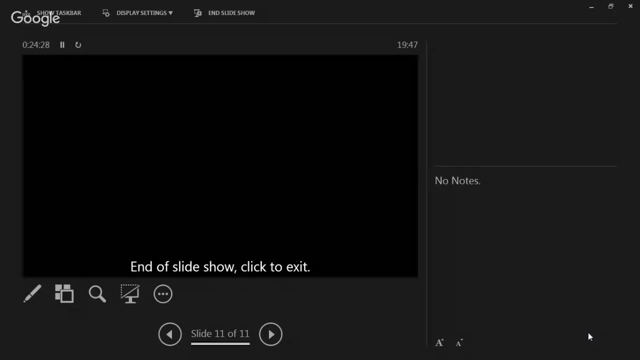 Like this ecotourism project. we have, for example, class boat tools for villagers and they have the sustainability of the business. The community received training and they could also establish fund to sustain the business And there was also screening, a lot of screening, of the tools and options. 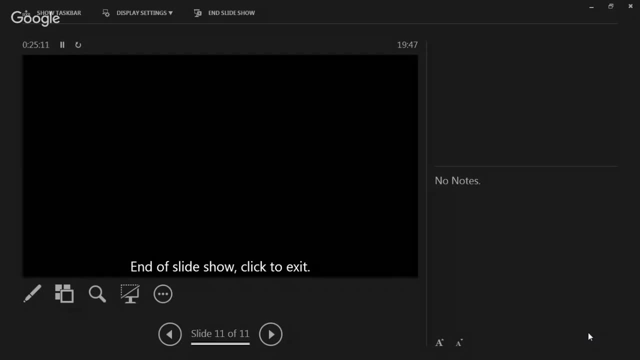 that they can follow or they can adopt in to sustain the activity And also involving the local community in the management of protected areas. They are involved in the board for the management and they're involved also in the in the monitoring and surveillance of the protected areas. 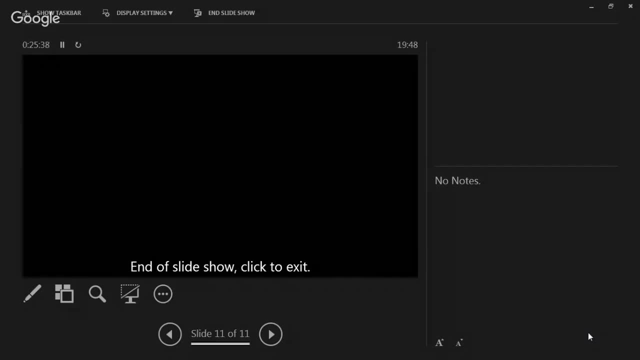 And they are also involved in the fishery monitoring. So there are a lot of aspects that we consider in this small on-ground sub-projects to sustain the activities by the community themselves. Another example: in Djibouti we have a project of mangrove. 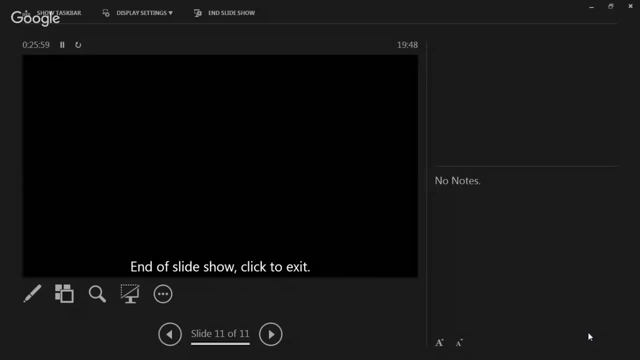 or mangrove, or mangrove restoration, community-based, And now this project is the project. the restoration activities are continuing. now It is getting sustainable And this restored area is is now a source of and source of tree of. 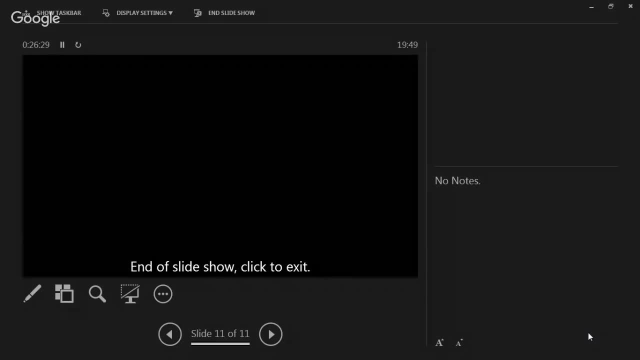 source of of uh in exporting mangroves to other areas, So the process is is sustainable. Thank you. In fact, I came late and I attended only the last presentation. This is why I will put my question to the last presenter. 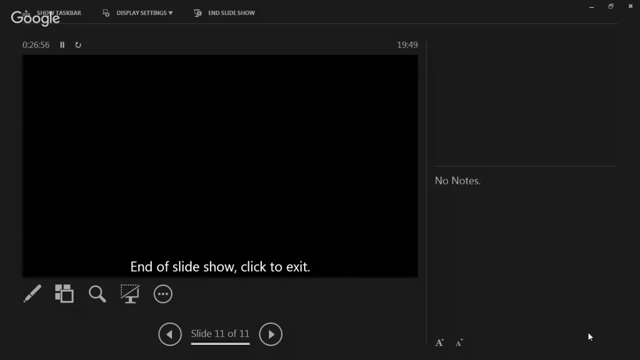 on the study on AQABA Um. the red sea is, by its location and nature, it's one of the warmest maybe sea. i mean one of the warmest in terms of temperatures- sea surface temperature- which is indicating that the ecosystem are already about their maybe upper limit to. 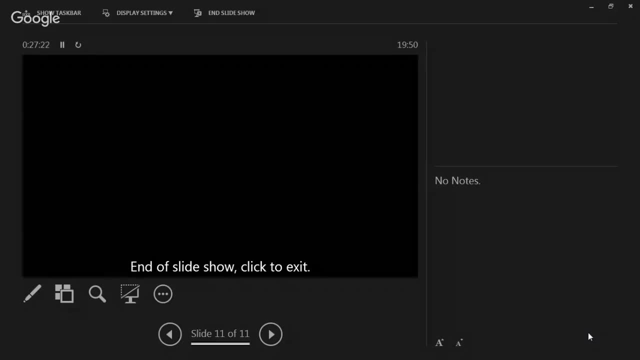 in terms of adaptation with these kind of increasing temperatures, especially now with the global warming? um, i just want to know whether this has been part of your studies and if you can share maybe more, some more insight about the results with the relation to sea surface temperature and the impacts on the ecosystem that are important for the livelihood of people. 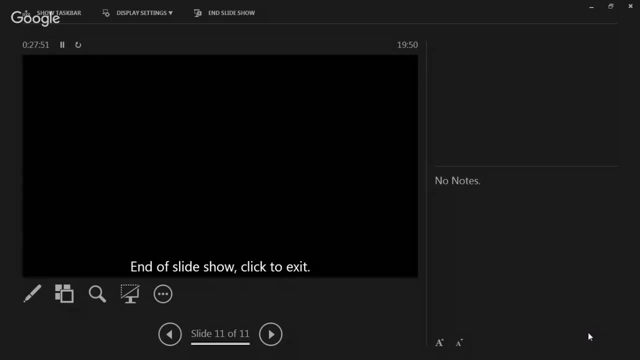 as part of this thing. thank you for the question. uh, actually, i disagree with you. the regarding the species of coral reefs, for example, species living in the red sea. this: the species living in the red sea, are characterized to live in such condition. the normal is the warm temperature is the normal for them. 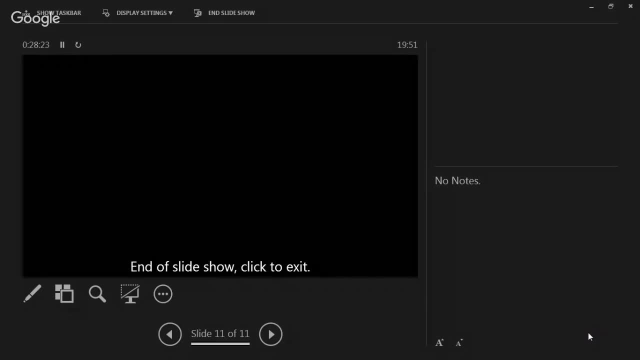 and if you increase the temperature more, this will be the problem. so so they are not in the higher limit, they are in the normal limit for this species, and this is the characteristics of the species living in the red sea in general. so this is the the point, but we of course considered that. 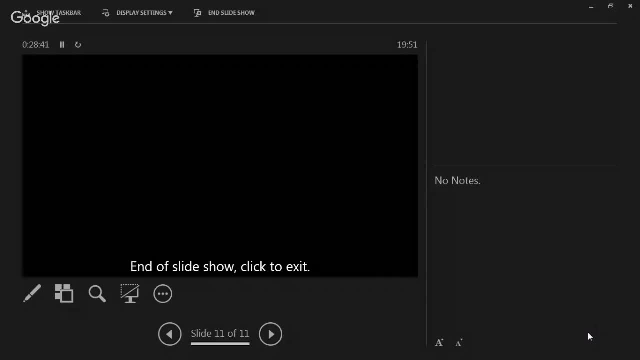 that we considered the increase in temperature in the sea and also the the changes in pH levels that is expected in the future, and I forgot to say that we used the regional model, not downscaling, and it we use the regional circulation models based on the chordics. 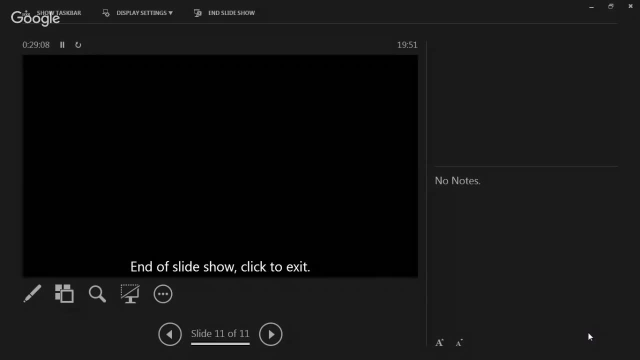 uh working group that with the domain of Africa, we used this set of information and set of models. so this includes all the, the, the parameters that you said, and we also considered the, the vulnerability of the system itself before climate change and after. so we made this distinction. 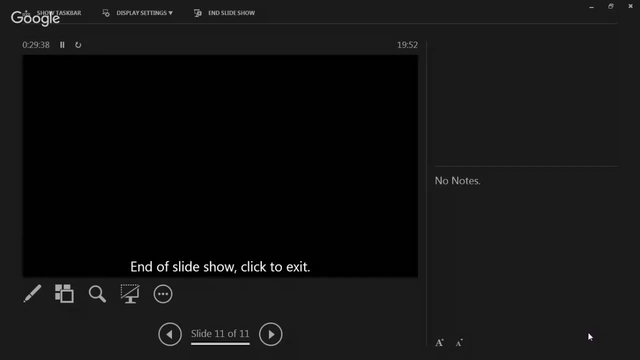 uh, and we could any. we included the, the human factor as well in the calculations. so if you are interested, you should look at the third communication report of Jordan for the UNFCCC so you can find all the details there. thank you about last question, please, hi um. 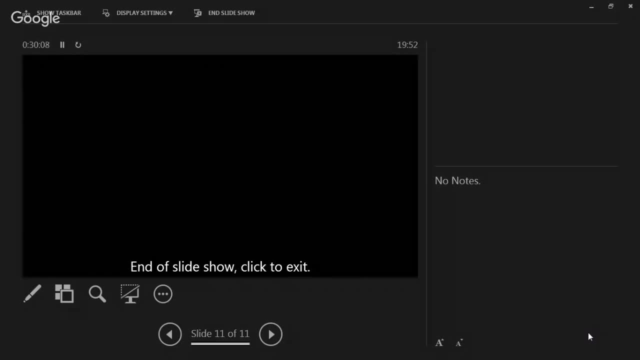 very late, catch your last presentation, so my question will be limited to you, but I'm lucky in your presentation with the final. you talked about coral revegetation or replanting corals. uh, replanting of corals, right, yeah, yeah, my question is: are you using the same corals?